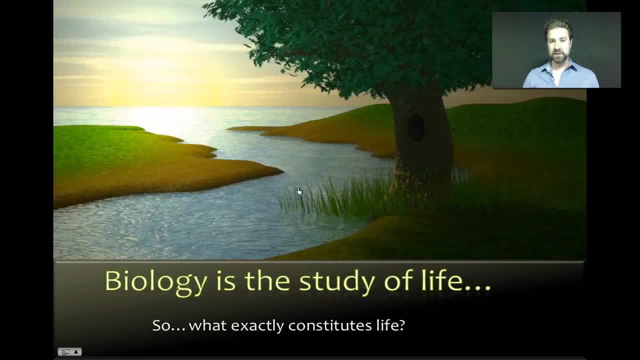 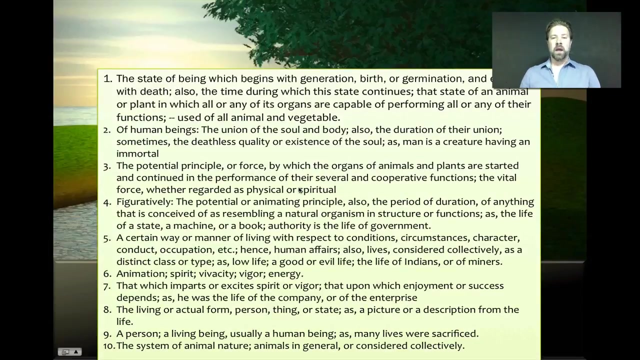 And those far outnumber the things that we see macroscopically, So there's a lot more little things than there are big things. All of those things, however, are alive, and biology is the study of living things, or the study of life. So what happens if we want to find a pure textbook definition of life? Well, I found one for you, and here is what it looks like when I looked it up. There's at least 10 different ways to think about life, So you would have to go through each one of them. 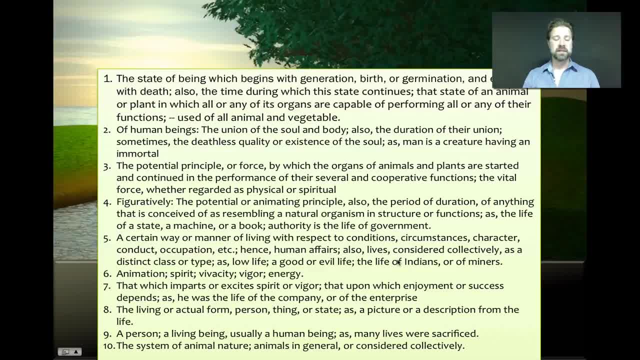 And you would have to figure which one sounds the best. Now, for our purposes, the first one is going to sound the best to us. So it says: the state of being which begins with generation, birth or germination, ends with death. Also, the time during which this state continues, That state of an animal or plant in which all or any of its organs are capable of performing all or any of their functions, used of all animal and vegetable. That's pretty heavy duty, And if you read through the 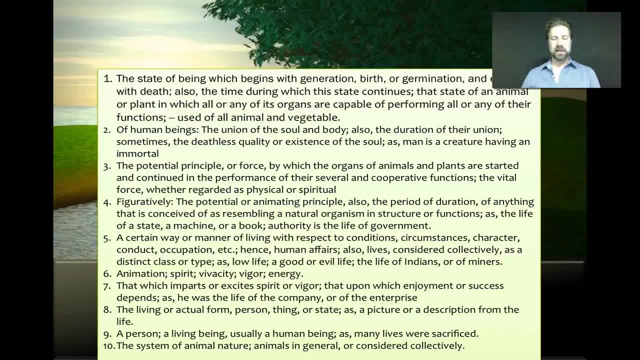 next nine, you're going to find that they are no easier to understand than the first one. Now, as good as the first one is, as much as it matches our purpose, there's some flaws in it, And one of the flaws that I see is the fact that it mentions particularly animal. 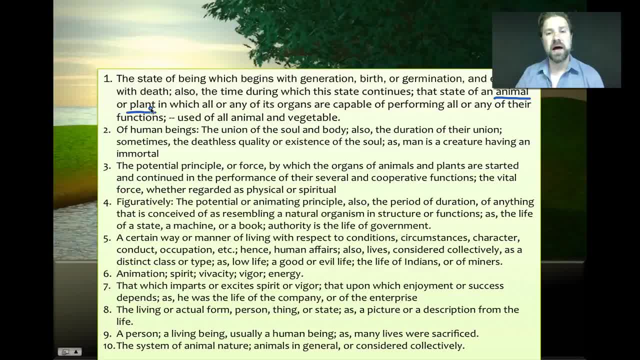 or plant. So what it's saying is: to be alive, something must be an animal or a plant, And if you look through your biology book, you're going to truly find that there are things in your biology book that are alive which would not be considered an animal or plant. 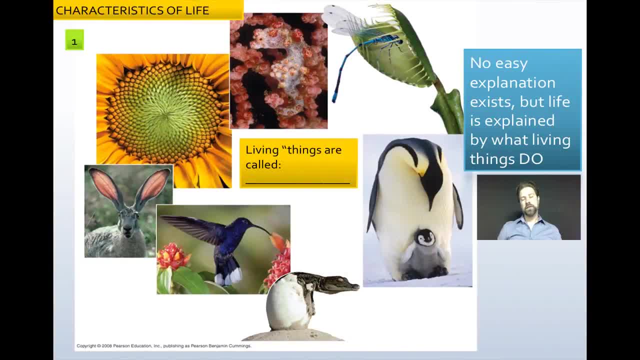 And we will delve into that this semester. So, then, there's no easy explanation of what exactly life is, But life is explained by what living things do. So here we see a wheel of pictures, all of which show living organisms, displaying the characteristics of life And 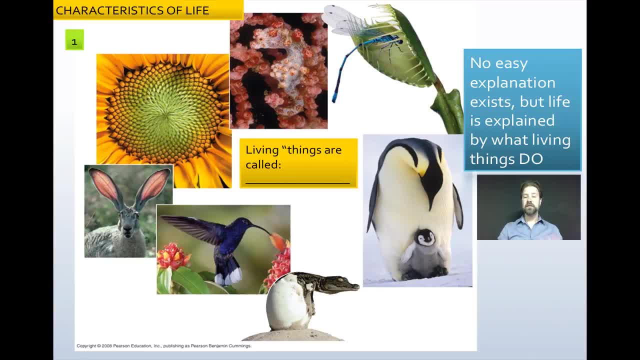 the first thing we can kind of knock out right off the bat here is that living things, when we refer to them as whole entities, we're going to call them organisms. Okay, No surprises. You've heard this word before and we'll be referring to it quite often during this class. 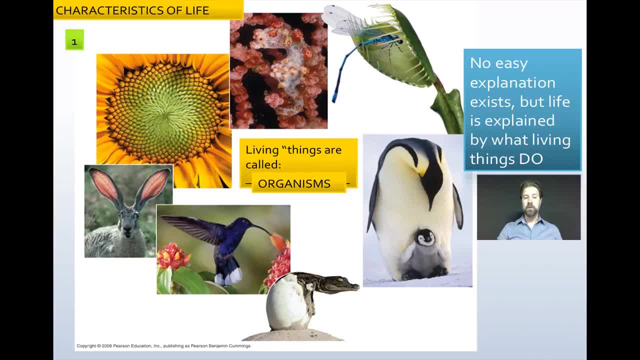 If we take a look at the first picture, the one marked number one, we can see that it's the center of a flower, And that flower is displaying order and organization. What that means is it's just not a random, chaotic mass of living material, but instead it's very organized. 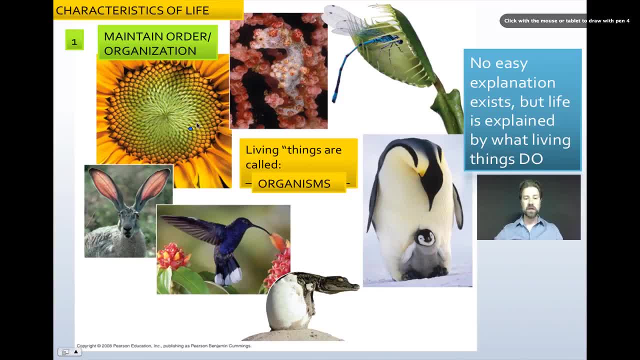 as you can see there. You can see that it has a central region here and you see that there are definitely lines of distinction That exist within the center most portion. So we have a round nature to the center. We have what we call radially symmetrical petals on the edges as well. that all seem to be coming. 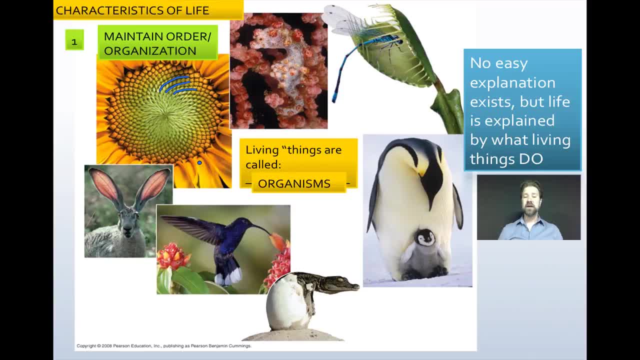 off of the central hub region. So this definitely is not a chaotic looking mass of organic chemicals that make up this living thing. They are organized very distinctly into unique structures. Now we could say the same for a human being. A human being is not a big bag of goo. on the inside There are definite structures. 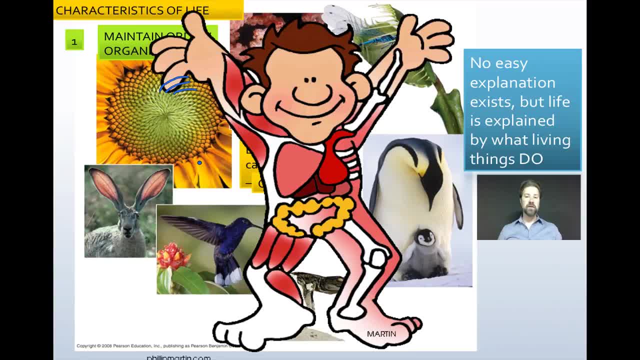 that have organization on the inside as well. Even when we are little children, we understand that there are hard parts inside of us called bones. Even though we don't know what the rest is or what it looks like on the inside, we know there are these hard structures called. 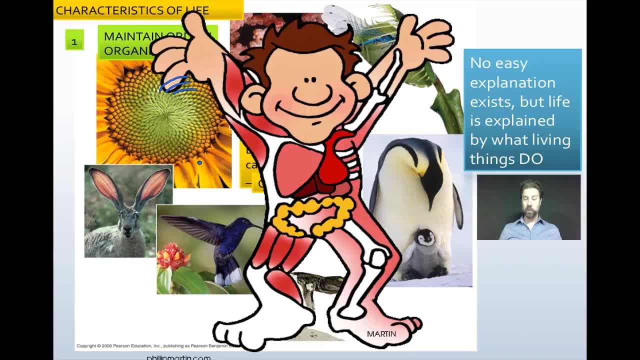 bones, and we try our best not to break them when we are little kids. So we must understand that there is a structure to living things- Exactly, Exactly, Exactly. That's right- And that these structures themselves are not chaotic either. They themselves have more organization inside of them than a lot of people know. 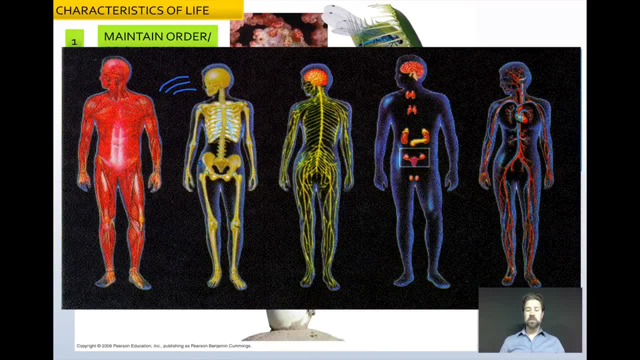 Let's take a look at some systems of the human body. So we see the muscular system on the left, We see the skeletal system, We see the nervous system in the middle, We see the endocrine system in the fourth picture And we have the circulatory system, or cardiovascular. 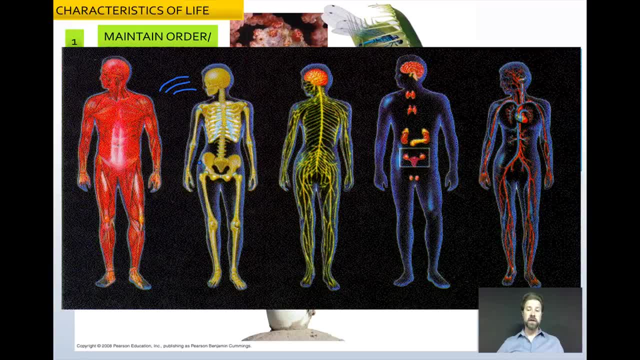 Well, yeah, just the circulatory system And cardiovascular. we'd have to see the lungs in there and we don't. So the circulatory system is going to contain the vessels in which pass the fluids of life around inside of a living human being, which, of course, is blood. 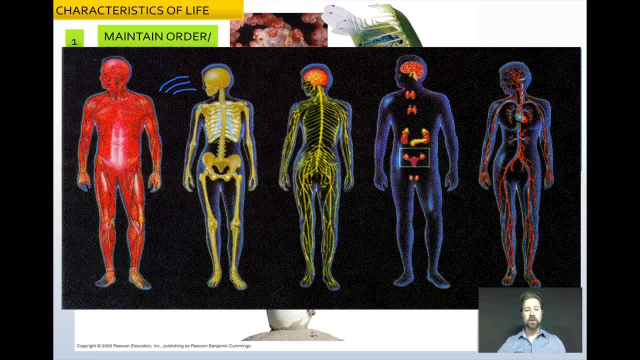 Now, if we take a closer look at the skeleton picture, we can see that the human skeleton is made up of a lot of bones- 206 of them- And those bones themselves. like I mentioned before, they have their own structure as well. 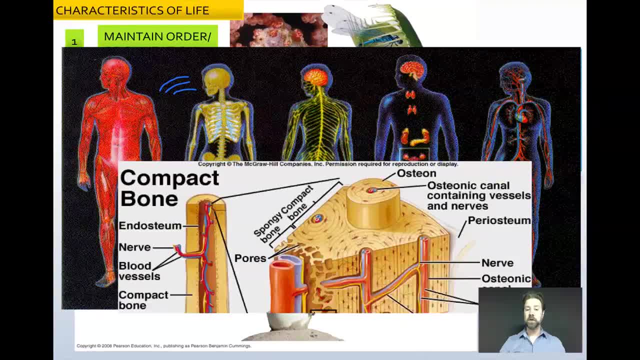 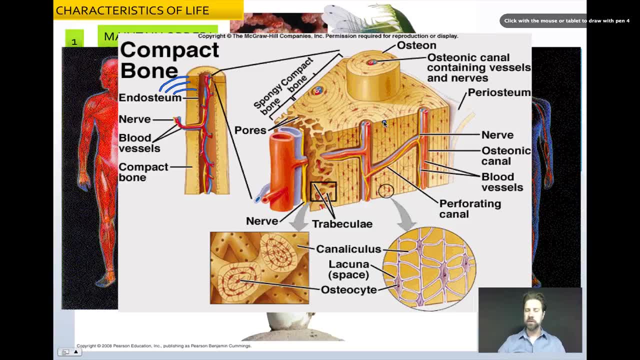 So if we took a look at the interior of a portion of bone, we might see something like this. So what we see here is a very organized structure. It has its own system of organization. This is called the Haversian system or the osteon. 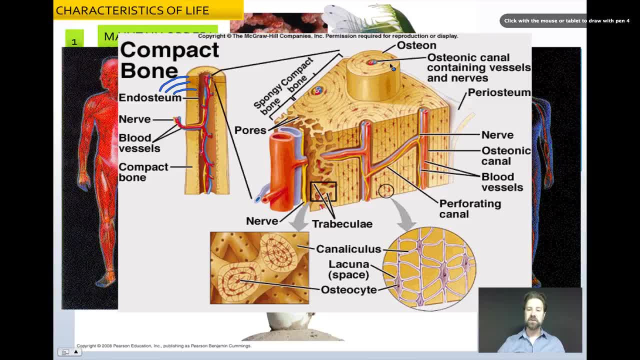 And you can see that you have little blood vessels inside of each one of these circular cylinders And you also see these concentric layers of rings on the outside. You see these little dotted structures on the inside. These are little cavities where cells exist. 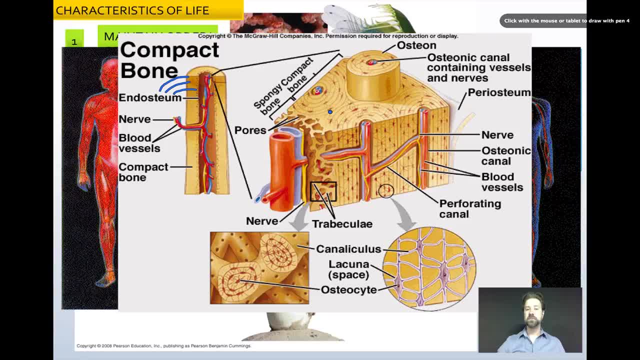 And what they do is they have these little cavities. They do is they can contribute to bone making or bone taking. So they'll either add or remove bone from a given region of bone at any particular moment in time, depending on what the body needs at that time. 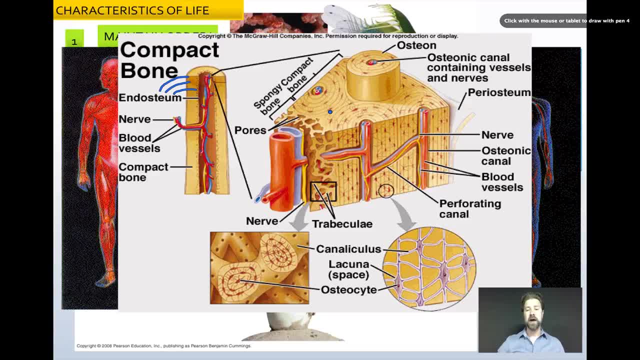 We'll talk a lot more about the skeletal system when we learn about the human body later in our class. So we never stop seeing patterns of organization within living things. Now we can even go as simple as a human cell, or really any eukaryotes cell. 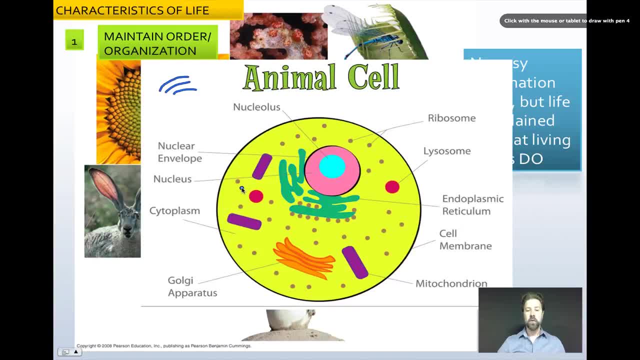 We can even go as simple as a human cell or really any eukaryotes cell. Now, we can even go as simple as a human cell or really any eukaryotes cell cell, and this is what we're going to find on the inside. We're going to see what looks like it. 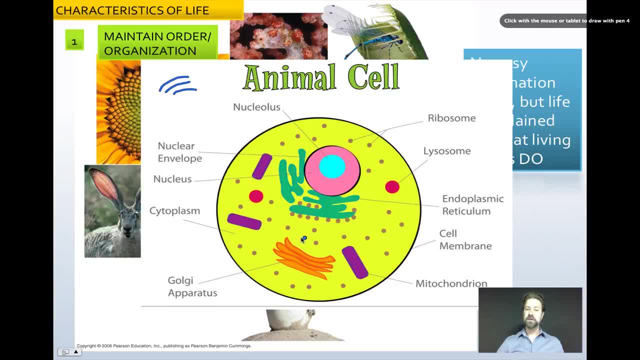 could be chaos, but the fact remains that in every single one of these animal cells, we see the same structures over and over and over. The three things that are always going to be present is the cell membrane, which you can see right here. We see the cytoplasmic region right here, which 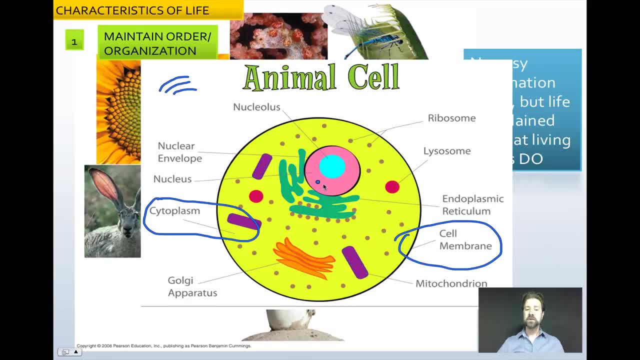 contains this soup full of organelles, and we see a nucleus here that has a nuclear envelope around it. So those key structures are always going to be present in animal cells. Now, things that are also present in animal cells are going to be organelles, and this is where you probably remember. 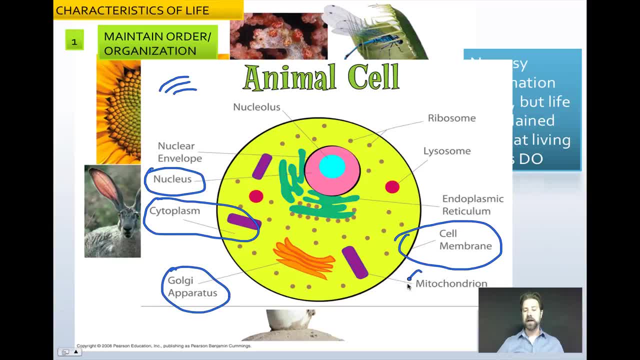 some of these names from your last class, like the Golgi apparatus, mitochondria, lysosomes, endoplasmic reticulum, also called ER, little protein building factories called ribosomes, and even a dark central spot in the nucleus called the nucleolus- All of these things are present. 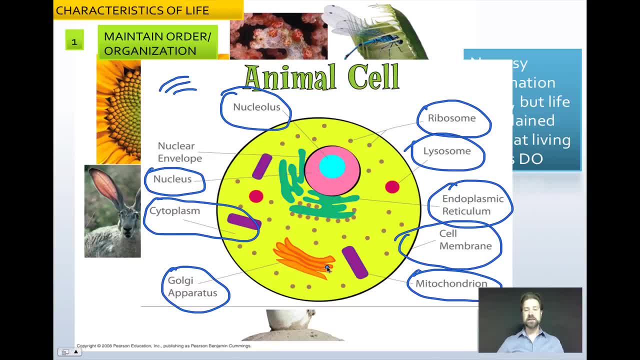 in the nucleus. So we're going to see what we're going to find in the nucleus In every animal cell. So this is a system of organization. It's a little bit more loosely organized than other structures, but we see the same pattern over and over and over, which means 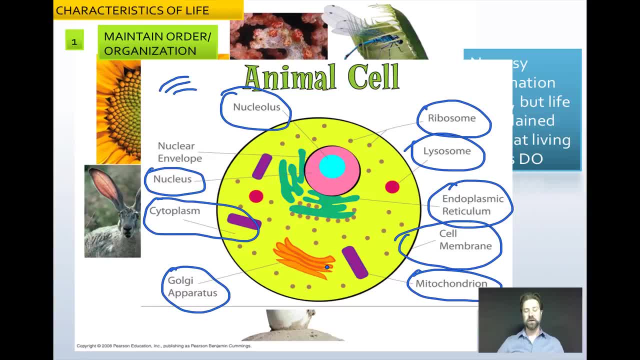 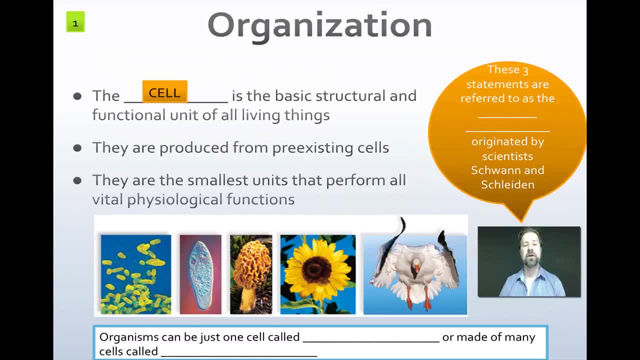 that it is a structure of organization. It is a unit of organization within living things. So the cell is, then, the basic structural and functional unit of all living things. So if you look into anything that we consider alive, you'll find one or more than one. 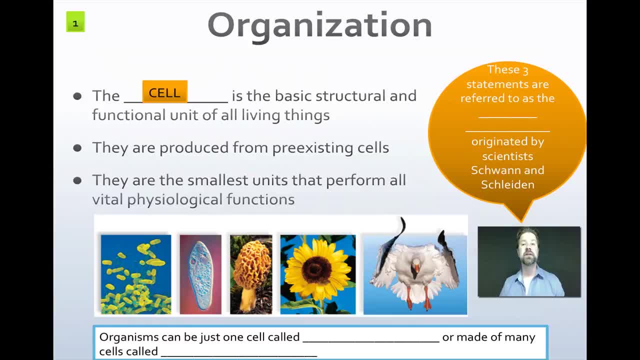 cell present and you will see sometimes hundreds, sometimes thousands, sometimes millions and sometimes trillions of cells that work together to form possibly a tissue, possibly an organ, an organ system or even an organism. Now, they are all produced from pre-existing cells. What does that mean? Well, it means that a cell cannot just spontaneously create itself out of nothing. 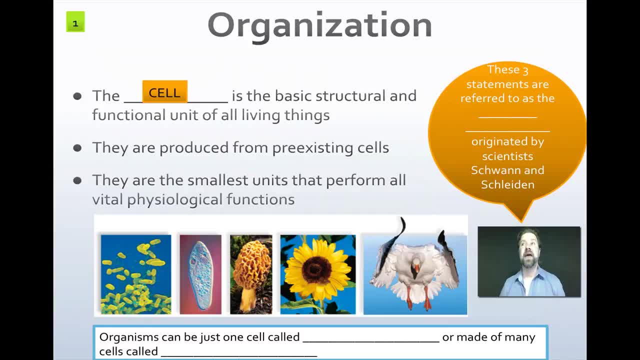 Hundreds of years ago people believed that things like maggots and little worms could come out of nothing and just spontaneously appear on things like grain and dead organisms. They also thought that mice could appear in grain stocks out of nothing. So they did all kinds of tests and research and they were able to come to the 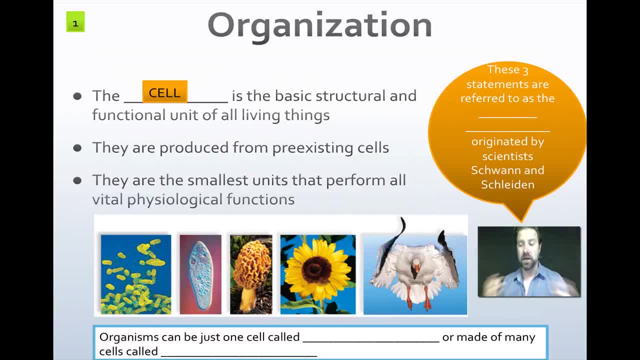 conclusion that they were wrong, That it wasn't just coming out of nowhere, but instead each of those things, from a maggot to a worm, to a mouse, they all had cellular origins. So there was an experiment that really helped this idea along. It was done by Louis. 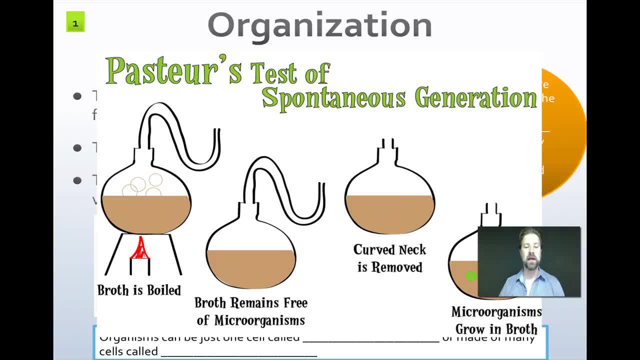 Pasteur, and we're going to find out more about this experiment later. but using a special type of biological apparatus, he was able to prove that you cannot just spontaneously generate cells. Instead, it's going to require another cell to go ahead and divide to give you your next set of cells. 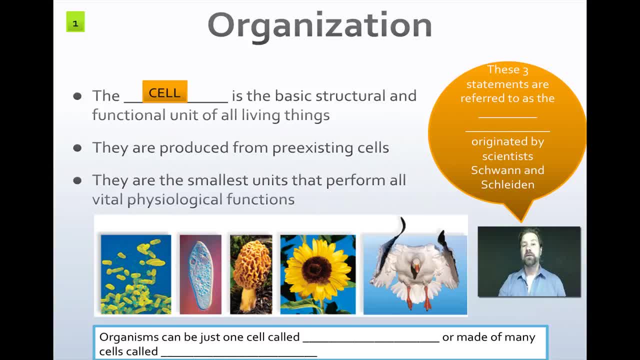 Cells are also the smallest units that perform all the vital physiological functions. So from our last slide you saw a whole wheel of pictures and a cell can do all of those things because it can perform all the vital physiological functions or characteristics of life. Now these three statements are actually very special because they are considered cell theory. 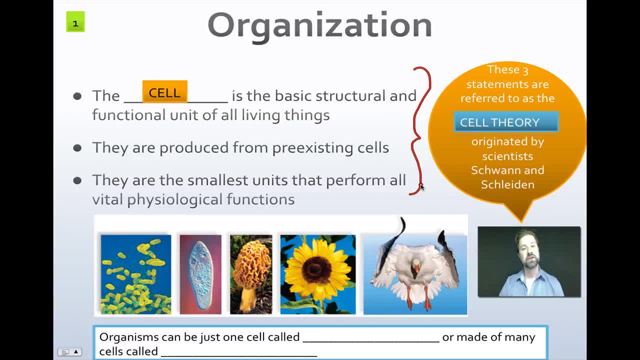 Cell theory was originated by the scientists Schwann and Schleiden, And they are a big key part to the understanding of basic biology. If we look down below, we mentioned these earlier that these are bacteria, and we know that every bacterium must come from another. You can't have these just come out of nowhere, So it's possible. 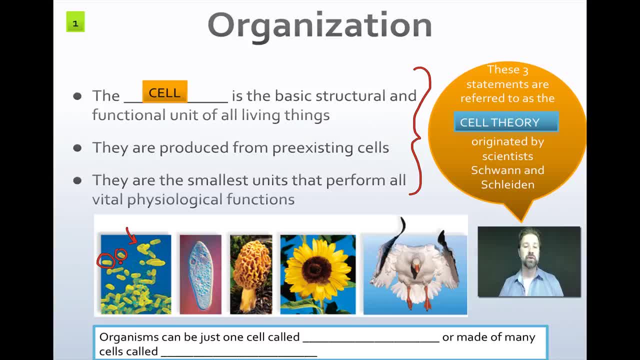 that this one here came from that one there. It grew to a certain size. Once it hit that size, it's split in two by a process of binary fission. To the right of that we have a cell called the cell of the human body. 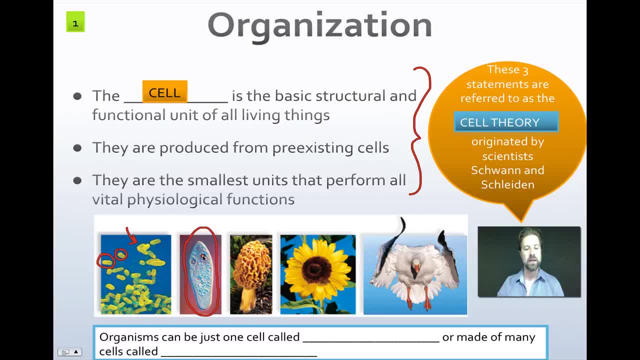 And to the left of that we have a simple one celled organism. here. This is a Paramecium. We have a fungus. here We have a flower part of the plant kingdom here And here we have an animal. Organism can just be one cell. So in this case, this one here and this one here represent living things. 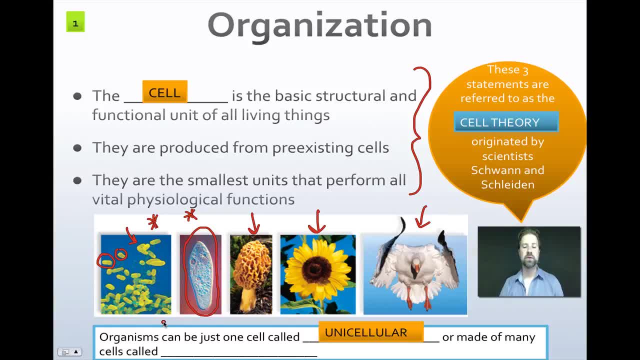 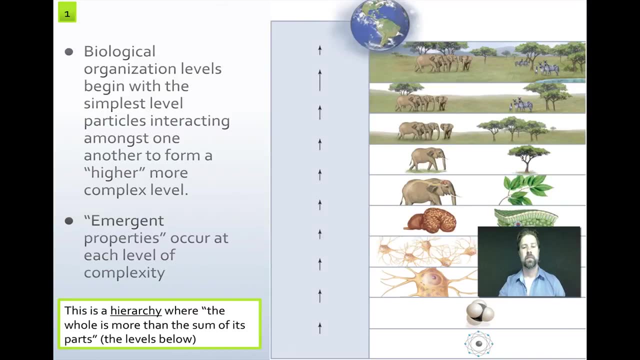 that are just one cell big. Those are called unicellular organisms. Or it can be made of many cells, is the case of the fungi, the plant and the animal, and that's what we've called a multicellular organism. We are a multicellular organism as well If we look at the levels of organization. 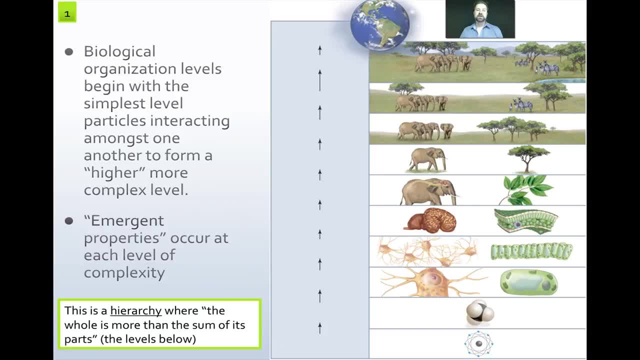 we can start at a very small level and we can start to see properties emerge as we go up every level. For example, at the bottom level on the right here I see an atom. If you guys remember back to high school, you have atoms and these atoms when they find the right partners. 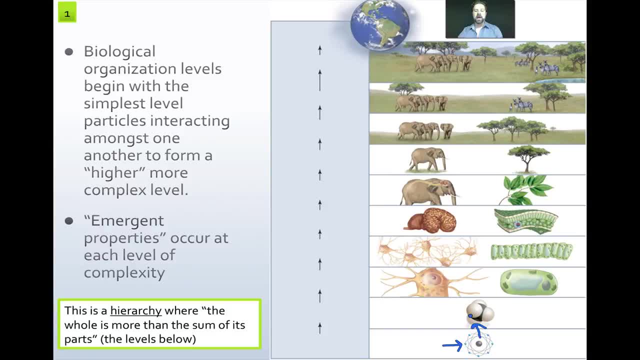 they can change into molecules and molecules do different things chemically than atoms do. Now if I happen to put together a few million of the correct molecules, I may be able to form a cell, either an animal cell or a plant cell, and going from these millions of, 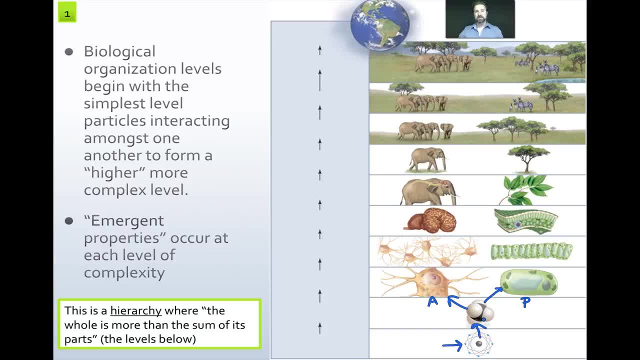 molecules to a cell. I'm going to be able to form a cell and going from these millions of molecules to a cell. I'm going to be able to form a cell and going from these millions of molecules that do not exhibit any of the properties of life, If I have the right ones. 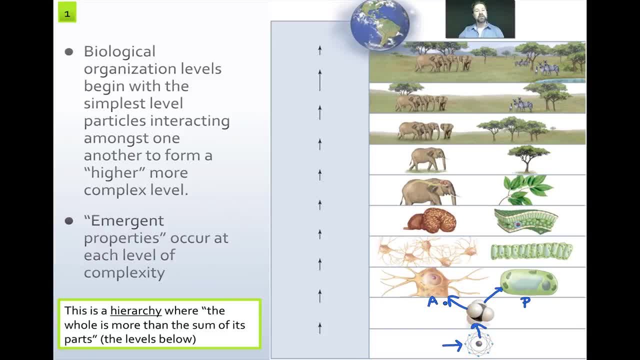 there. I can form a life form here and the simplest organism that can exhibit those properties of life that it couldn't as a molecule. If I put enough of these cells together of the same type, I may be able to form tissues. So this here would be an example of nervous tissue. The way 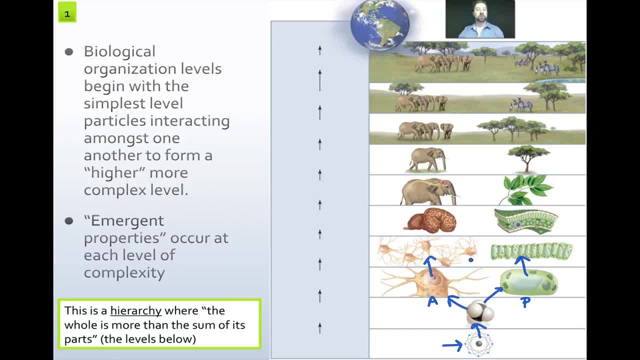 that these cells are shaped, tell me that this comes from the nervous system. So if I put together this 진 오늘은의 이걸게 Khisteriyin, this particular plant cell here will become part of a leaf, And those little dark green things that you see in there are chloroplasts that allow it to photosynthesize. 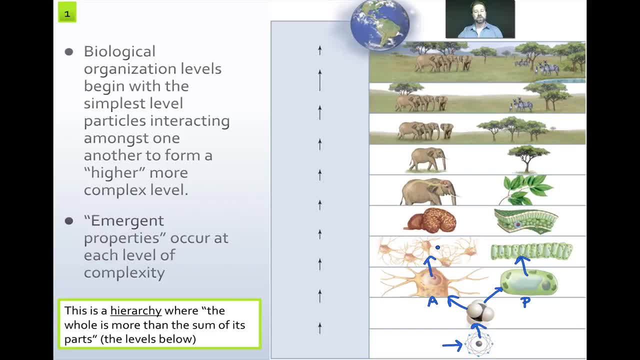 As we climb up the particular type of tissue and we put enough tissue together, we might form organs. So in this case we see the brain. You can take a look up here. It is going to be the brain of an elephant. 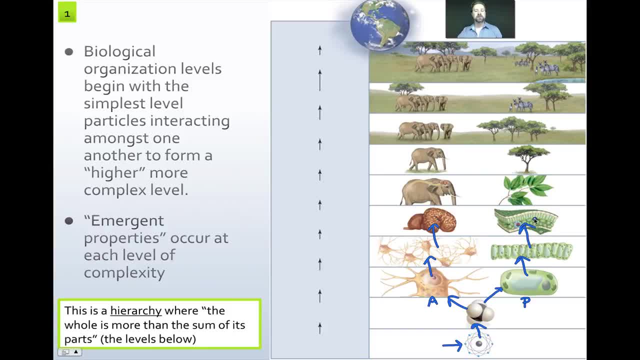 And again, this is a bigger cross sectional piece of the brain. And again this is a bigger cross sectional piece of the brain: the leaf. and if we put organs together we build a bunch of organs that are connected together. we can have an organ system such as the nervous system in. 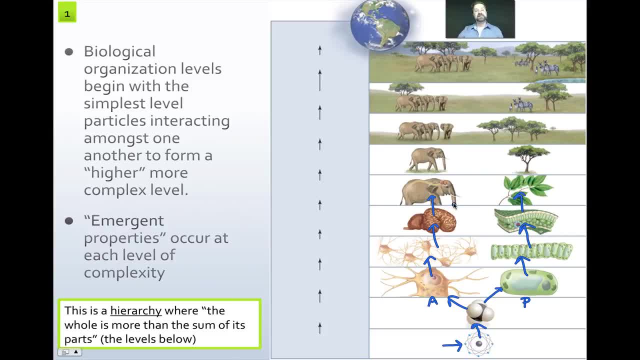 this elephant. once enough systems are put together, you may be able to have an entire organism, a multicellular organism, which has a lot more properties than just a organ system or an organ, because we know that these don't do too well on their own without those other systems being present. so each time we move up a 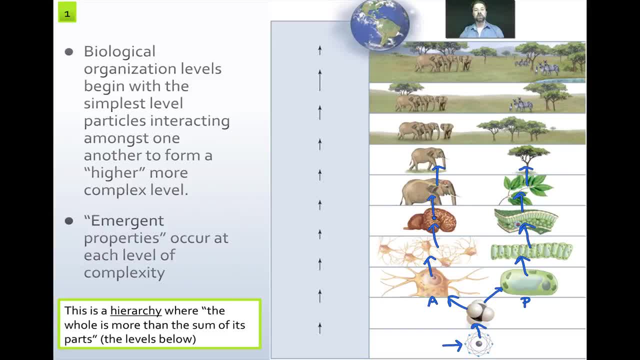 rung on this ladder, we start to see new emergent properties come out. let me catch up with some of the labels for each one. I forgot to pop these up. we have the atomic level, the molecular level, the cellular level, tissue level, organ level, organ system level and then, finally, the organism level. 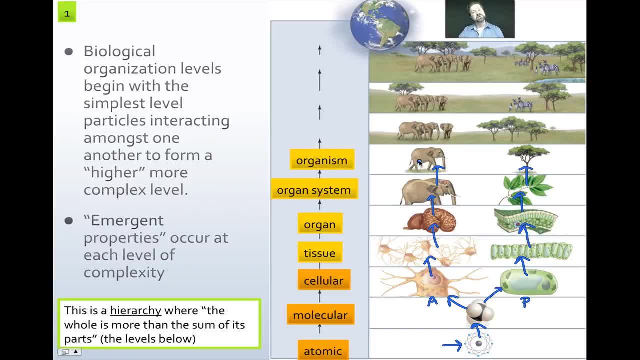 now you can see that the pictures go further, because once you put a number of the same species together, you then go from a single solitary organism to a population of organisms, and once you put a number of populations together of different species. so here we see zebra, here we see those trees, here we see 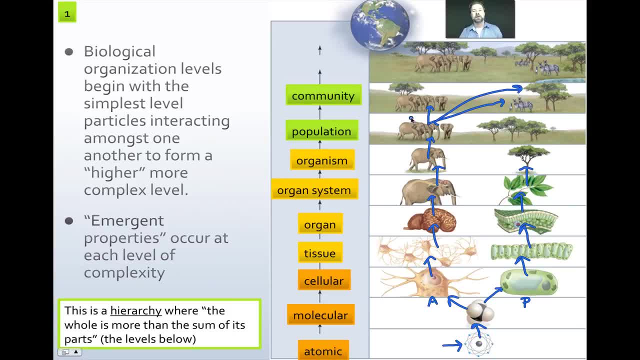 elephants. we then have what's called a community community that lives and interacts together, and those interacting communities can form an ecosystem with the rest of the environmental things that are around it. so this would be a much larger area here to qualify as an ecosystem. so we take into consideration some of the abiotic factors that exist. 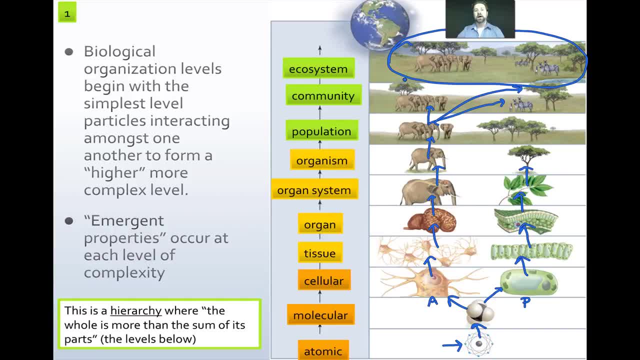 here as well, such as water, such as the wind, such as the amount of Sun and the soil, the rocks that are present, and then, finally, all the living things on the planet, are going to interact in the biosphere. so we can't separate- truly separate- one ecosystem from another on a 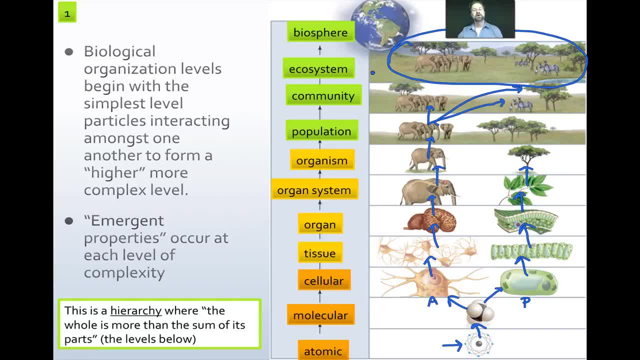 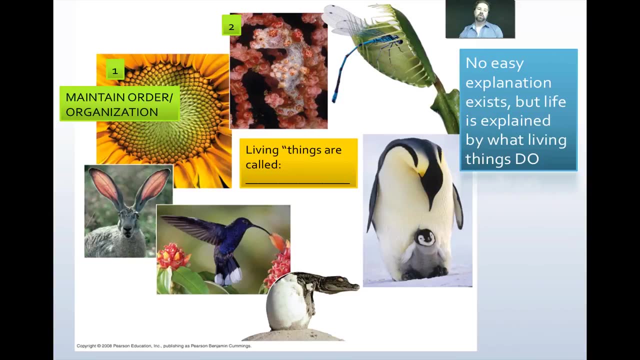 line on a map with a line, it's just too difficult. there's a lot of blending that goes on and all the things that are alive share this, this planet earth, and make up the biosphere. Okay, so we've touched upon organization. we know living things maintain order and they're. 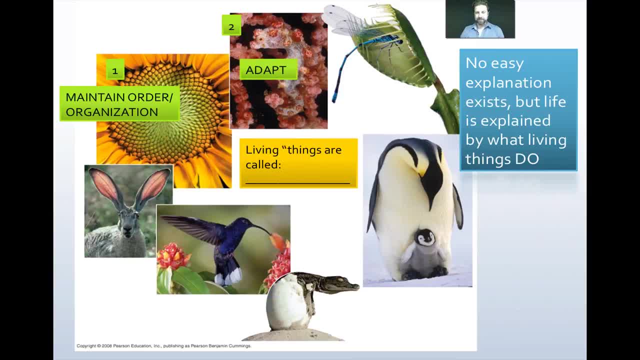 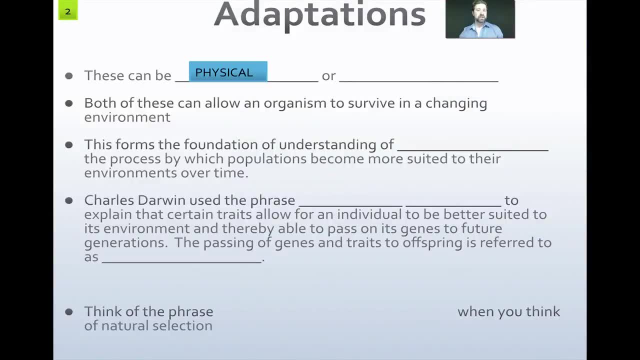 organized. Two living things adapt. Now adapting may mean that something is physically changing or possibly behaviorally changing. Now what would be the best example? The best thing we could do is take a look at an animal and talk about what physical and behavioral adaptations it may have. 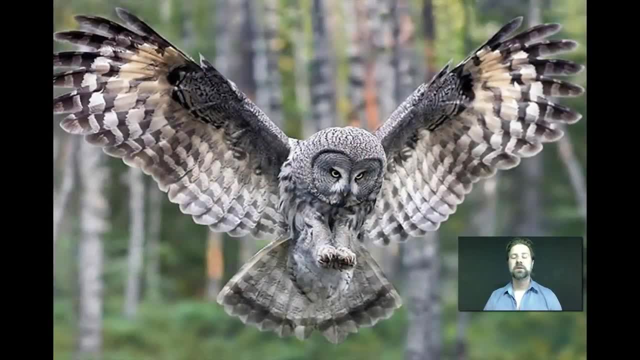 So here we have an owl, and the owl has a number of physical adaptations that's going to help it survive. All of these adaptations are going to make an organism better suited to its environment to survive and pass on its genes to the next generation. 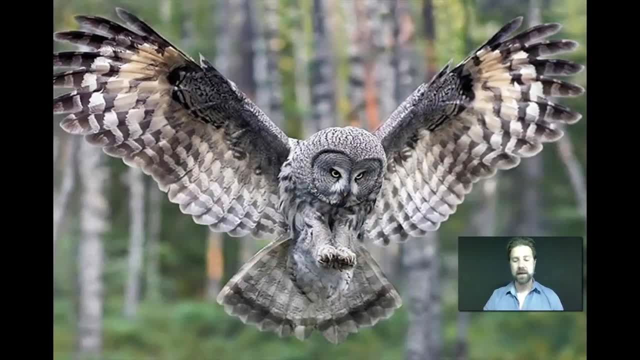 So the first thing that we could say is that it has talons. We can all see that. it has these claws come out of its feet here, and these are very strong claws. In fact, they kill most animals, They kill most of their prey with those claws alone, and the owls are said to have some. 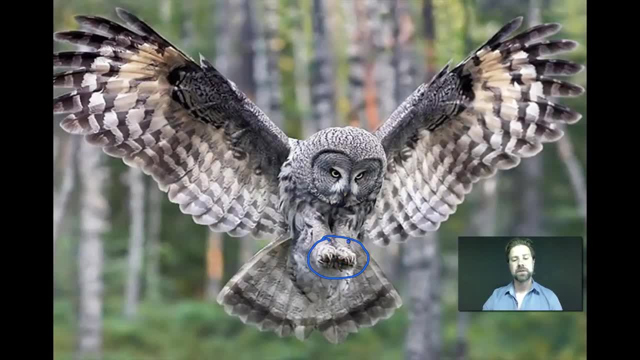 of the strongest gripping strength of any of the raptors, of any of the birds of prey. It's kind of hard to tell, but owls usually have very large eyes in proportion to the rest of their body as well, which give them great vision, and especially nocturnal vision. because they wind up doing most of their hunting at night. So inside the eyes we have two types of cells called rods and cones, And rods are super sensitive to light, and so an owl's eyes have a lot more rods relative to, say, a human's, because we do most of our things diurnally throughout the day. 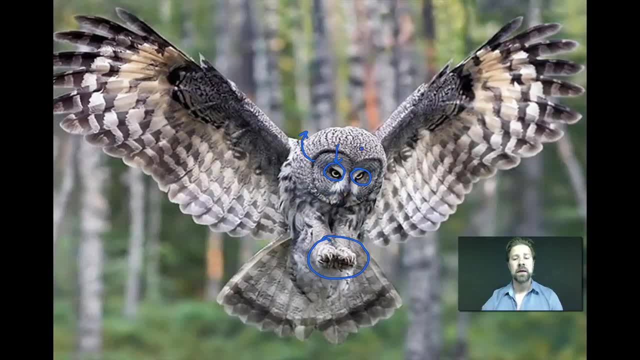 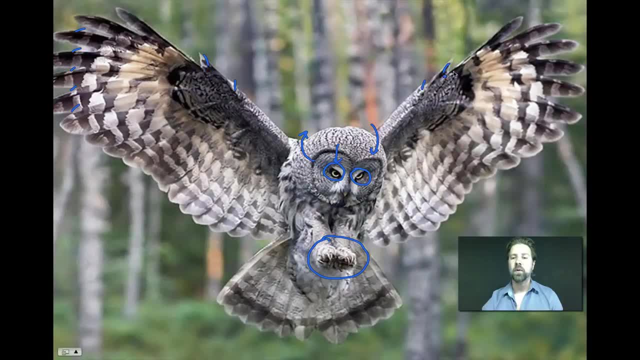 So these feathers that are found on the wings when an owl flaps them. you don't hear the owl, So it very stealthily goes after its prey. Consider that with a regular bird that flaps its wings and you can hear it coming from. 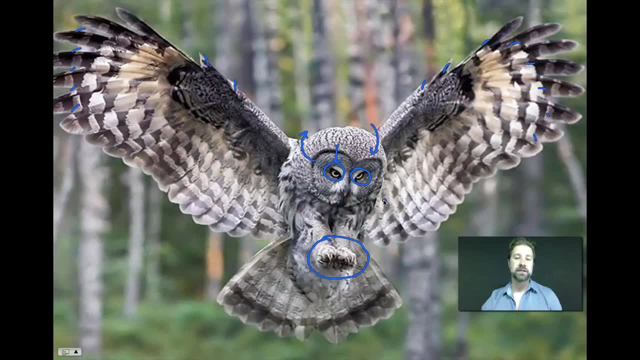 feet away. So an owl's an ambush hunter. So those are all physical adaptations. What about behavioral? What does this owl do behaviorally that allows it to survive better? One of the things that it does: it only hunts during the night. 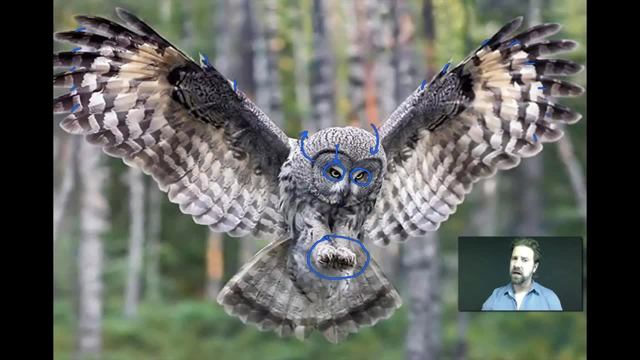 Why would that matter? Well, if you think about the other things that hunt during the day, that are raptors or birds of prey, we have things like bald eagles, we have things like hawks. Maybe to decrease the competition amongst these birds, it chooses nighttime because 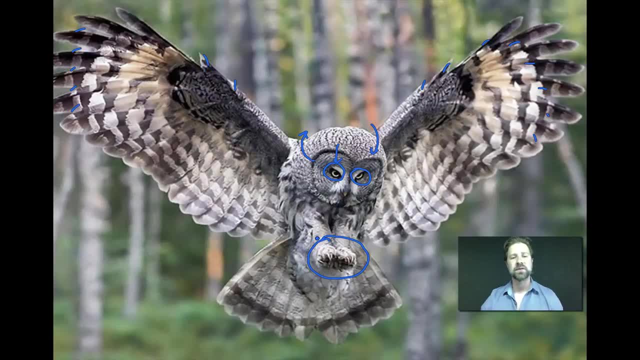 its body is better suited to that, And that had to take place over thousands upon thousands of years to have the two of them work harmoniously like that. But it was a winning strategy, because we know that there are owls present at night and 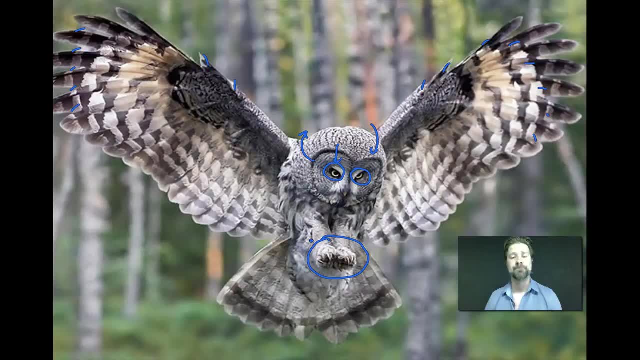 we know that there's hawks, There's owls and eagles that are present hunting throughout the day. Another thing that these owls will do is they will perch very high on posts and they will watch and they're very keen on sensing moving things out in the field that they're watching. 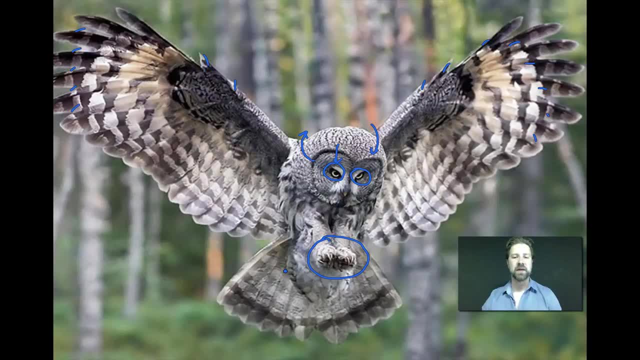 Once they sense something is moved, they'll go ahead and they'll do a particular type of flight pattern where they kind of just soar quietly back and forth over a field looking for that disturbance that they saw. Behavioral adaptation will allow them to be more efficient hunters as well. 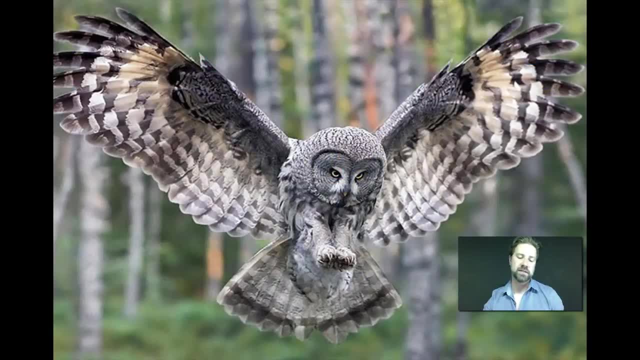 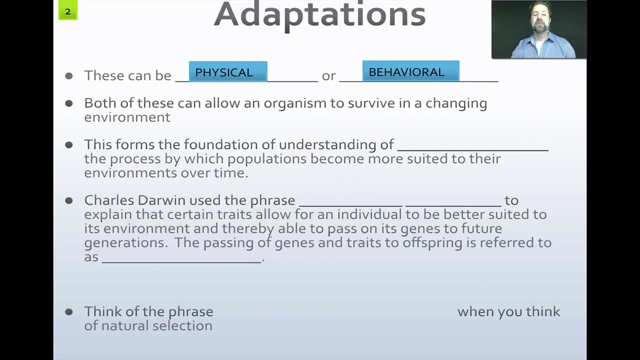 So, physically and behaviorally, the owl makes a great study for adaptations. This forms the foundation of the understanding of evolution, the process by which populations become more suited to their environments over time. So as environments change, animals also change as well Populations. 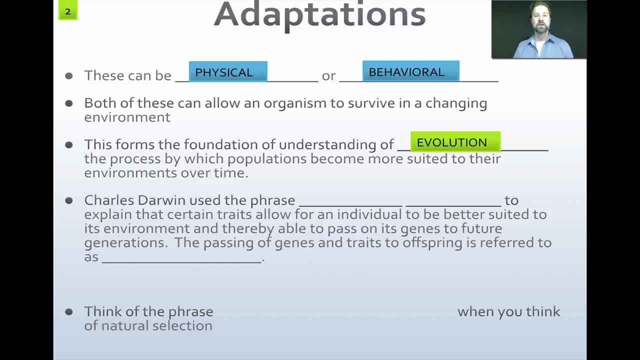 They take on new traits that may or may not work towards its benefit. Charles Darwin used the phrase natural selection to explain that certain traits allow for an individual to be better suited to its environment and thereby able to pass on its genes to future generations. The passing of genes and traits to offspring is referred to as heredity. 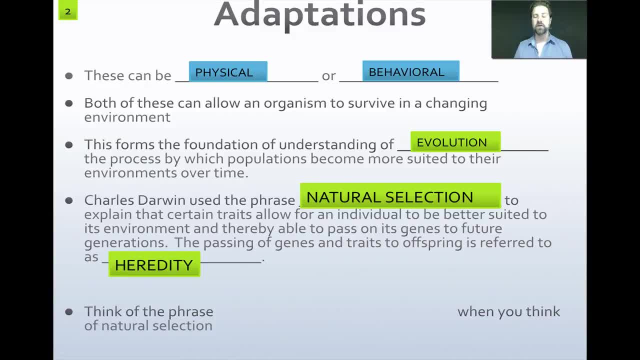 So the best suited individuals to a particular environment are going to survive and live on to reproduce. They will then generate that next generation and it will continue to do so until it doesn't have the necessary adaptations to survive. If something doesn't have an adaptation, the chances for it reaching reproductive age are 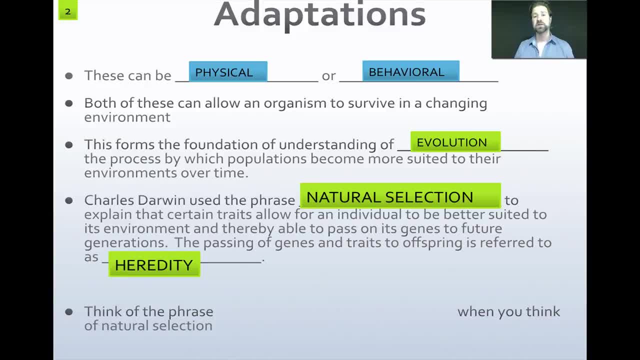 much lower, and successfully producing offspring is much lower than it would be if it had the adaptation. So try to think of the phrase differential reproductive success. Some things successfully reproduce very well, Some things don't- Some animals and some do not. The ones that do will continue their genetic line to the next generation. 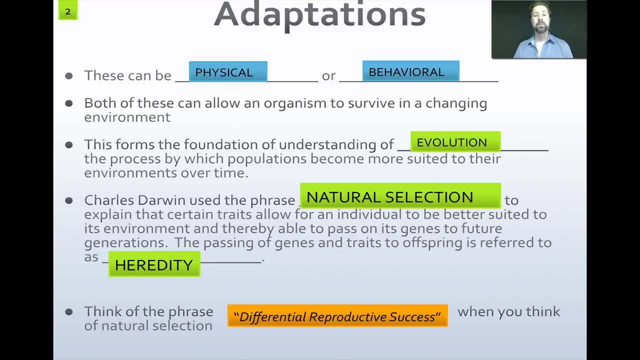 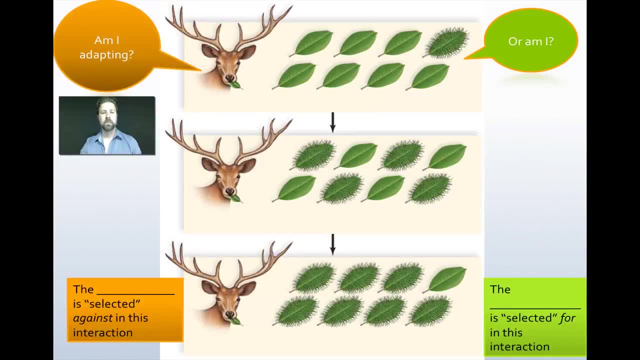 The ones that have very low reproductive success will probably wean out over time and will go extinct. Here we have a scenario of a deer whose favorite food is a particular type of shrub that has leaves that look like these. Now we're going to make believe that some mutations 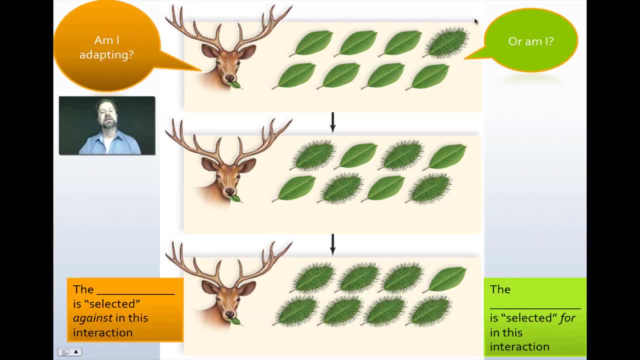 And it caused the leaves to come out with this kind of spiky, unpalatable surface that the deer just does not like to eat, because it hurts its tongue when it bites into one of these leaves. So what's going to happen here is the deer is going to continue to eat its normal meal. 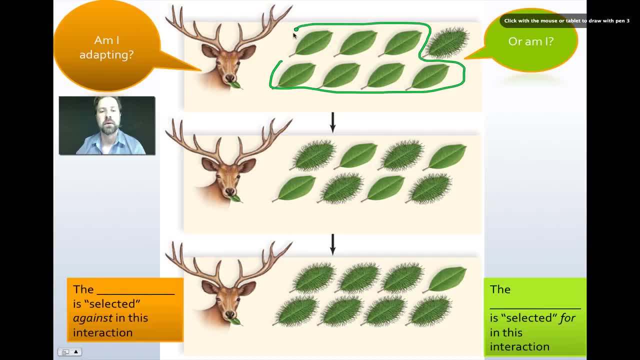 which is this non-spiky type of leaf here, And it's going to try to dodge this one. It doesn't want to eat this one very much, So upon eating these leaves, it's also going to eat some of the reproductive structures. 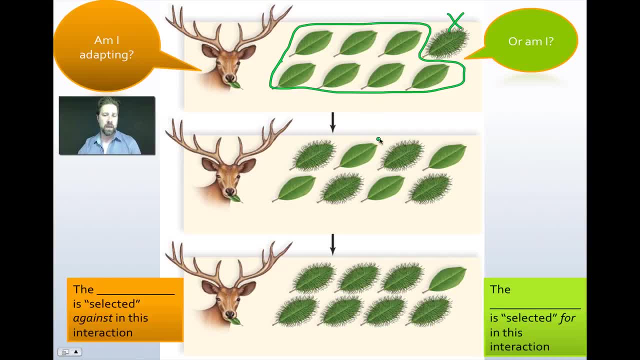 that wind up budding off of the particular shrub And in doing so it gives the shrub less of a chance to plant seeds in other locations for more of this plant to come out. So by the deer eating what it normally does, it's decreasing the fecundity of this particular. 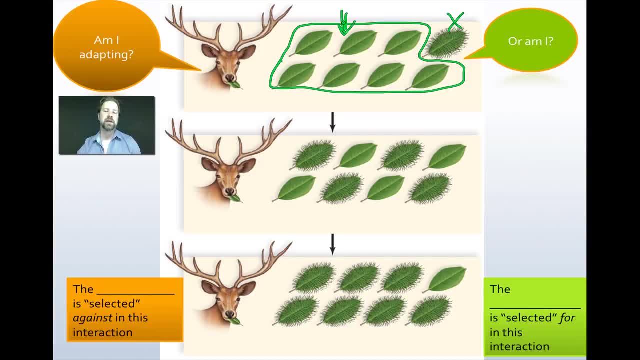 type of shrub. So it's going to eat these leaves, It's going to eat the shrub, So its ability to reproduce successfully. So what that means is if it's avoiding this particular spiky leaf, the spiky leaf has 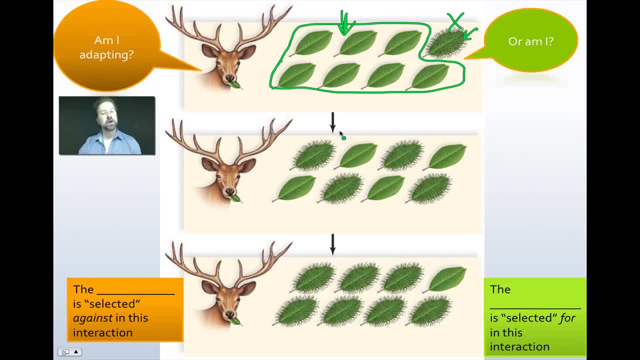 no problem reproducing in other areas. So you're going to start to see more and more spiky leaf plants, And meanwhile the number of deer hasn't caught up to the fact that it's losing its food source, because now we only have half of the regular shaped leaves available for this particular 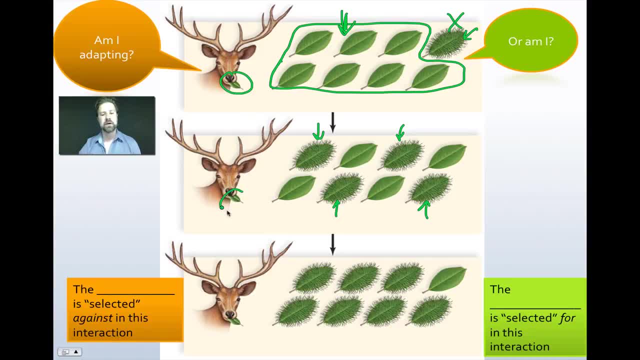 deer And, as we can see, he hasn't changed his eating habits at all. It's still the smooth-edged leaf versus the spiky one, And as the number of deer increase and the smooth leaf becomes a limiting resource, a couple things are going to have to happen. 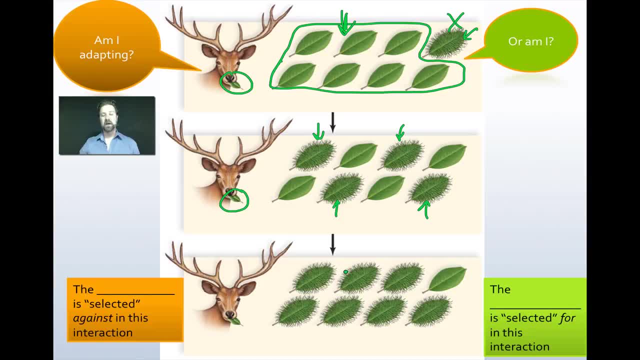 Either the deer is going to have to change what he normally eats- adapt behaviorally- or the other option is die, Because if it can't eat this particular type of food that it's currently eating, it may not have enough nutrition in order to maintain enough calories to survive. 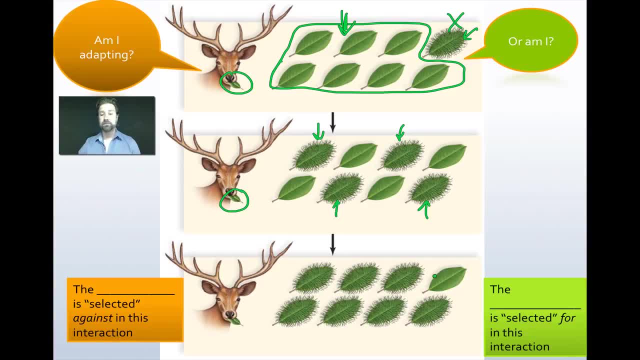 So here we see- almost you know we're talking- 80 to 90% of its original food source is gone. It hasn't yet developed the ability to withstand eating this spiky one. So the question is: will this deer adapt or die? 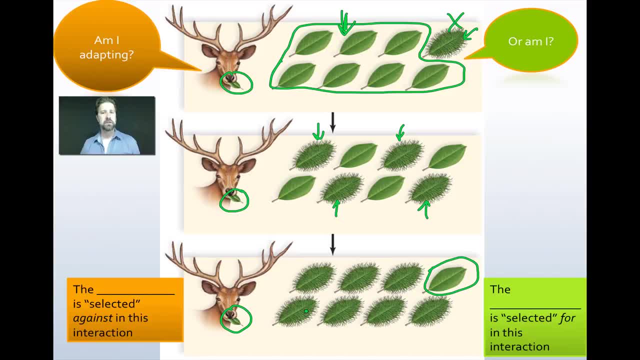 Now, when we talk about Darwin's view on natural selection, we say that some species are selected for And some species are selected for And some species are selected against. Now the question is, who is selected for here and who is selected against? 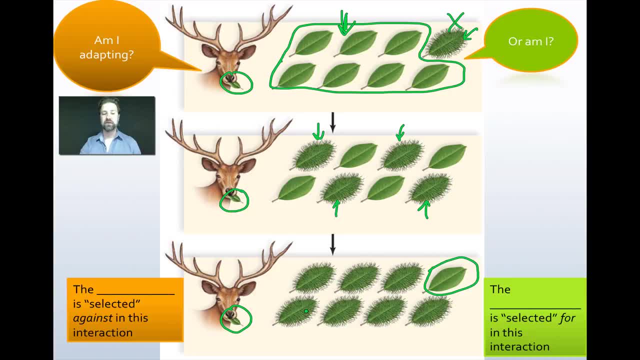 Well as we can see, the deer, by not changing its food source, means that it is going to be selected against in this interaction. The prickly leaf subspecies that came from mutation is selected for in this interaction If the deer move on and, over time, give this particular plant a chance to grow back and 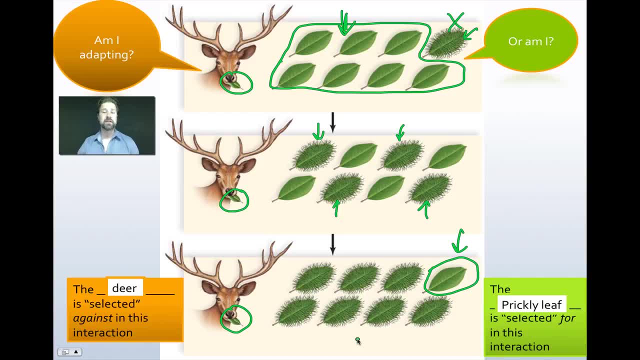 to repopulate. That may happen and the deer might be fine if they find a new foraging ground. However, if it doesn't, and this stays as its only food possibility, it may die if that food source runs out. So in the case of who's adapting here, the shrub actually adapted by way of a mechanism. 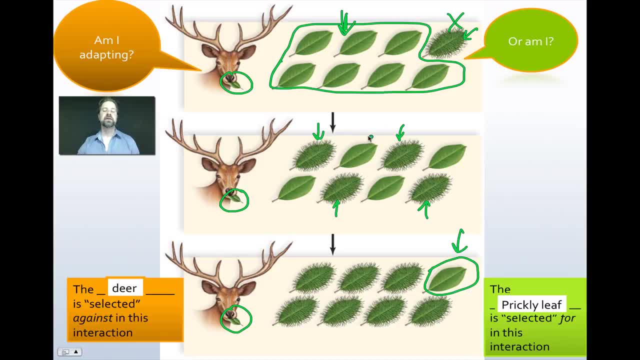 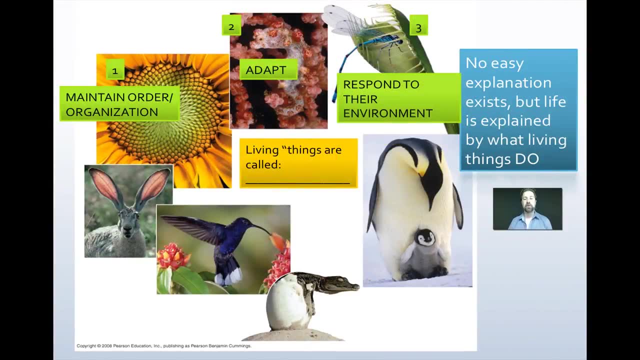 of a mutation, So it worked out positively this time for the shrub. The third characteristic of life we're going to look at is that organisms respond to their environments, And in this situation here we see that a damselfly has been attracted to a venus flytrap. 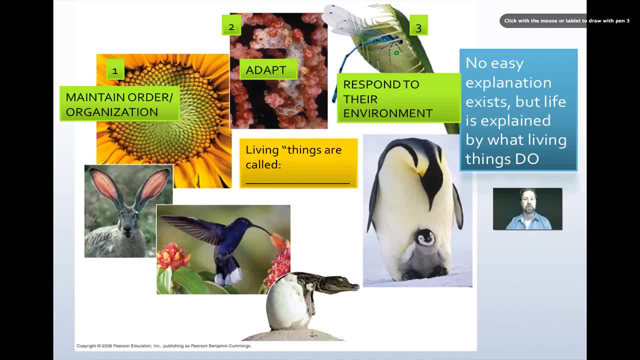 Possibly the coloration of the venus flytrap. the chemicals that are present drew this damselfly in for a possible meal And the damselfly happened to trigger a couple of trigger hairs that are present on the venus flytrap here and here. 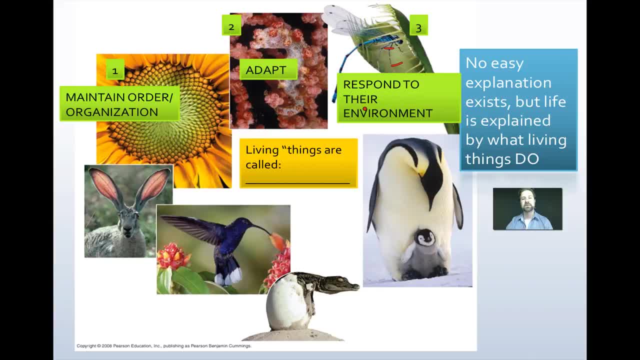 It struck them with its feet and striking those two trigger hairs at a certain tempo allowed the venus flytrap to use that as a stimulus to close its jaws on this damselfly. And now the venus flytrap has responded to its environment and now it has a meal. So it grew this structure because it has to obtain its nitrogen not through the soil, because the soil that a venus flytrap lives in is very poor. So it grew this structure because it has to obtain its nitrogen not through the soil, because the soil that a venus flytrap lives in is very poor. 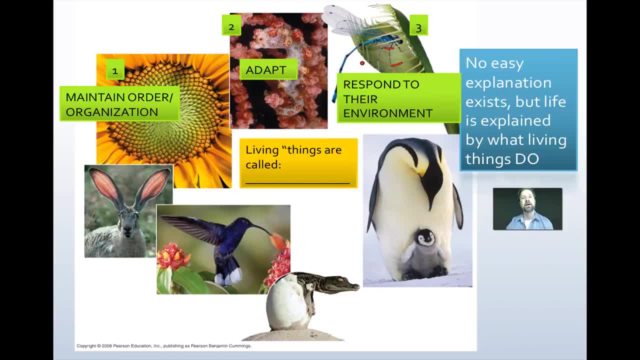 So it grew this structure because it has to obtain its nitrogen not through the soil, because the soil that a venus flytrap lives in is very poor, So it obtains its nitrogen through eating live animals, in this case a damselfly 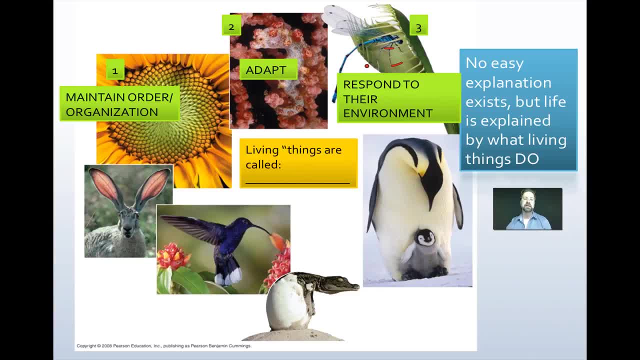 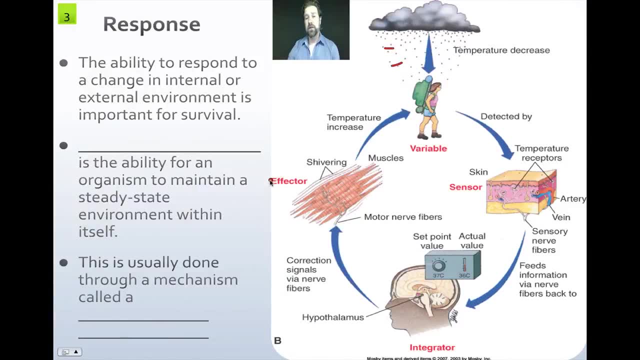 So each one responded to its environment, and it did so in order to successfully survive that particular environment. Now, responding to the environment is a very, very important thing, and we do so as well. For example, just taking a quick peek over here this hiker, if the temperature decreased, 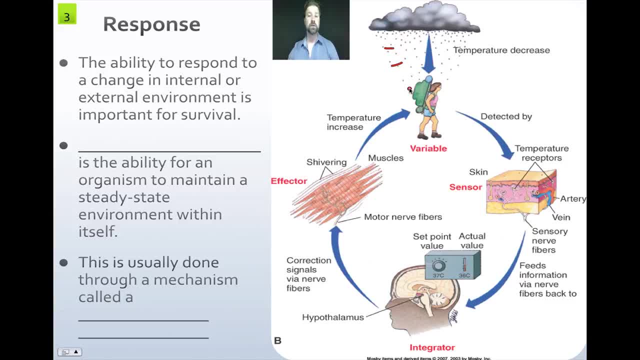 and we were close to home. we'd run back home and we'd put on new clothing. We'd put on new clothing because the environmental conditions have changed, So we're going to respond to that. In this case, here we'll say that this hiker wasn't close to home. 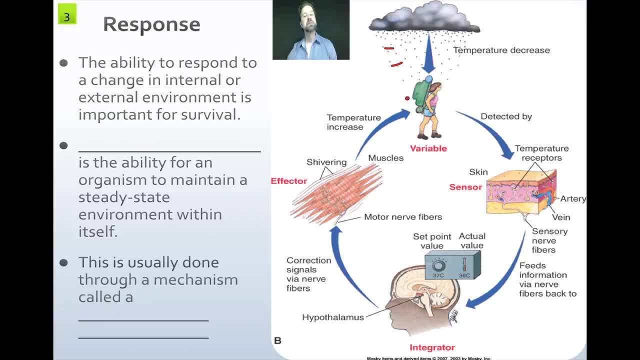 In fact, she was very far from home and she was caught without the proper clothing in an area she shouldn't have been in on that particular day. So what her body is going to do is going to try to prevent it from dying by using an internal 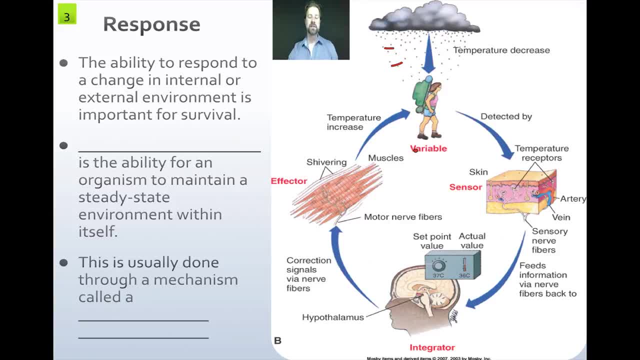 response mechanism. Her body wants to maintain a steady state. It doesn't want to decrease in temperature, because if it does, she may become hypothermic and that could lead to her demise. So what's going to happen is that those cold temperatures are going to reach her skin and 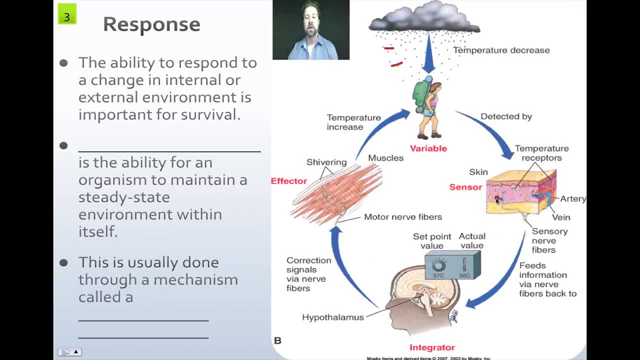 they're going to trigger, as a stimulus, particular nervous cell stimulations, their message is going to be transferred. So what's going to happen is that the temperature is going to be transferred from the skin, from these temperature receptors, down these sensory nerve fibers here and it's going to travel. 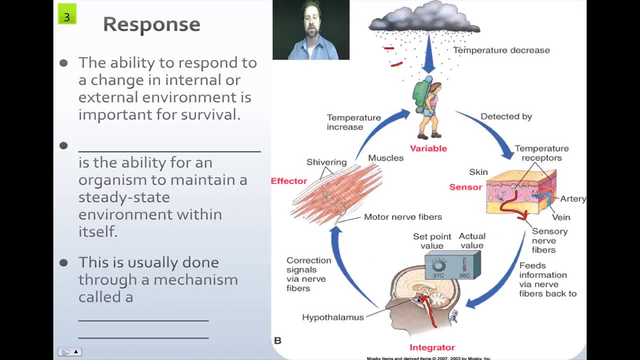 all the way up to this person's brain and it's going to reach a particular little tiny structure in the brain called the hypothalamus. The hypothalamus is like a thermostat on your house, So there's a set point value And if you live in Michigan, we know that we have cold winters and we set our thermostat. 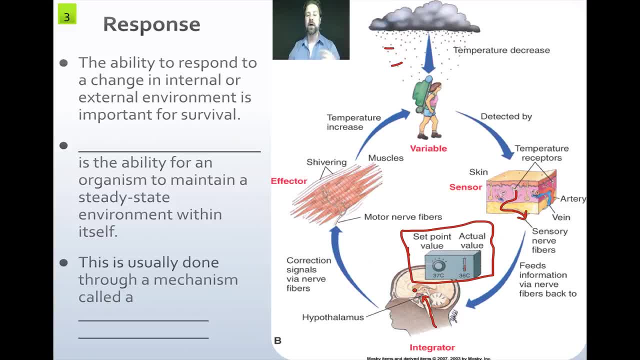 at a certain heat level that we're comfortable with. If the temp dips down below that temperature, then we're going to have a temperature drop And below that particular temperature, what's going to happen is that's going to trigger, by way of a stimulus, the furnace to kick on and the heat's going to blow out until 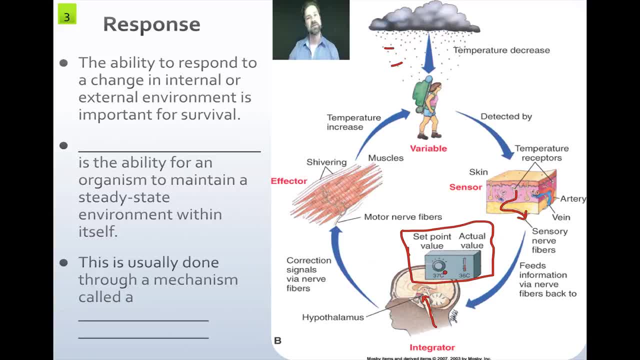 the ambient room temperature is above that particular temp that you set it at, And that will be a trigger to shut it off at that point, because we don't want it to run endlessly. So what's going to happen is the furnace of our body is going to be a correction signal. 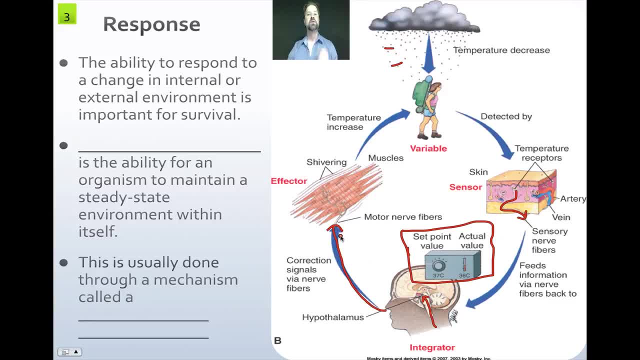 that's going to go to our muscles and it's going to cause them to start shivering, and it's doing that. so we build heat And the blood's going to be diverted to our core. we're going to start shivering, and that's. 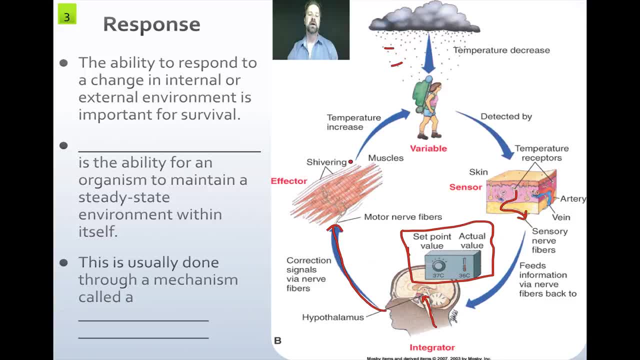 going to generate some heat on the inside, Maybe enough to get her to somewhere safe again. So it's going to try to bring it back to a steady state- 37 degrees Celsius or 98.6 degrees, And if she cannot maintain that and her body is working too hard and it dips down underneath. 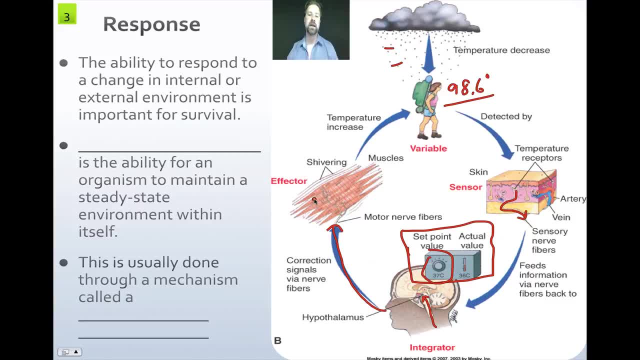 that 98.6, she may go hypothermic, which would be a bad case, A worst case scenario for her. And we have a name for that. We have a name for your body or an animal's body trying to maintain a steady state on. 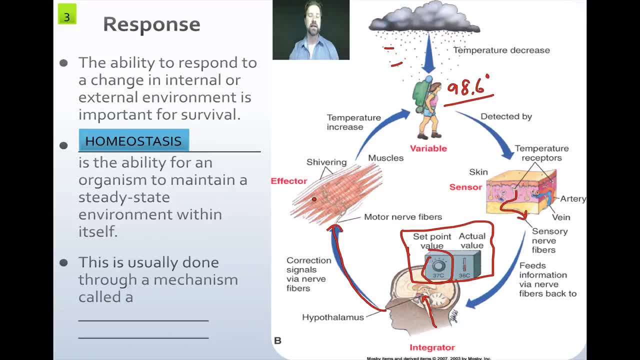 the inside and that's called homeostasis. We're going to look a lot into this concept this year And the particular loop that you see here- a loop from stimulus to sensing it, to integrating the message to an effector- that loop is going to be called a feedback loop. 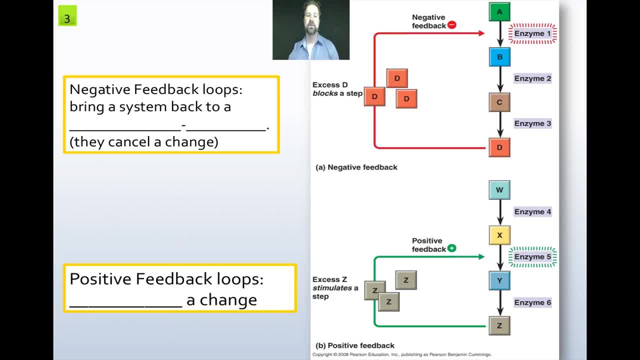 And this one in particular is called a negative feedback loop, because it brings a system back to a steady state. Now, inside our bodies, aside from temperature, we also have a whole bunch of complex chemistry going on as well, And in chemistry we know that we deal with reactants and we deal with products. 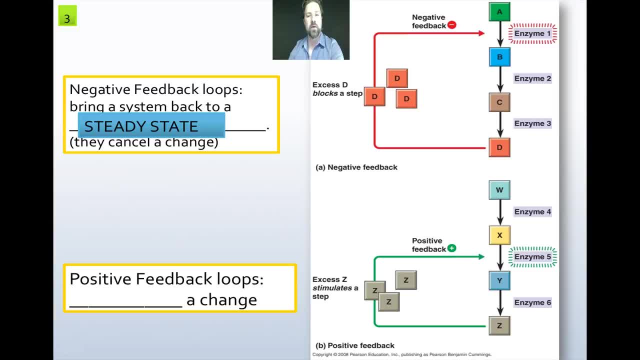 And we have to have a very specific amount of each one. If you go over too much, bad things can happen. If you don't have enough, bad things can happen. So internally it helps us if we're able to maintain a steady state as well. 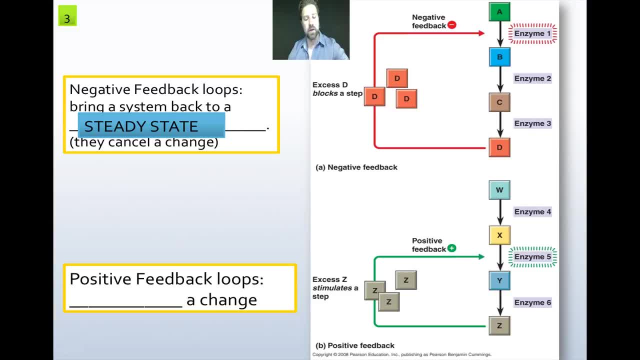 And through a negative feedback loop, we can see that happen also. So take a look over here and we can see that we have a reactant. so this might be something you ate. We'll call it A, And this A food substrate can be changed to B, because we know that food. 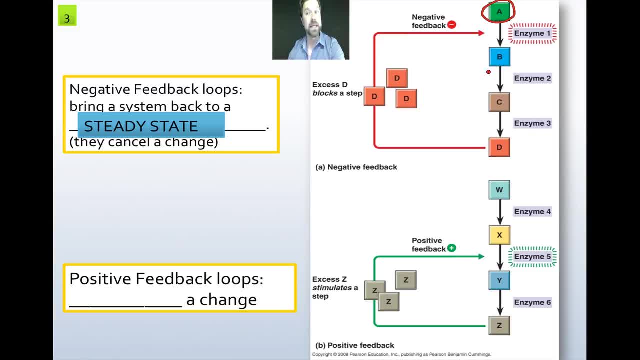 leaves us in a different form than when we first ingested it. So it's going to go through a number of changes And enzymes are going to perform a different function. It's going to provide a lot of those changes that we see. In this case, enzyme one is going to change substance A into substance B. Well, substance, 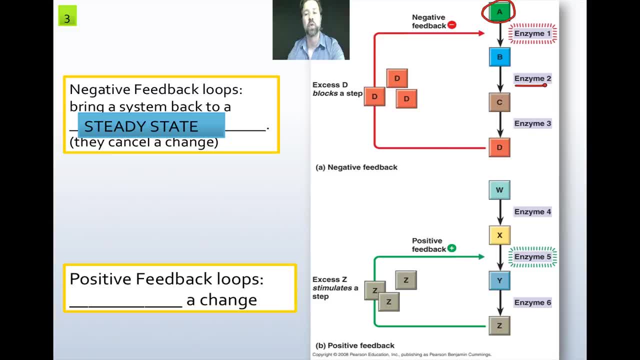 B is going to be changed to substance C by way of enzyme two, And substance C is going to change into substance D by enzyme three. So those three enzymes are necessary to change our food, our nutrition, from A to D, whatever that may be at a later time. 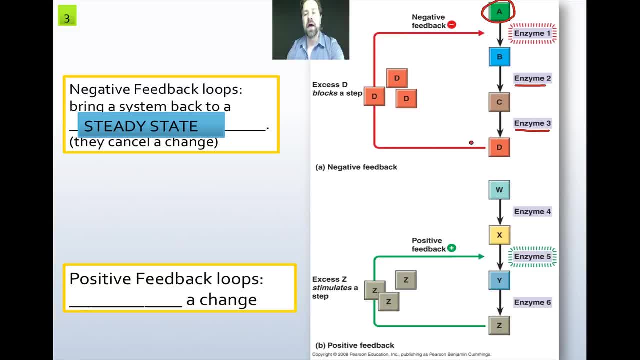 But Once we have enough D present, we have an internal mechanism that allows us to shut down this change because we don't need any more product D. So once you have an excess of D, it's going to send a signal to enzyme one to shut down. 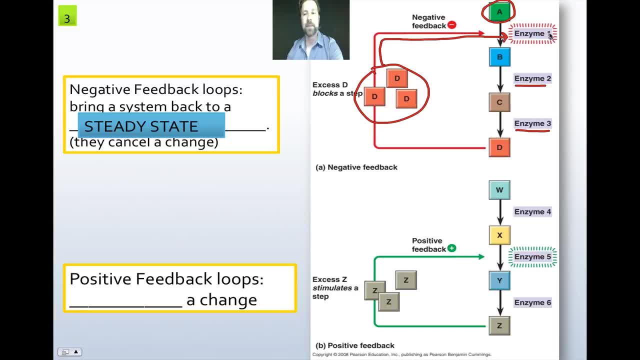 And if enzyme one shuts down, that means we're all topped off. We don't need any more of that particular chemical. So then A will probably pass through us at that point. We also have another system in play. It's called a positive feedback loop, which is kind of the opposite. 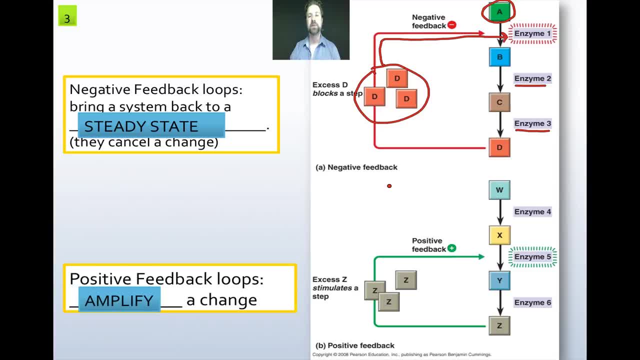 It doesn't bring things back to a steady state. Instead, it amplifies a change, It makes more happen. So in this case, here we have substance W, which changes to X at a later time, which changes to Y, which changes to Z. All of these changes are being helped by enzyme four, five. 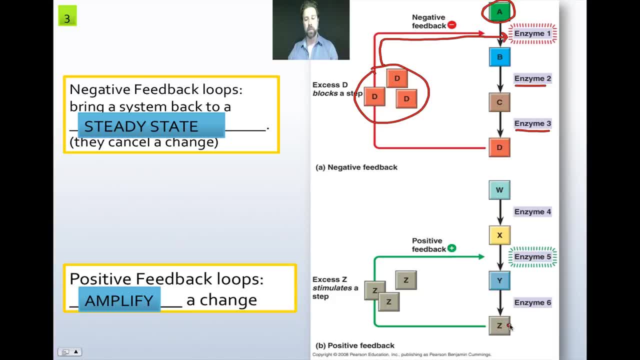 and six. All of them are on in order for this to happen. But So here, when Z is made, a large amount of Z doesn't shut it down. Instead, you can see this plus here It's going to cause more of it to happen. 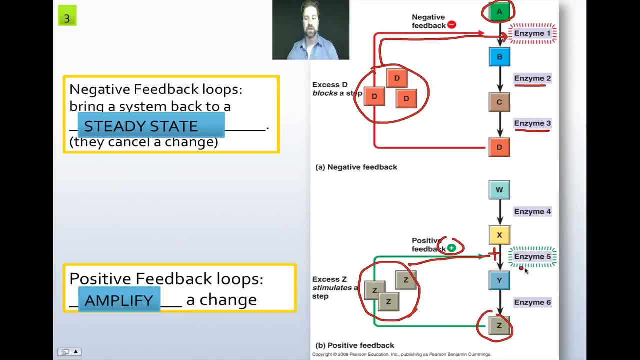 So what's happening now is that enzyme five has been supercharged, or maybe more enzymes have been produced to handle more W and eventually change it to Z. So in certain scenarios in organisms, you may want a positive feedback loop amplifying a particular change. 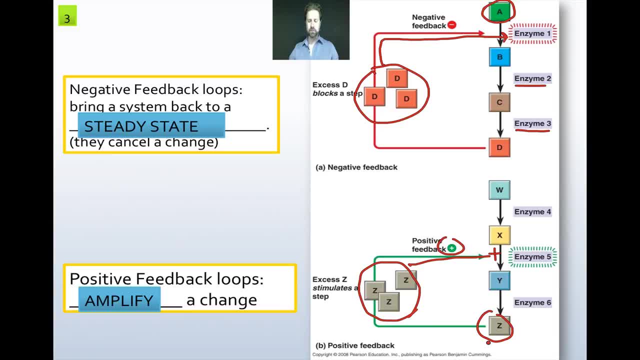 What are some examples of that? Well, if you think about childbirth For childbirth, once the birthing process has occurred, it helps the female body to push out that offspring, that organism with stronger and stronger contractions from the uterus. if we're talking about mammalian animals, 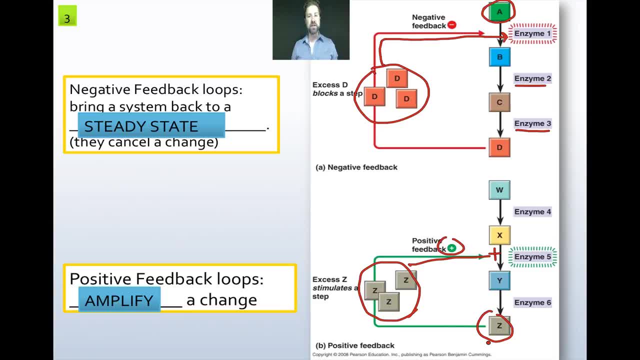 So as the uterus, uterine muscles are stretched, it's going to stimulate a stronger response, a stronger contraction of uterine muscles. Okay, To expel the baby. So in that case, positive feedback works very well during particular processes, one being 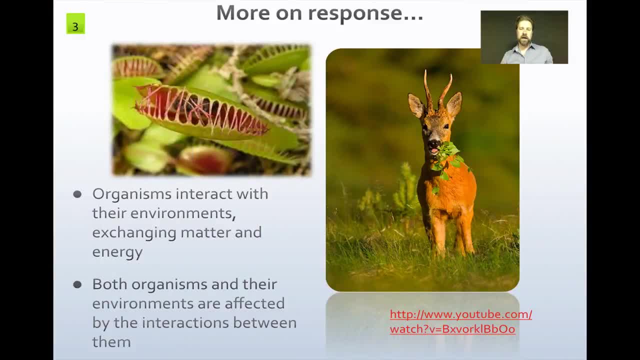 childbirth. One additional aspect when thinking about living things responding to their environment is the fact that they exchange matter and energy with their immediate environment. So whether it's a Venus flytrap exchanging matter with the food that it's caught, or this animal here that's enjoying a leafy meal, 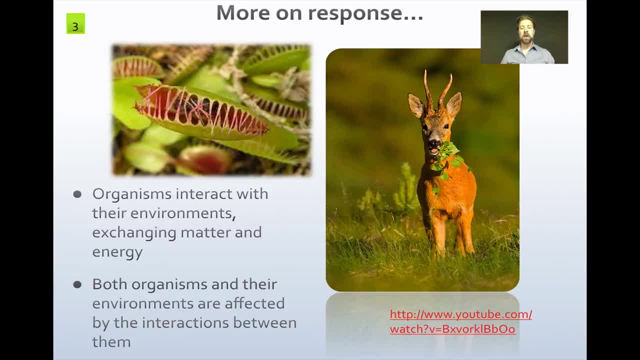 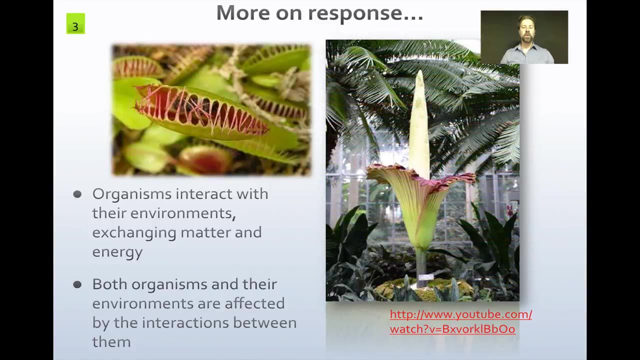 Matter will be transferred to the other species and energy will come with that matter. When animals release waste, that waste can be converted from waste to nutrients for growing plant matter as well. This past summer we saw a flower bloom called the corpse flower. 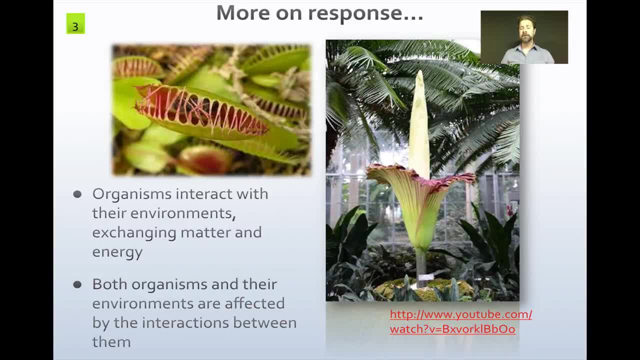 This flower is held in a botanical garden in England And the key interesting trait about this flower is that it's a plant that can be used for various purposes. It can be used for various purposes. It can be used for life. It can be used for a child. so bringing it back to life is wonderful because it can be. 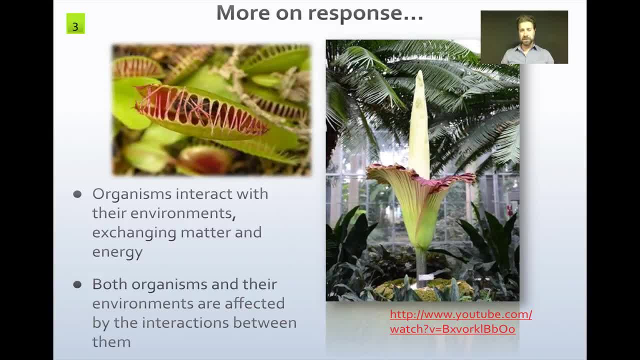 used for the child. This flower is sort of a family thing. This flower can be used for any other purposes, And what I love about this flower is that it smells like a dead, rotting carcass when it blooms. Now, what evolutionary adaptation would that serve? 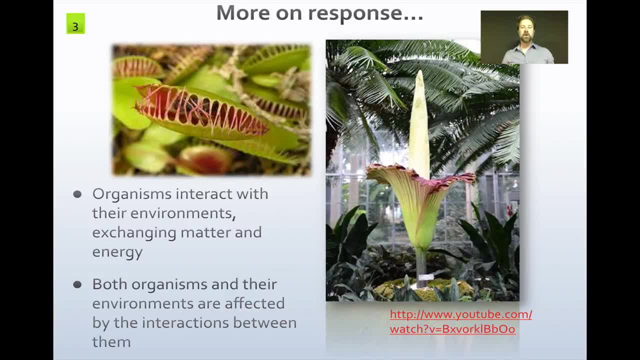 How would this benefit this flower? Well, here's the thing: These flowers tend to be solitary. There's not many around, So when it blooms, it's going to need a means to carry its pollen to another plant in order to fertilize it. 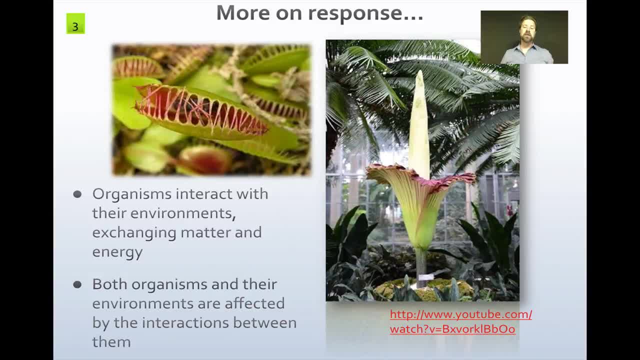 So this one does so. draws in flies, of course, and the flies are going to feed on this blooming flower, and as they do so they're gaining nutrients. but there is also matter being transferred. the pollen from this plant is being transferred to the flies, which may land on another flower which will work to cross pollinate. 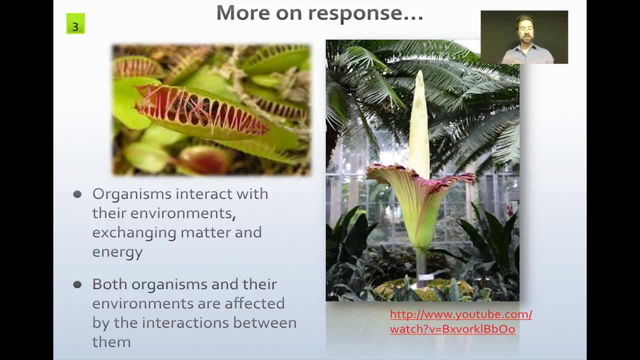 that other flower. so there is a exchange, an exchange going on between matter and energy by this particular flower by smelling like a corpse, and that's where it gets the common name corpse flower, another type of great lakes. example of exchanging matter and energy and responding to the environment, we can look at an invasive species called the sea lamprey. 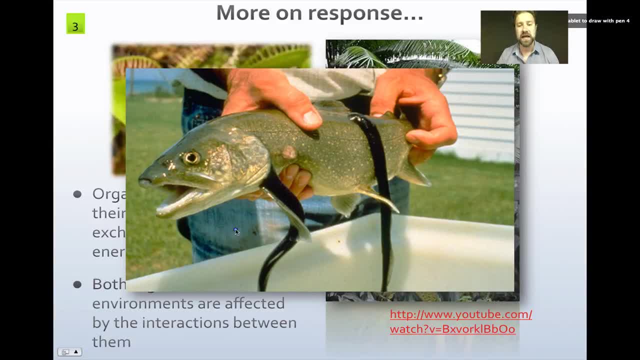 now, the sea lamprey, as you can see, is not the fish, but instead it is this guy right here, and what this guy does is he's going to latch on to the fish and he's going to chew a hole through the side of the fish and it's going to extract matter which it's going to use for. 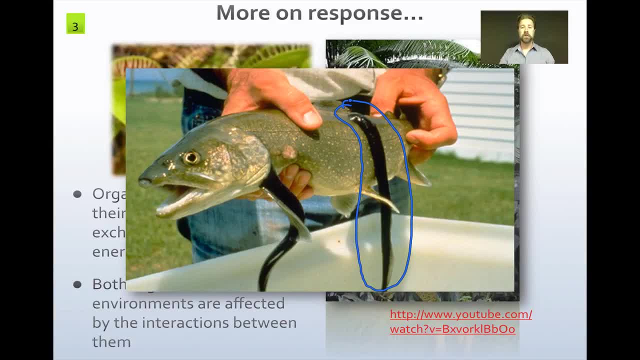 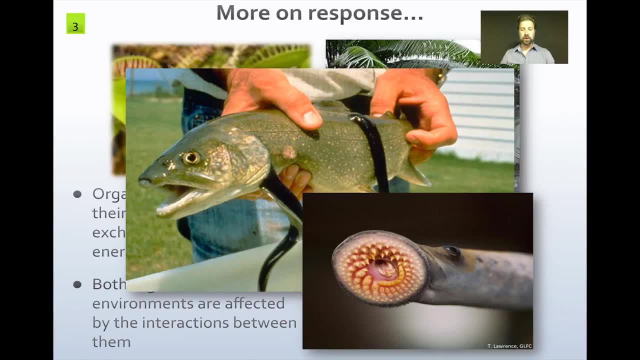 its own energy stores for as long as possible. how does something like that attach to a fish? well, it's kind of- uh kind of medieval look in here and pretty brutal. but basically there's a suction disc on the front of this animal right here. you can clearly see it, and it has a number of rows of 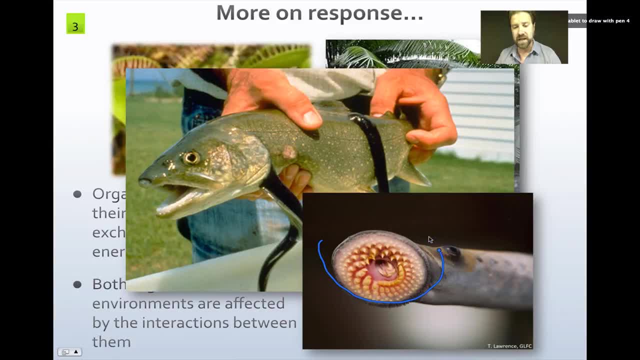 teeth as well, and these teeth are going to help to kind of lock in on the side of the fish's tissue. it has what's called a rasping tongue in here which is going to bore a hole into the side of the fish and it's going to be able to take the nutrients from the fish. does it hurt the fish? of course, 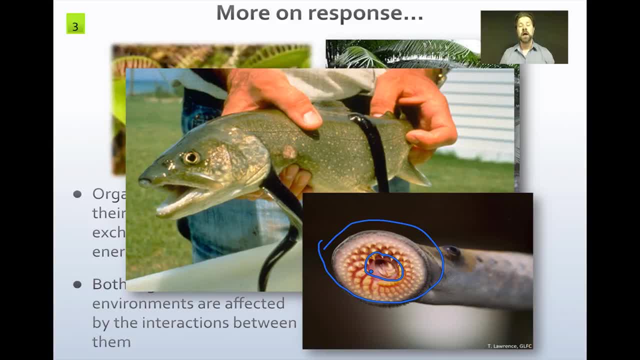 this is a parasite, so eventually it's going to weaken this fish so much the fish may die, uh, from the wounds that it's going to take on from the lampreys latching on to it. now, how does a fish like this get into the great lakes? well, uh, this one has almost a 70 to 80 year history of entering. 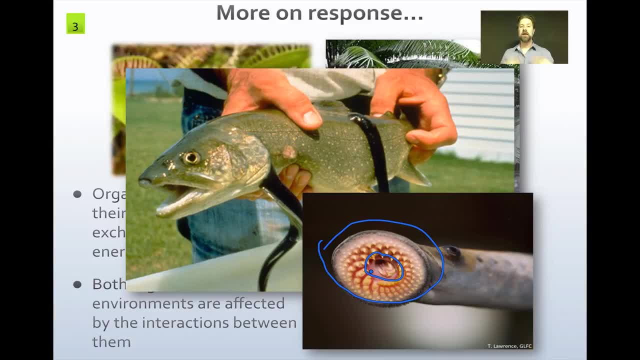 the great lakes, and when it found the white fish population of the great lakes, it found a great prey species in order to attach to it and then further its own life by doing that particular act of latching on, uh, boring a hole and sucking out the nutrients. now, of course, this is problematic because a lot of people 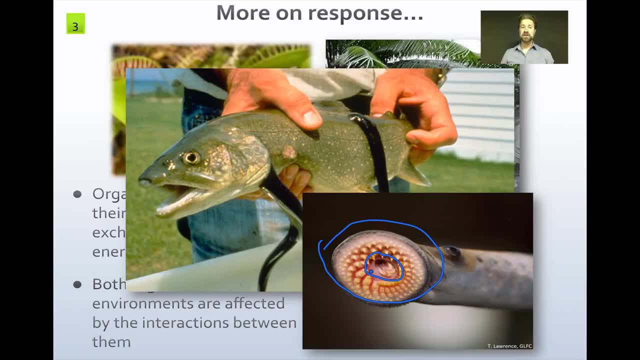 were relying on the great lakes to be productive, and these big, large fish could feed a lot of individuals, so we had to look into control mechanisms. now, one thing that we studied was the fact that when these lamprey die, they release a chemical which the other laminates seem to acknowledge. they seem to sense this death chemical released when lamprey die, and 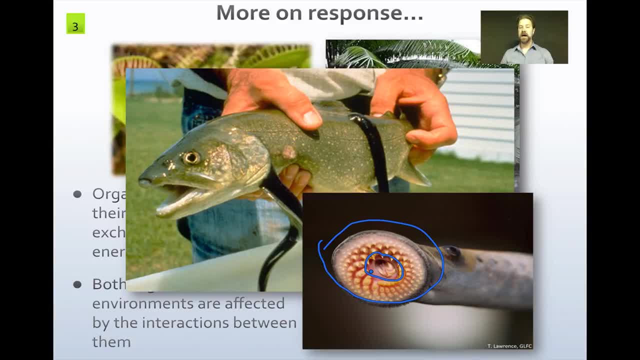 they respond to it by getting as far away from it as possible. so i want you to think of this scenario. we'll think of a horror movie. you're out in the middle of the woods, in the absolutely in the middle of nowhere, and you're afraid because you're lost and you start coming upon spikes with skulls. 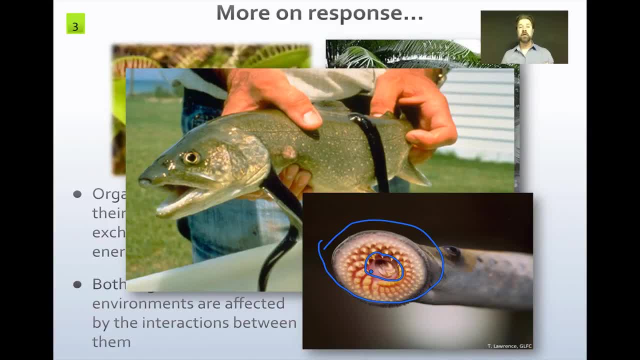 on the tops of them and you wander around, and the more you wander around, the more skulls on spikes that you see. now, as a human, you're probably going to have the fight or flight response kick in. you're going to try to get as far away from that threat as possible because you feel like your skull. 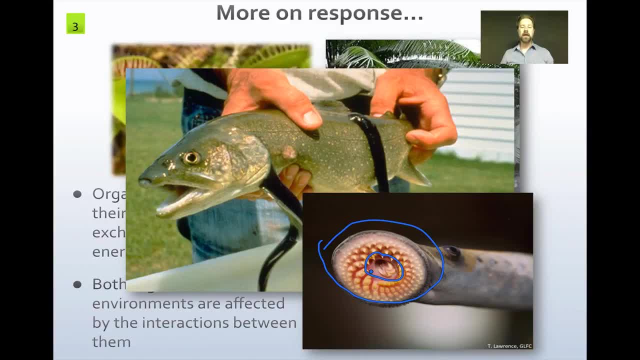 might be the next one on a spike. so these lamprey are kind of the same way their our senses sight. we see those things, we respond. their sense is through chemicals in the water. they're able to smell these particular death chemicals released when a lamprey dies and get out of that area because they have 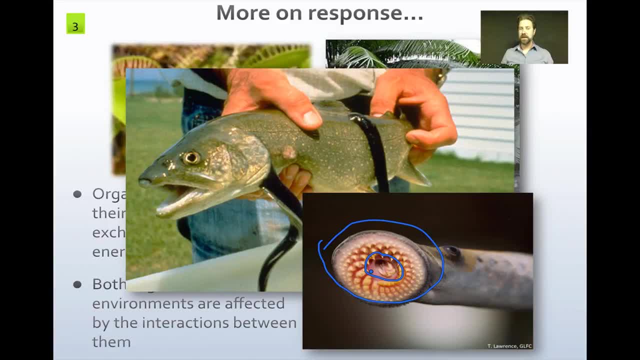 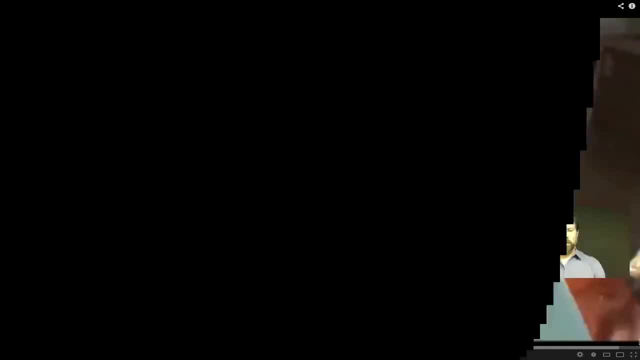 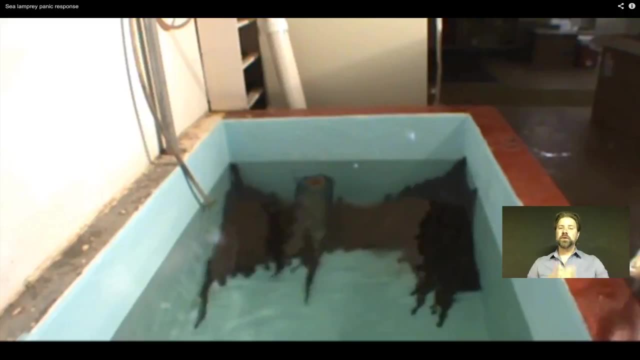 evolved this particular adaptation to keep them safe. so we're going to watch a little clip here on what happens when a lamprey senses this death death chemical. this is a study from michigan state. they were looking at the sea lamprey and they were trying to determine whether there were some. 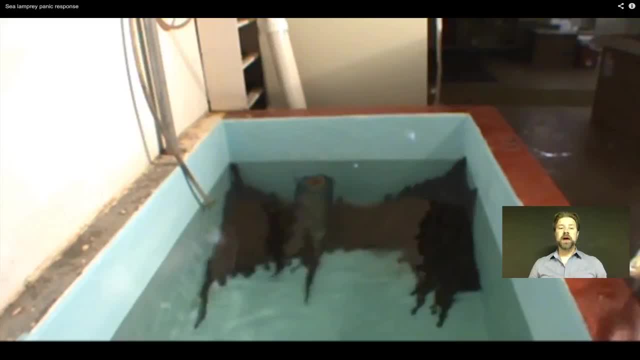 control methods that they could put into play to keep the population of sea lamprey down, because the higher the population is of this particular cartilaginous fish, the more damage they're going to do to our living system, and that's the reason why these fish have such a terrible life history. 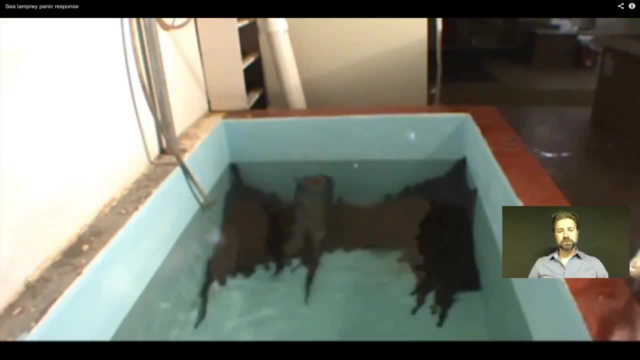 native sport fish that we have here in the Great Lakes region. So by looking at a chemical that can cause sea lamprey to move out of a given area, it may be possible to trap them in a given area and use a lampreyside or possibly trapping methods to catch these sea lamprey. So there's not so many. 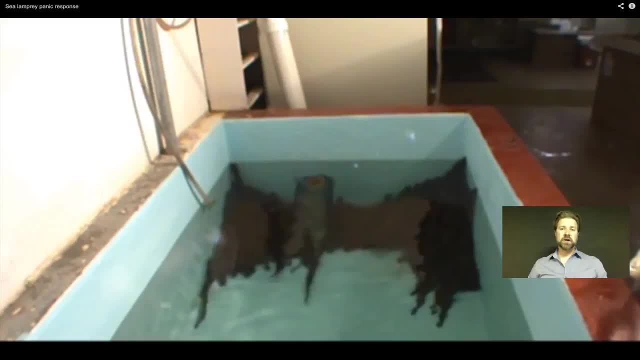 of them swimming around in the Great Lakes region. So what we're going to see here is a researcher who's adding this chemical to this tank, and you can see at the bottom corner of the tank here a lot of sea lamprey that are just kind of hanging out. They're going to put this chemical. 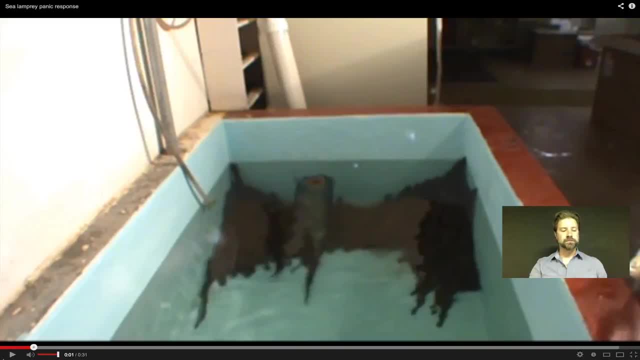 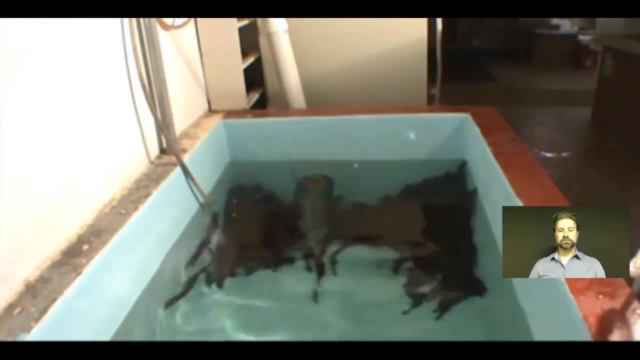 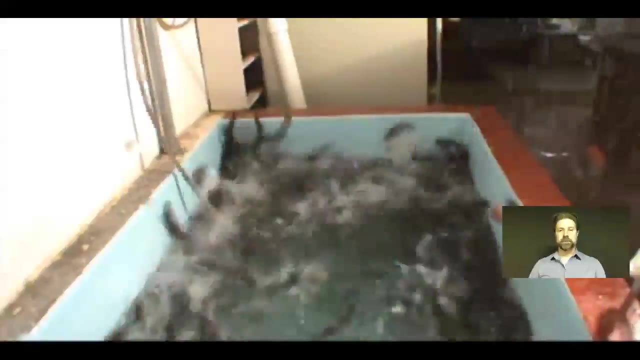 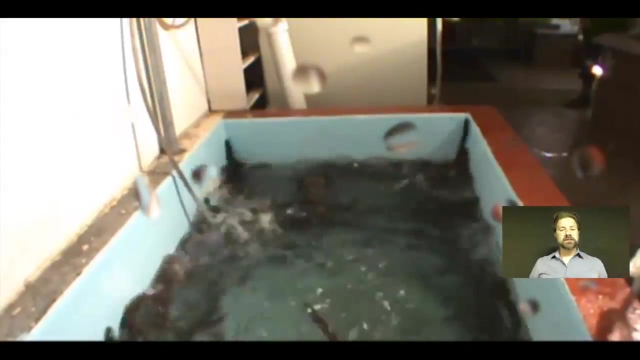 inside the water and we're going to watch and see what happens. So, as you can see, this is a pretty extreme response to its environment. It's sensing that there's depth in the area, And each individual animal here, of course, does not want to die. 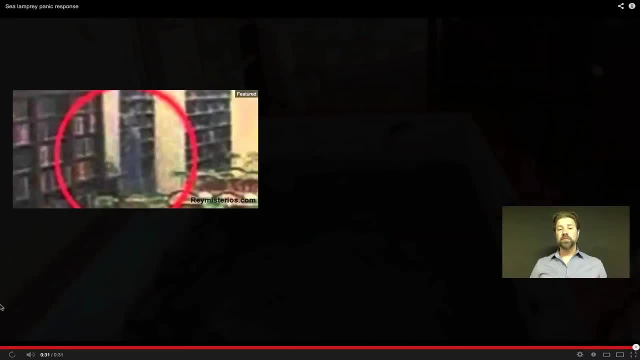 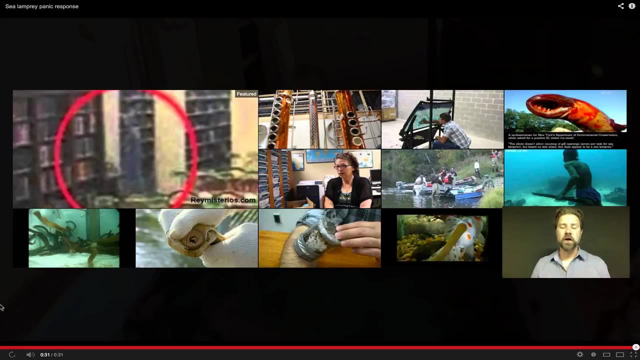 It wants to extend its life as long as possible and reproduce as well. So in order to do that, what we see happening is we see a flight response. It's getting as far away from the possibility of being around this death of land prey as possible. 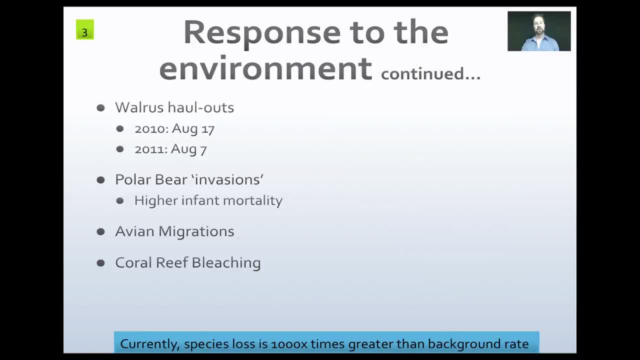 Some other remarkable types of responding to the environment. One is called a walrus haulout, And we're keeping an eye on walrus haulouts because of climate change And, as we know, as climate changes, one of the regions that's affected the most is the polar region. 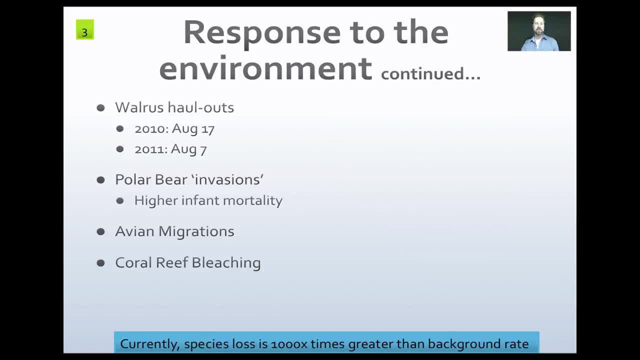 And what we're seeing is a dramatic decrease in the ice amount in those polar regions- Ice that's very, very important to some of the animals that live in those polar regions, such as the walrus. So I want you to take a look at this picture here. 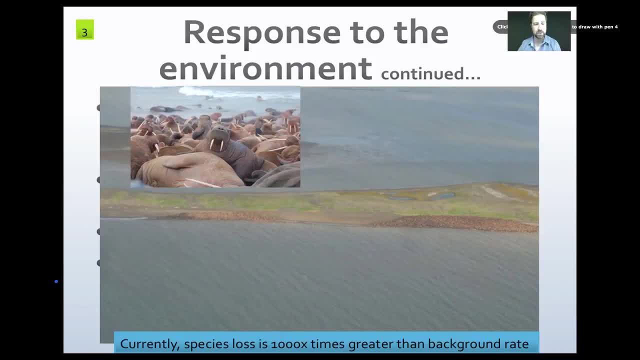 And you can see a couple of masses. I'll put my walrus picture up there. What this is here? we know what this is, But what we can see here are thousands upon thousands of walrus that have hauled themselves out of the ocean because there's no sea ice left. 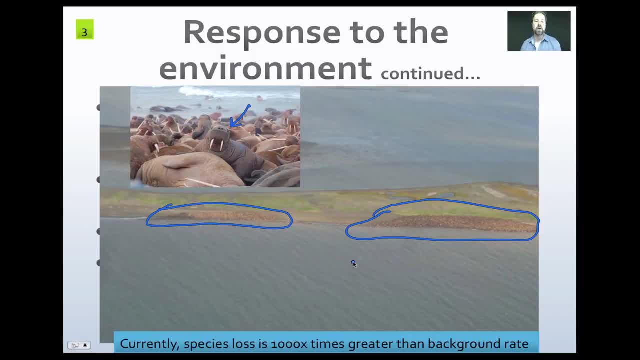 Now females will bear their young on floating ice because it's much safer, They're closer to the food and they're safe from being trampled. So you can imagine a baby walrus in this situation. If there's something that causes a stampede, they're likely to get crushed. 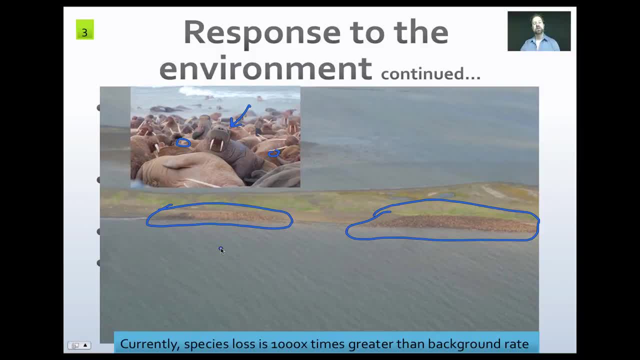 They're likely to get crushed. The weight of stampeding walrus- And we're starting to see a decline in their numbers as well- as they have to haul out early and young have to be tended to in these massive groups. here You see a much lower incidence of survival for the infants. 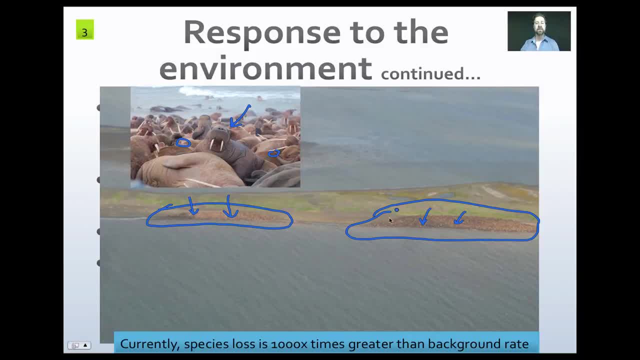 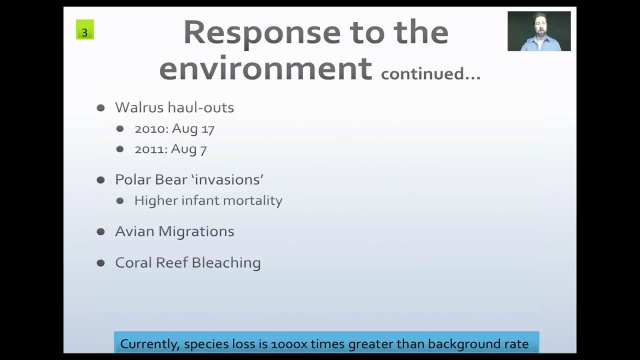 Very low if the infant has to be born in these conditions here. Another one that we look at carefully, also from the polar region, are the fact that polar bears have a lot of weight. Another one that we look at carefully, also from the polar region, are the fact that polar bears have a lot of weight. 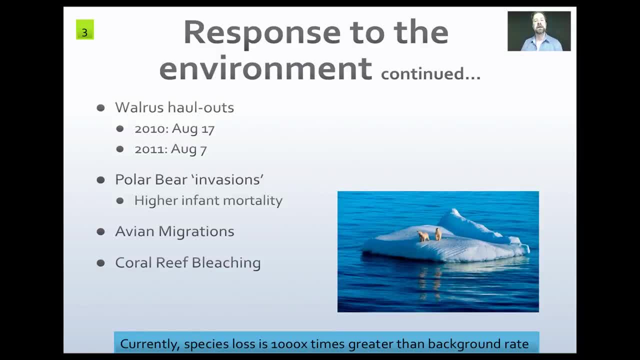 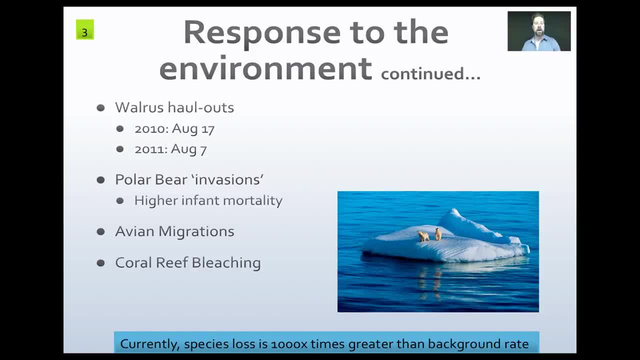 The reason is because their ice is also going away in the same manner And they need the ice to properly hunt because their main food is seal and they're able to stealthily hunt the seal by way of the ice. And they need the ice to properly hunt because their main food is seal and they're able to stealthily hunt the seal by way of the ice. 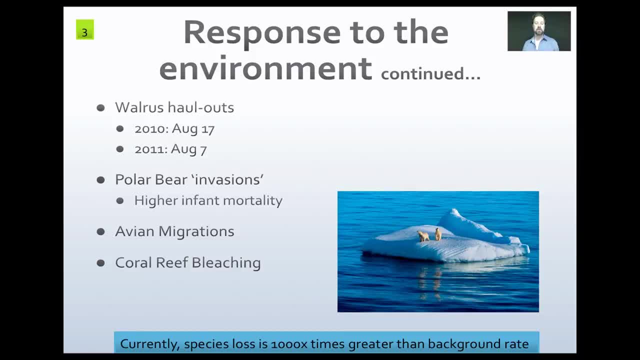 And they need the ice to properly hunt because their main food is seal and they're able to stealthily hunt the seal by way of the ice. And they need the ice to properly hunt because their main food is seal and they're able to stealthily hunt the seal by way of the ice. 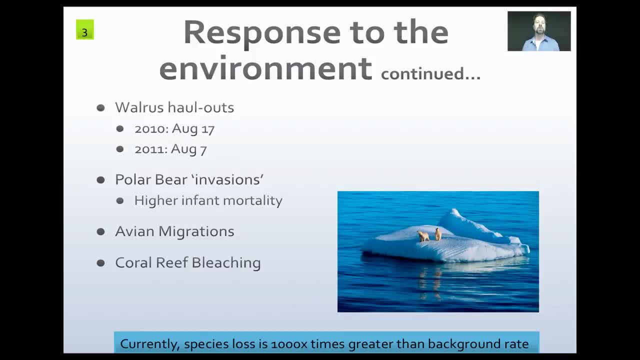 And they need the ice to properly hunt because their main food is seal and they're able to stealthily hunt the seal by way of the ice. And they need the ice to properly hunt because their main food is seal and they're able to stealthily hunt the seal by way of the ice. 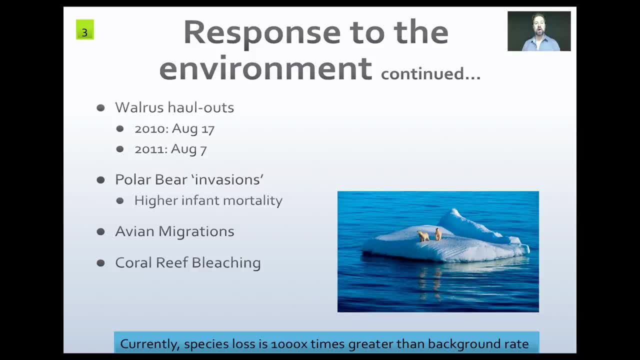 And they need the ice to properly hunt because their main food is seal and they're able to stealthily hunt the seal by way of the ice. And they need the ice to properly hunt because their main food is seal and they're able to stealthily hunt the seal by way of the ice. 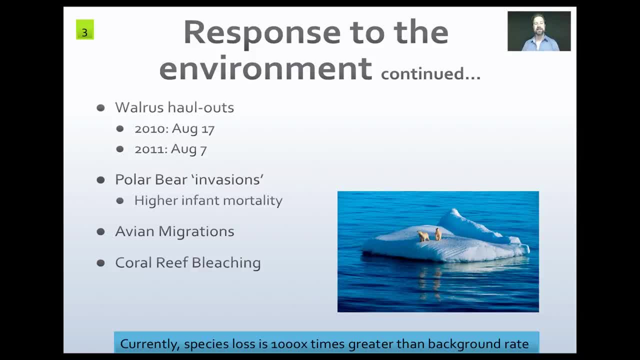 And they need the ice to properly hunt because their main food is seal and they're able to stealthily hunt the seal by way of the ice. And they need the ice to properly hunt because their main food is seal and they're able to stealthily hunt the seal by way of the ice. 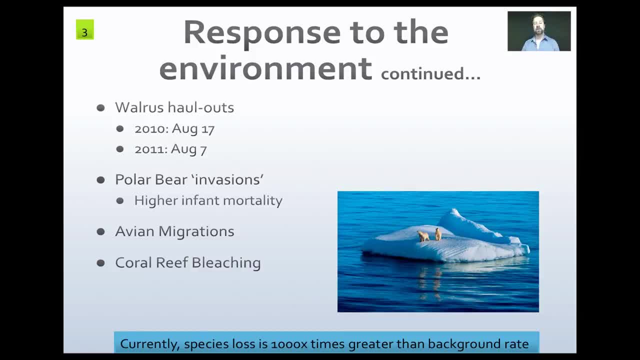 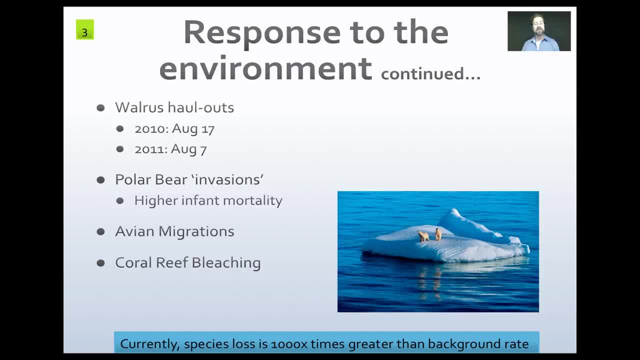 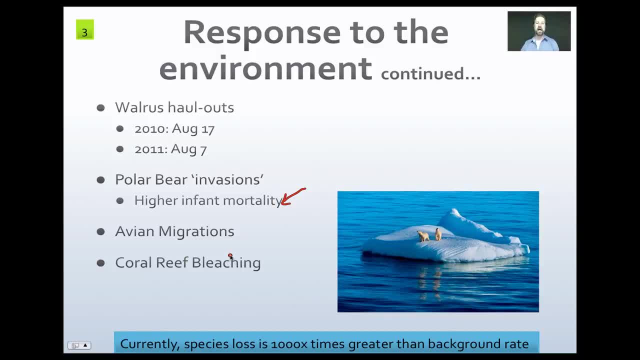 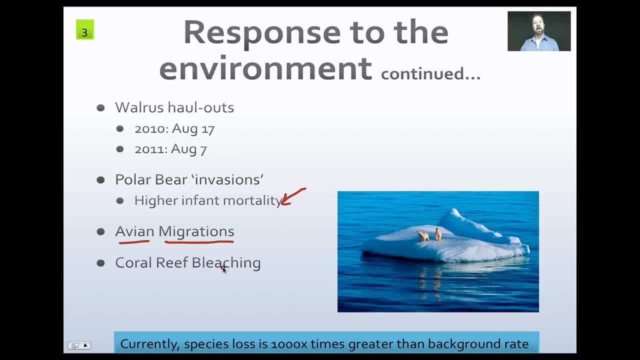 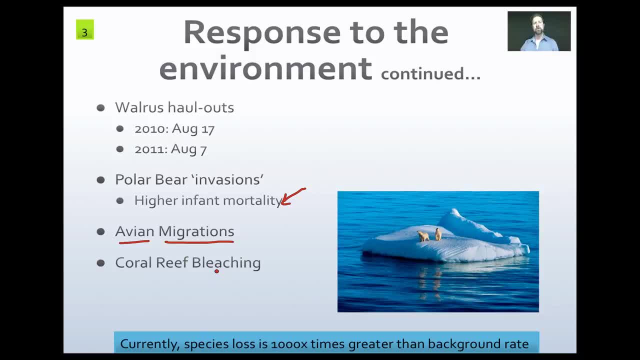 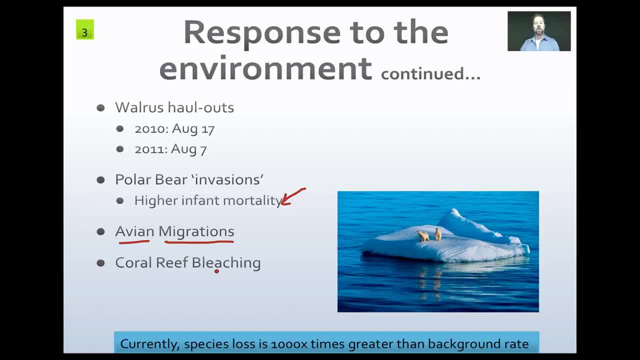 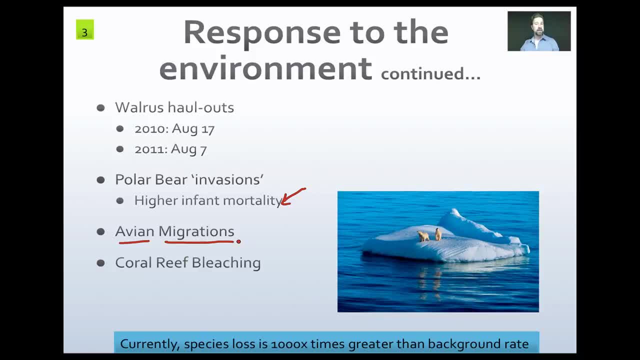 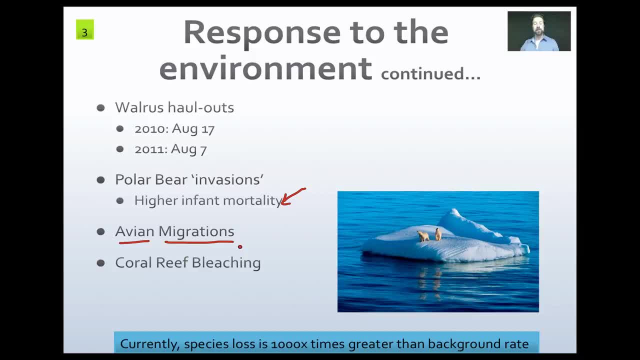 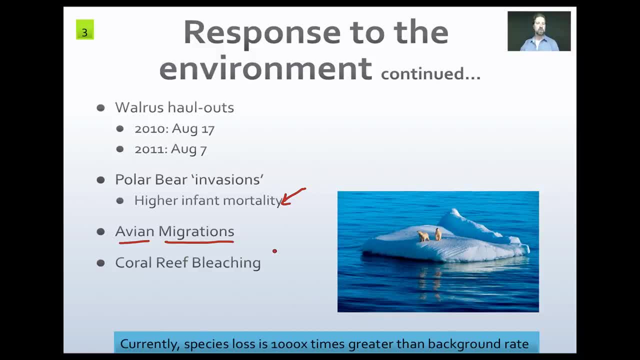 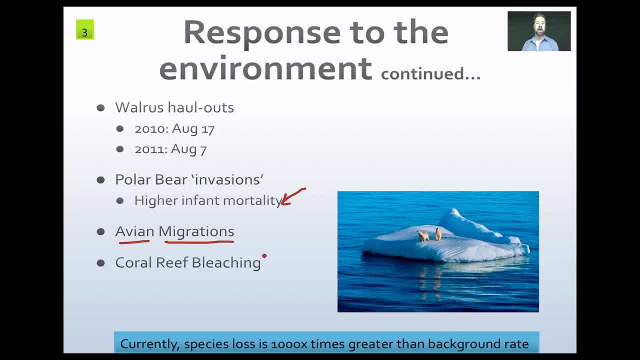 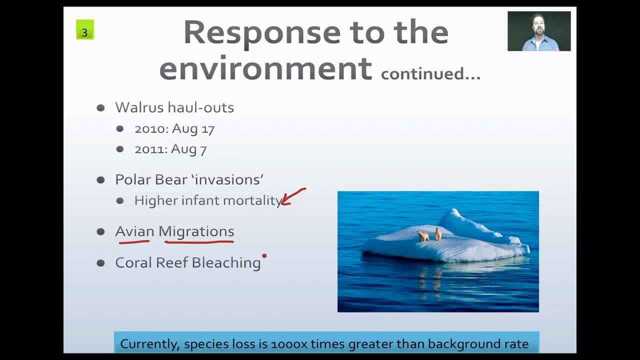 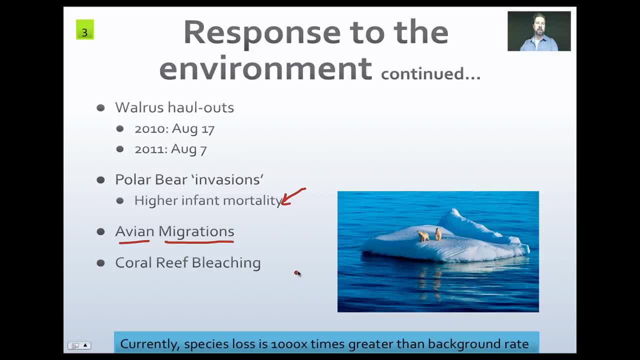 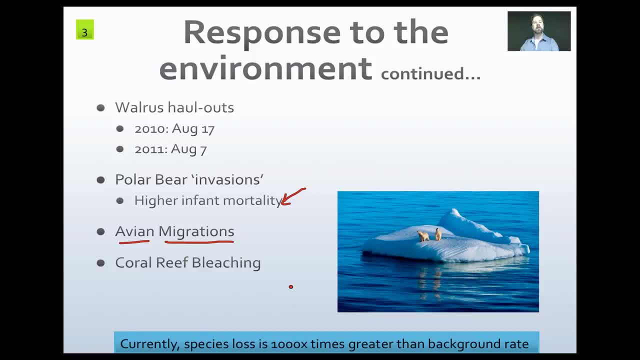 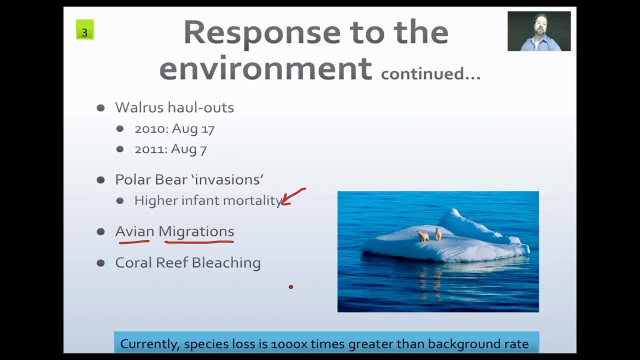 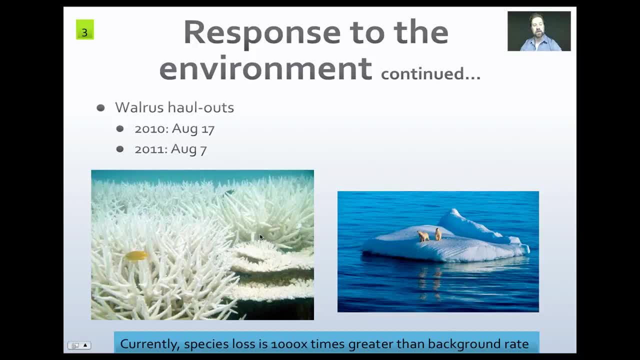 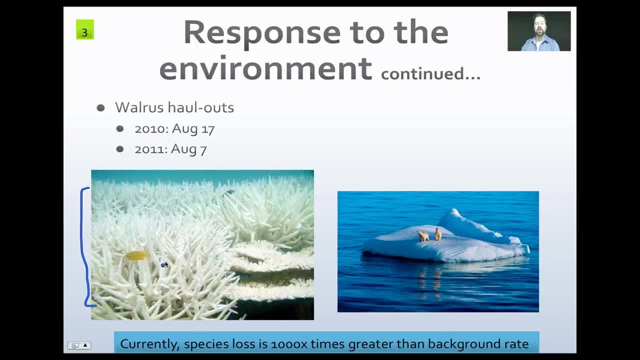 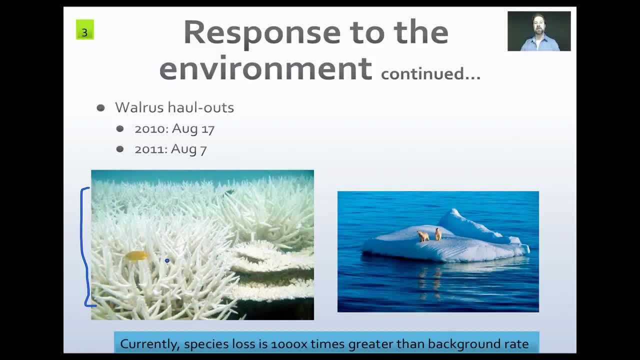 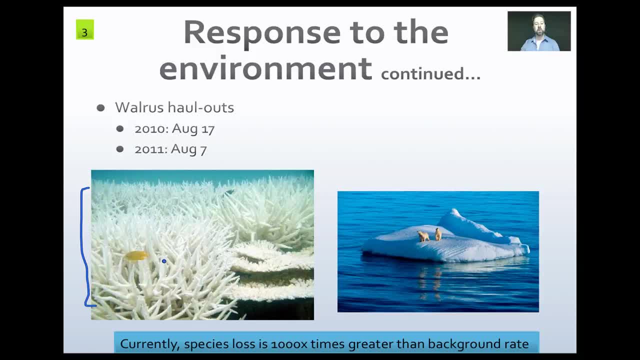 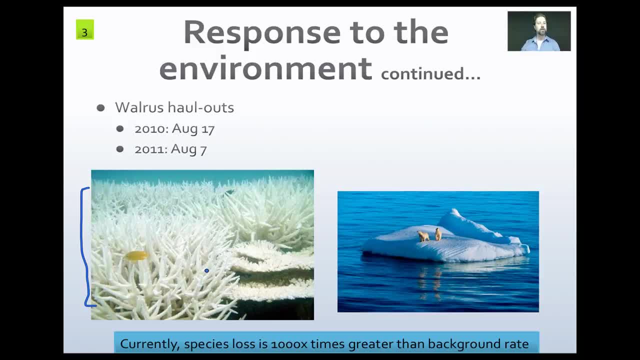 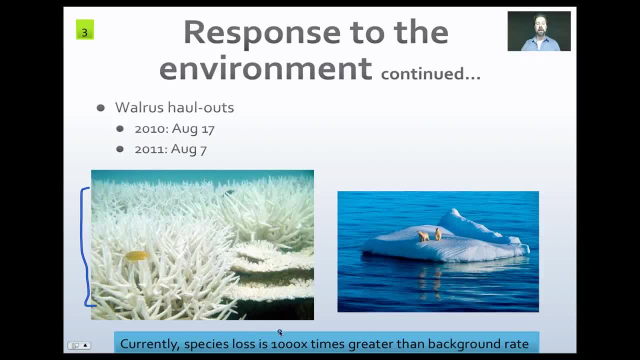 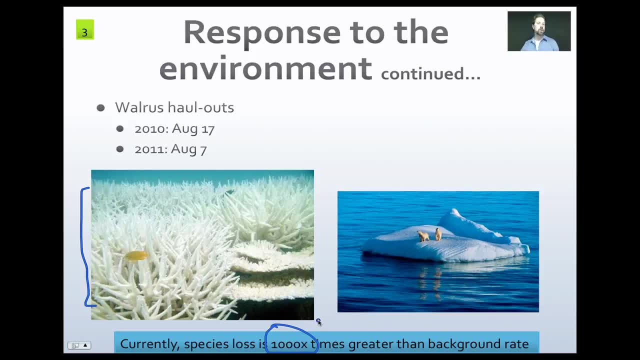 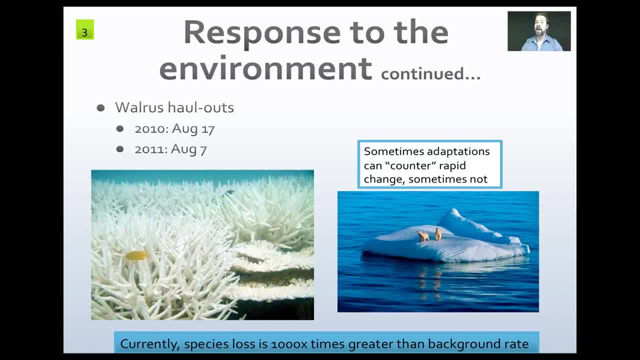 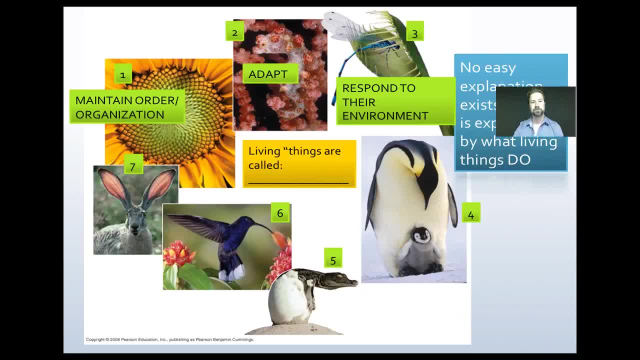 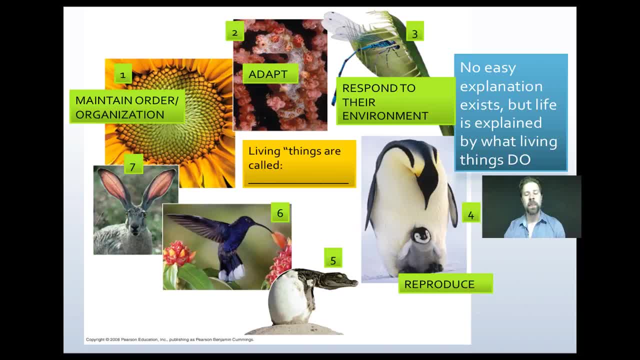 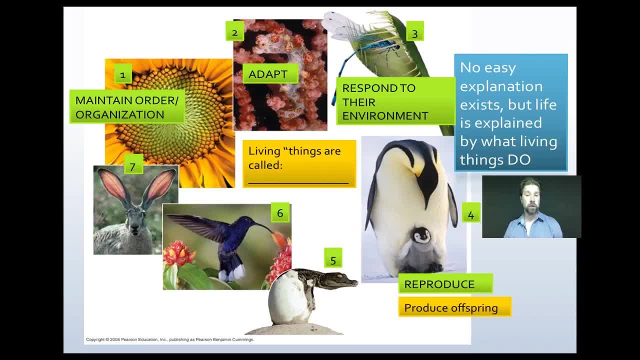 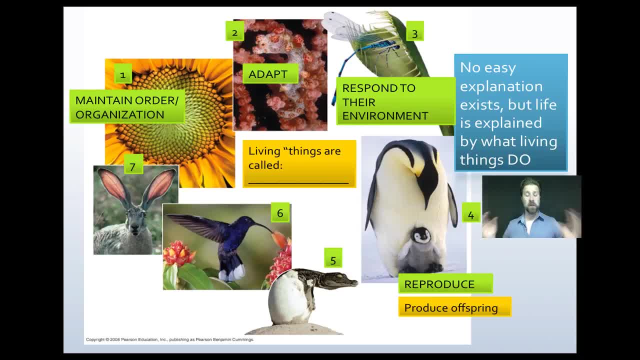 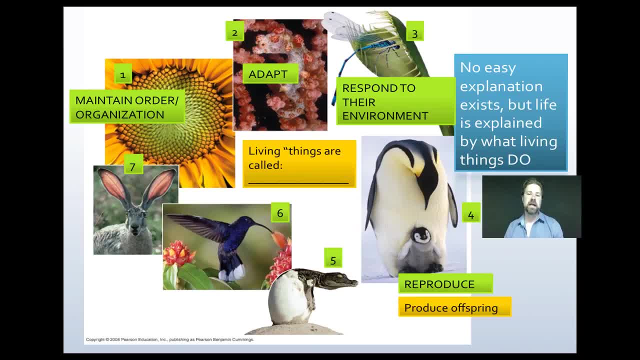 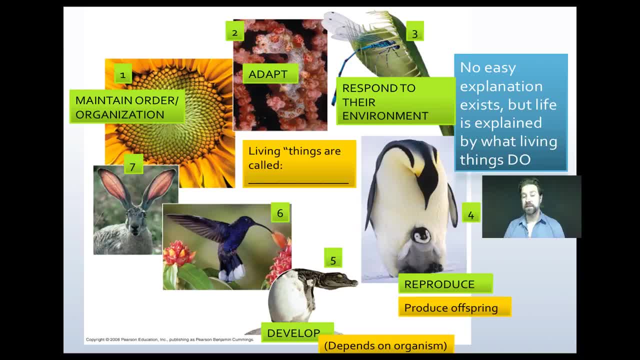 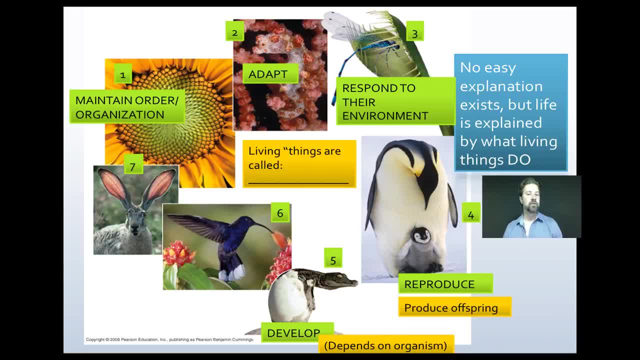 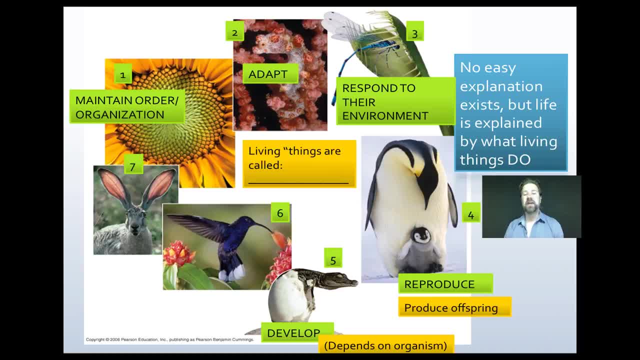 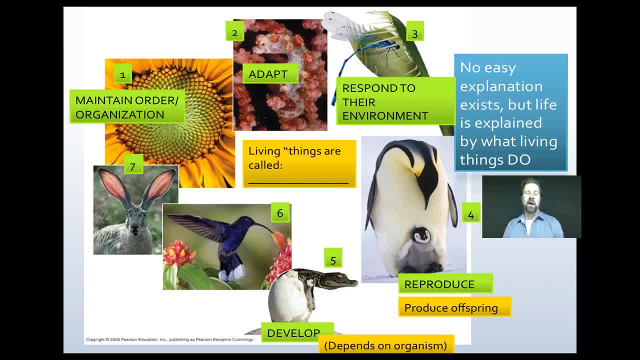 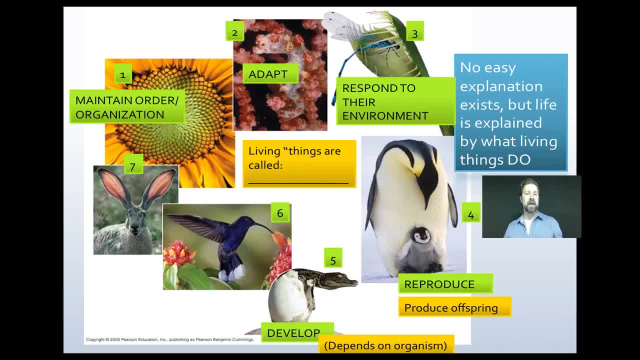 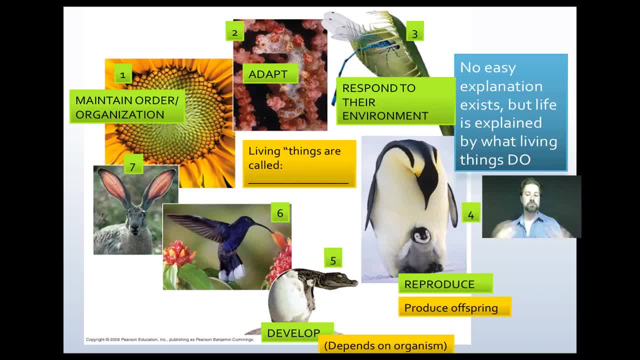 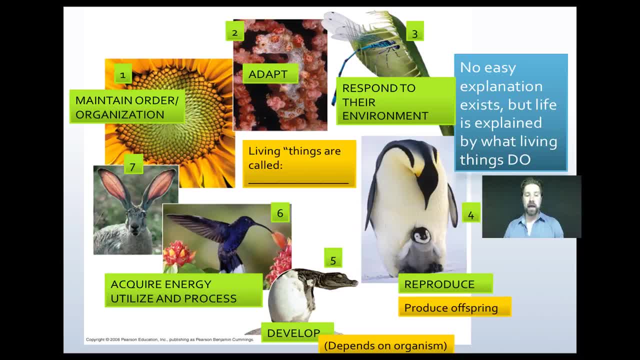 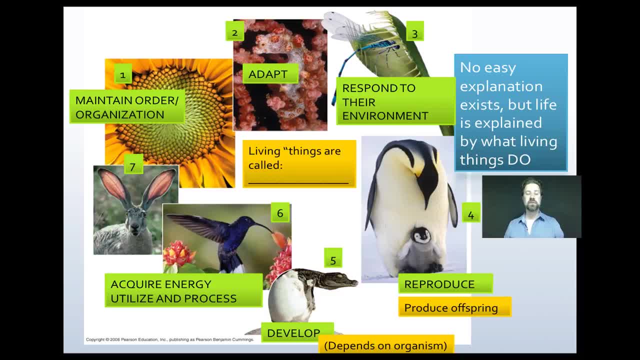 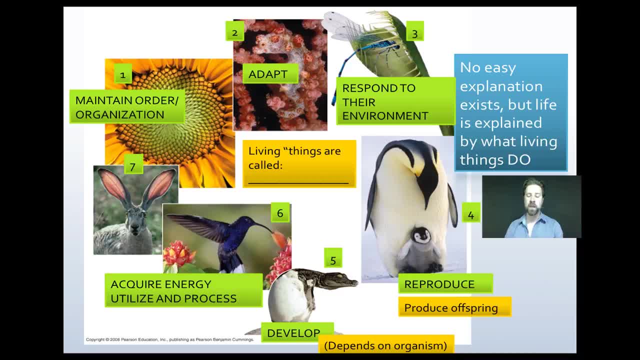 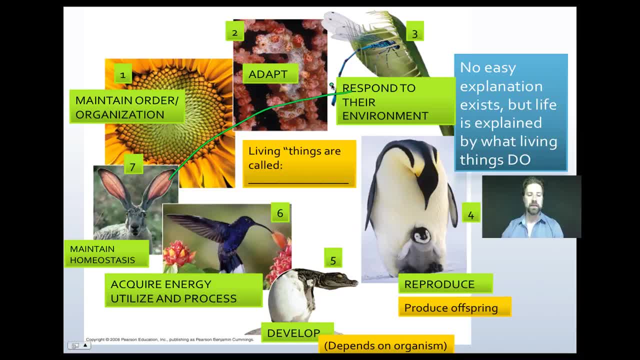 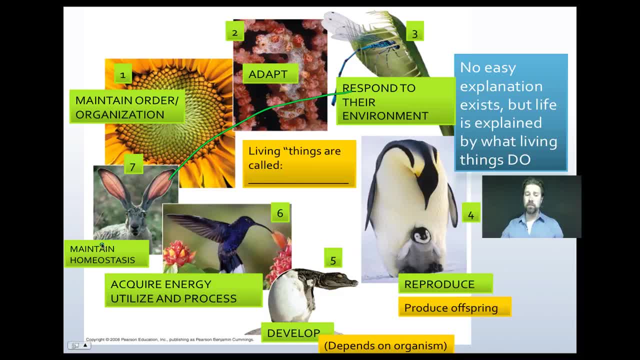 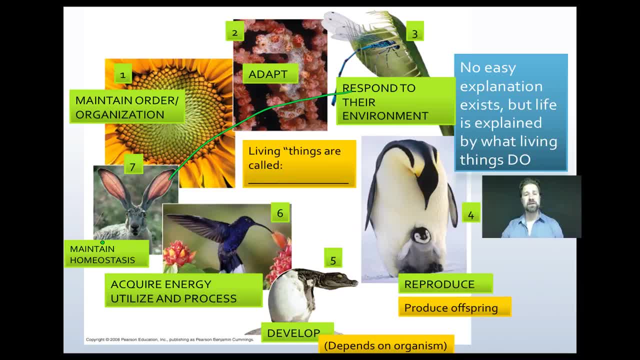 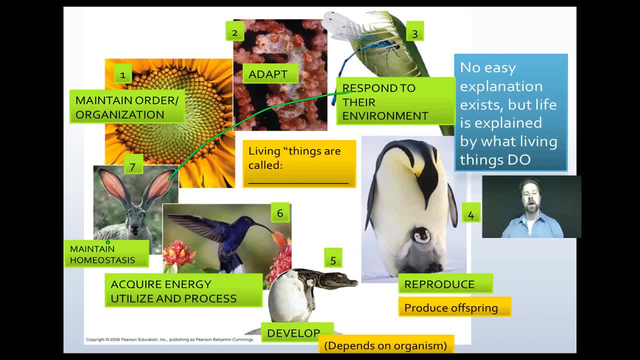 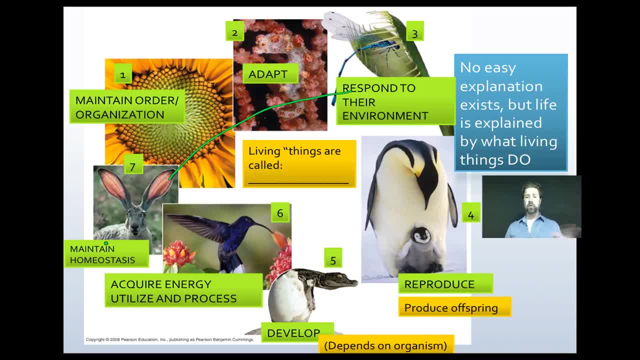 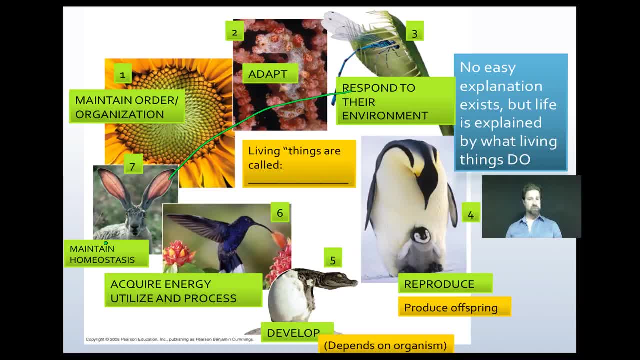 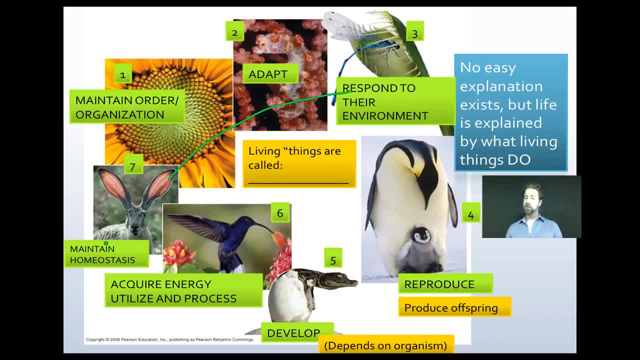 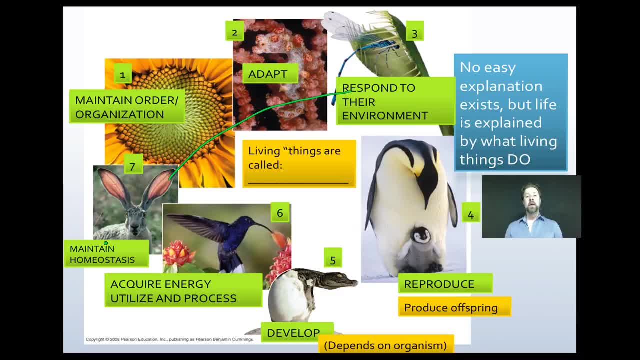 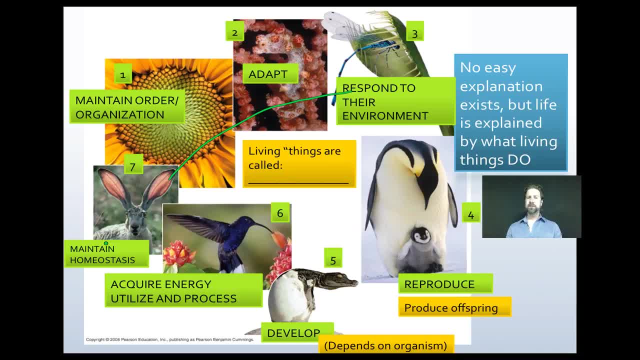 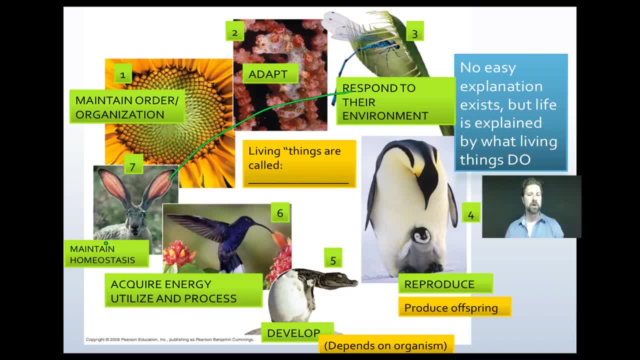 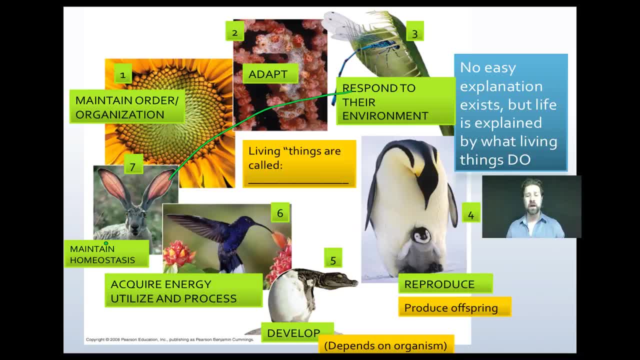 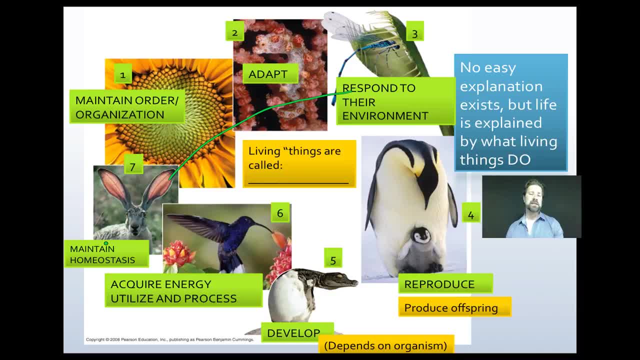 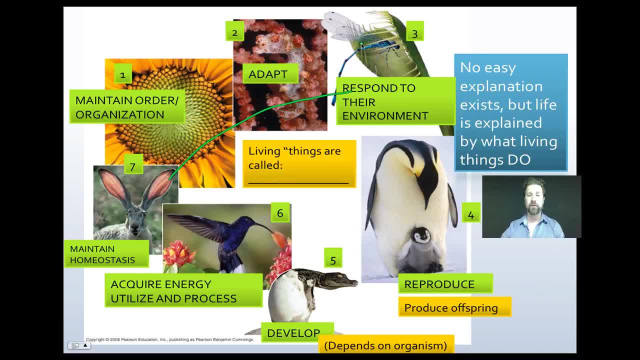 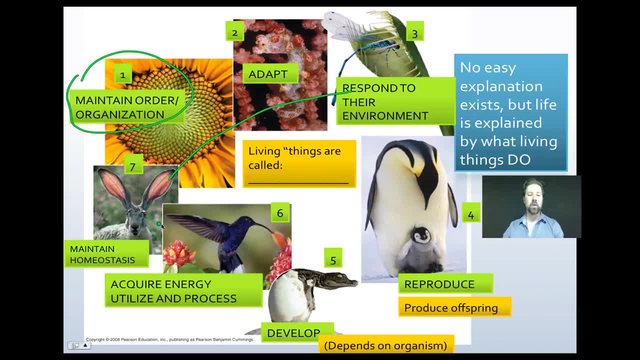 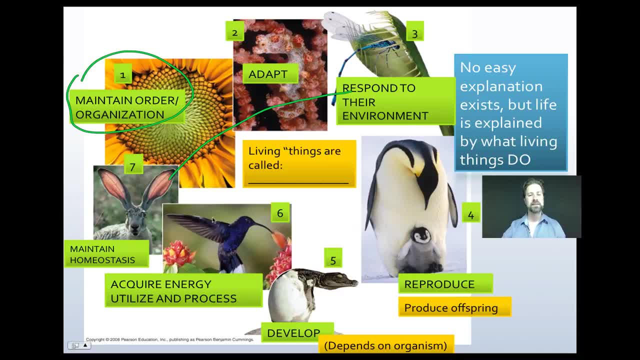 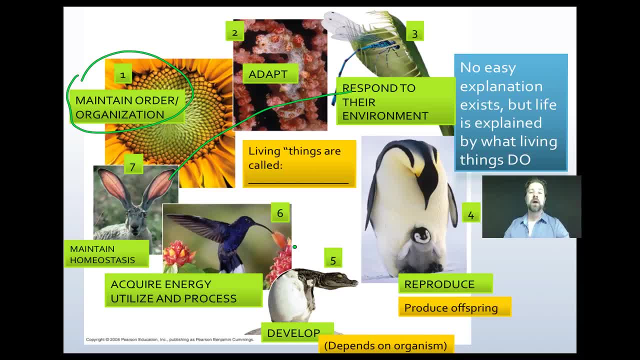 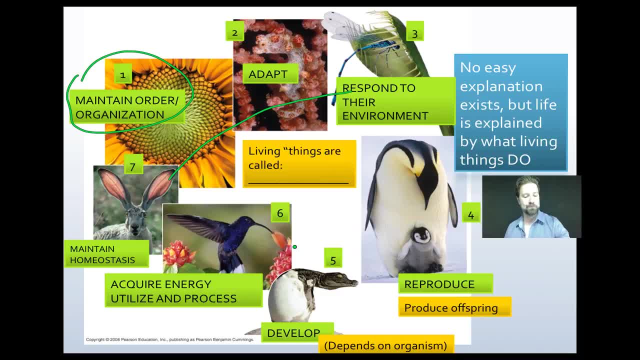 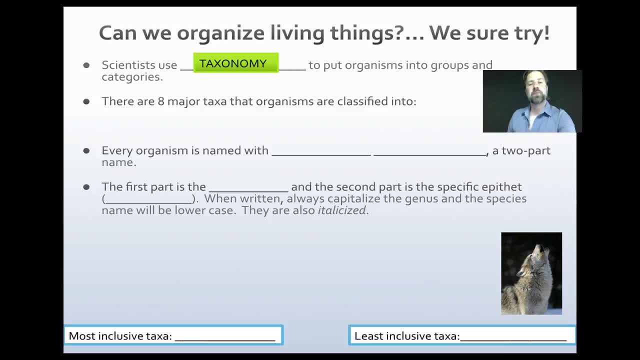 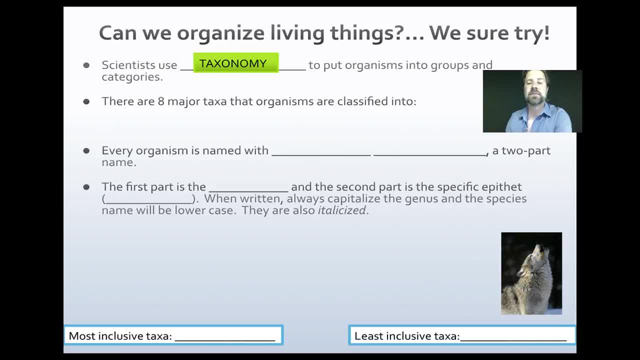 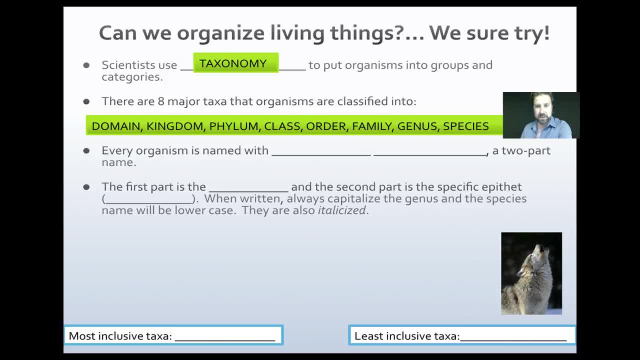 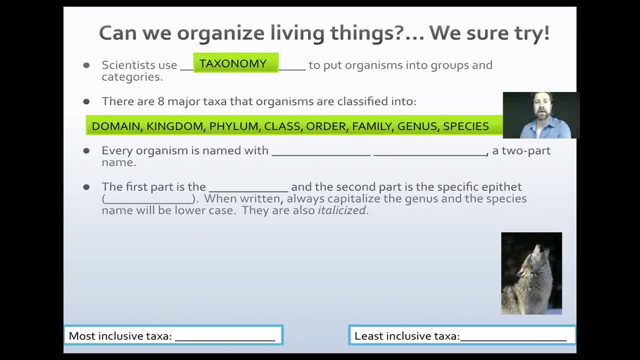 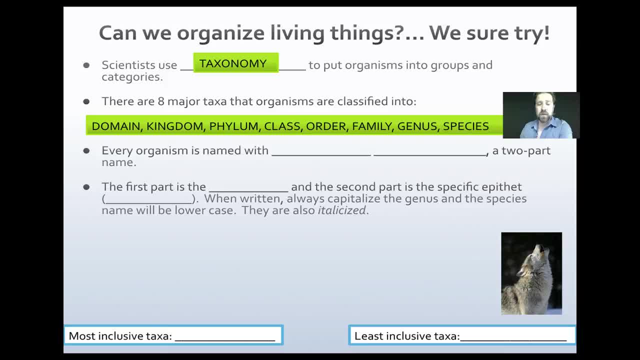 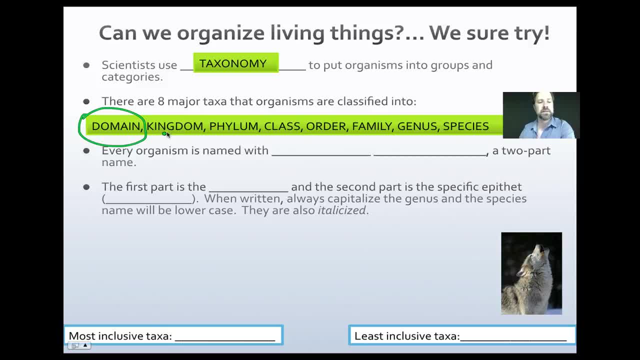 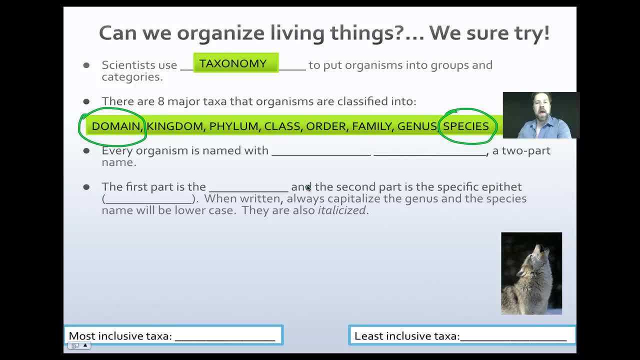 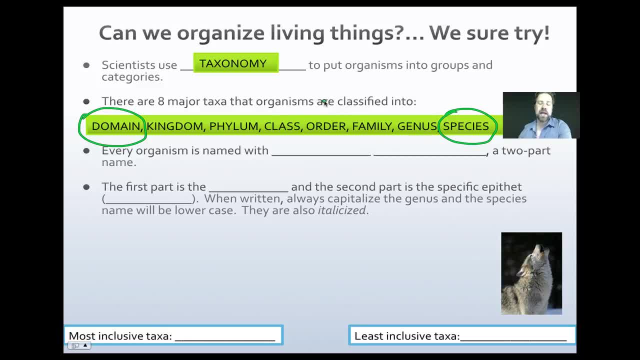 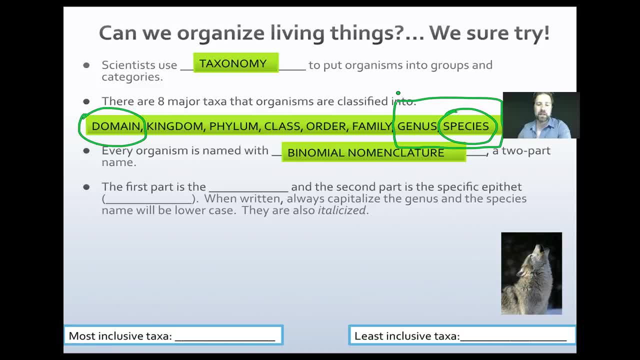 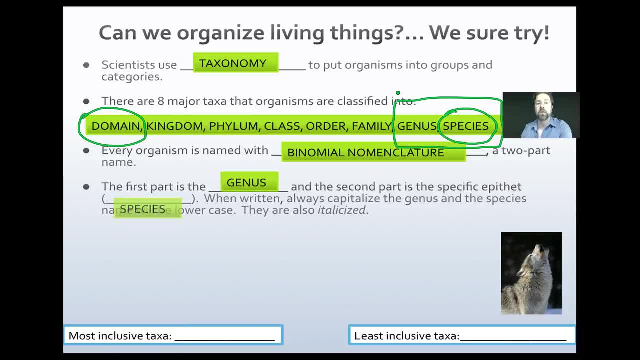 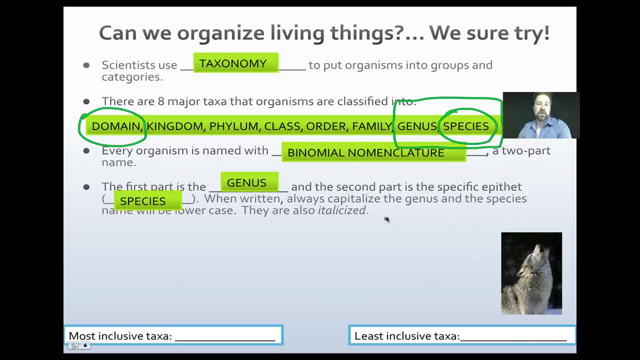 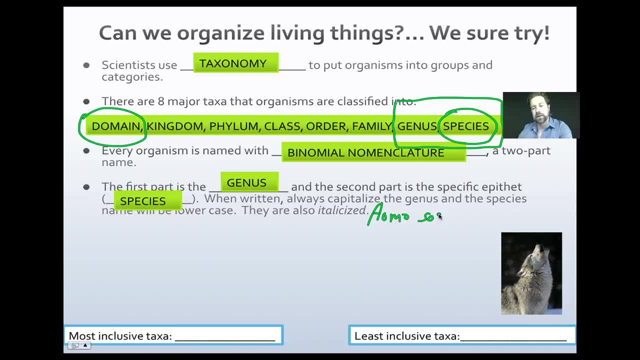 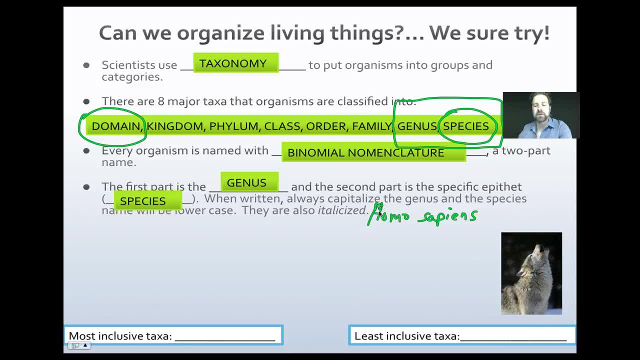 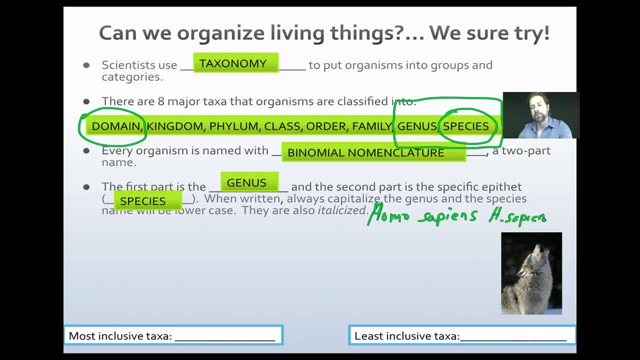 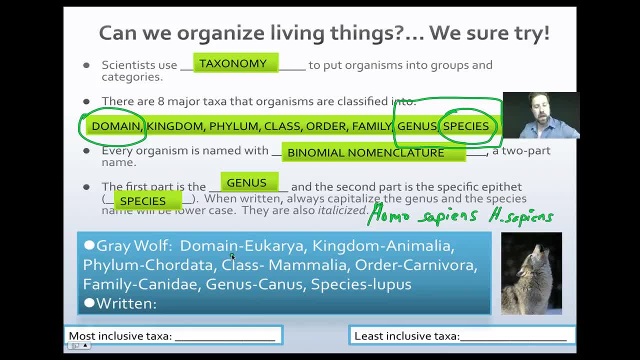 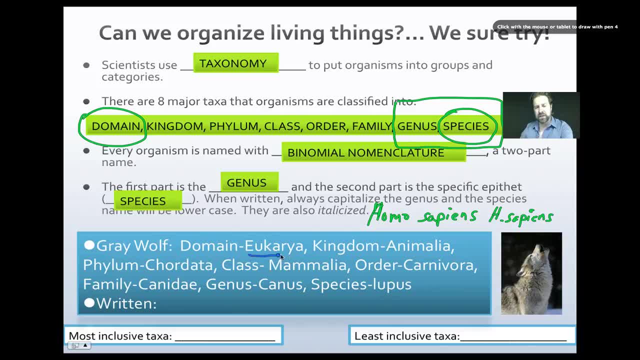 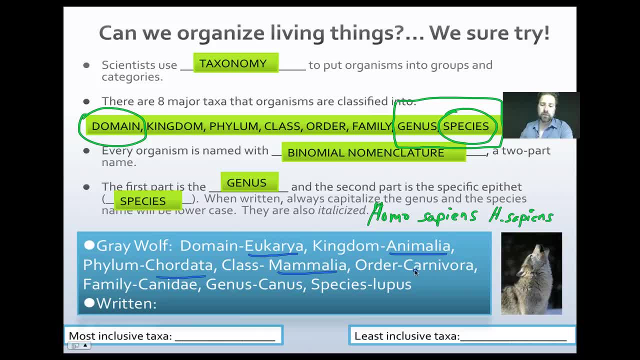 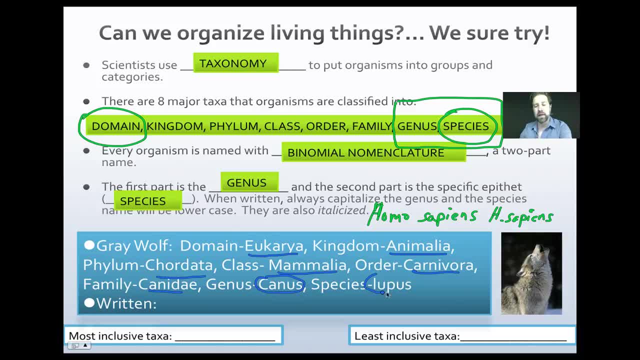 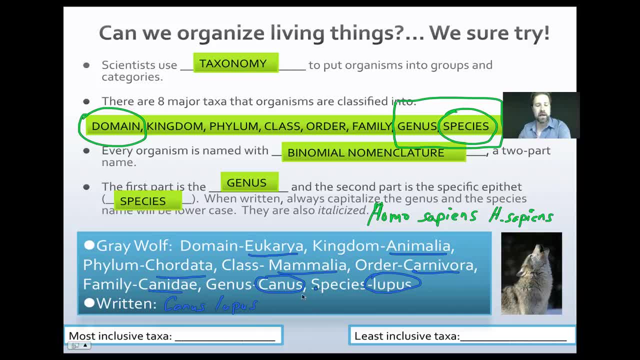 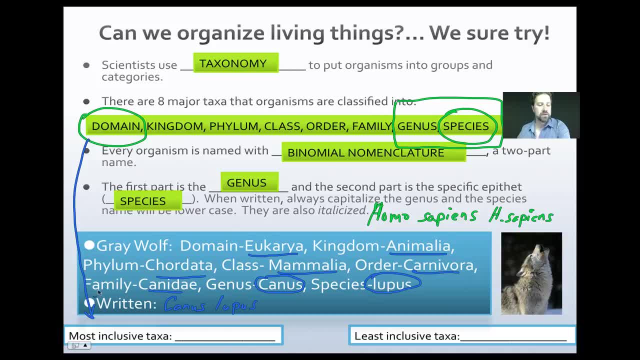 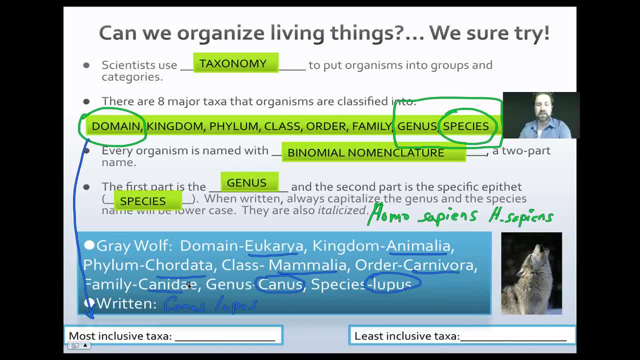 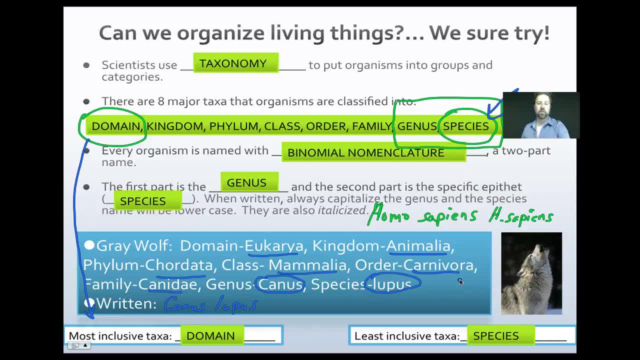 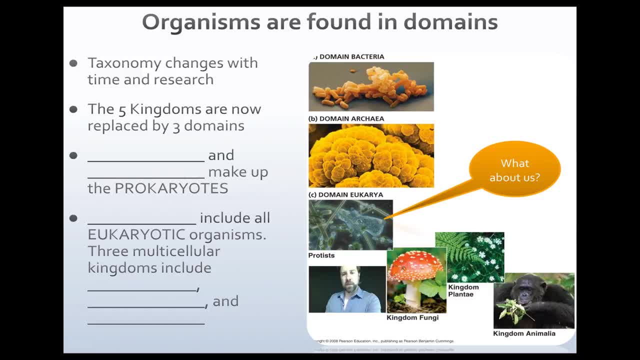 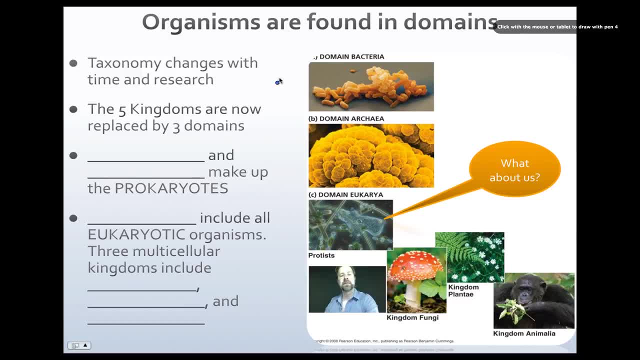 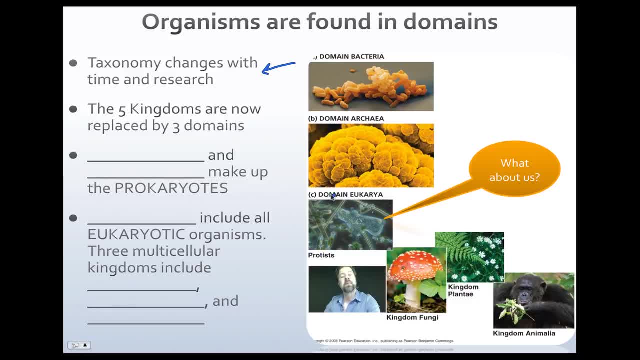 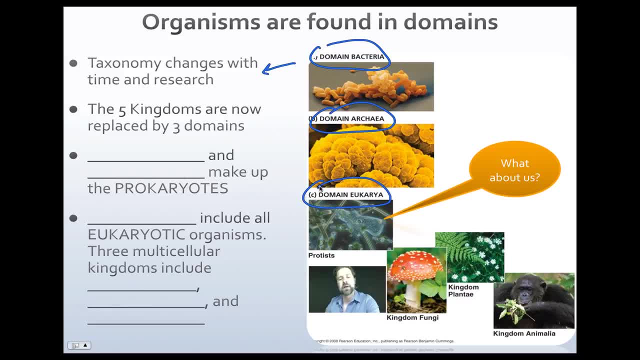 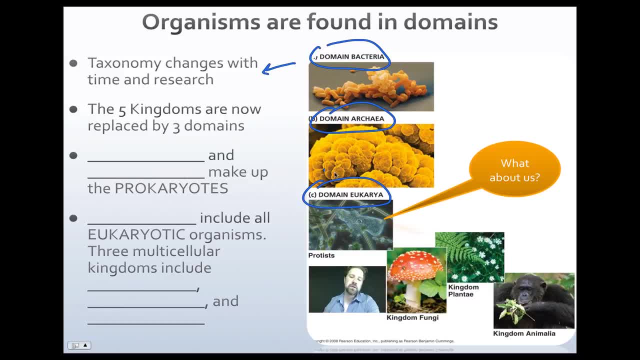 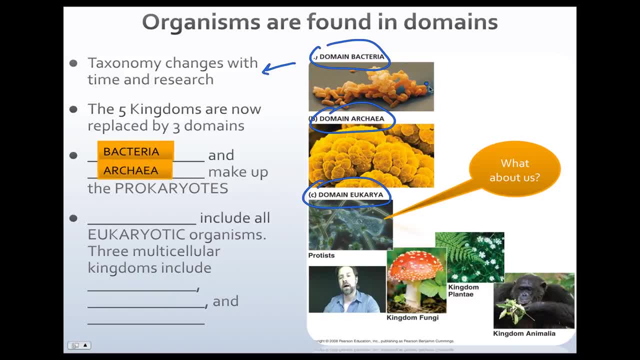 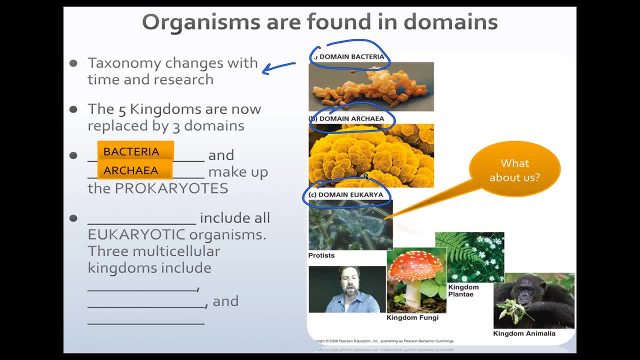 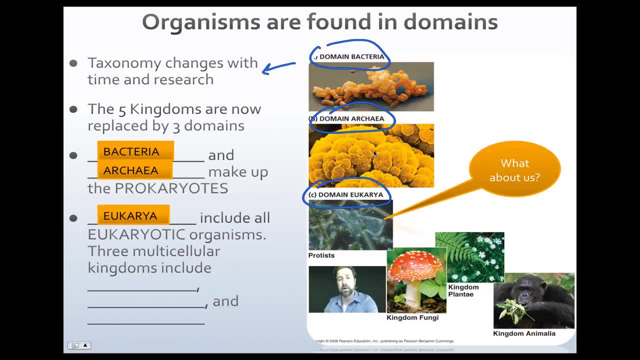 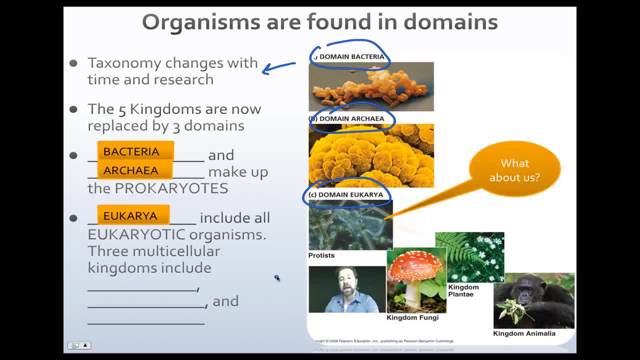 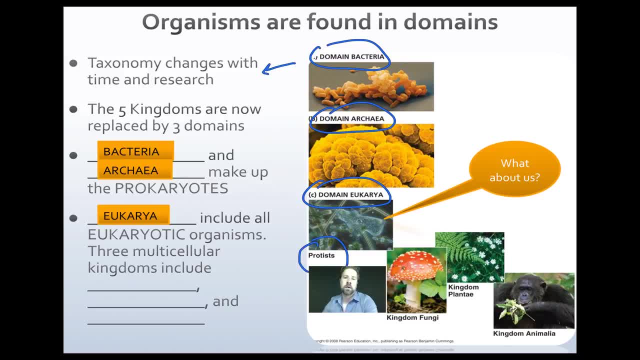 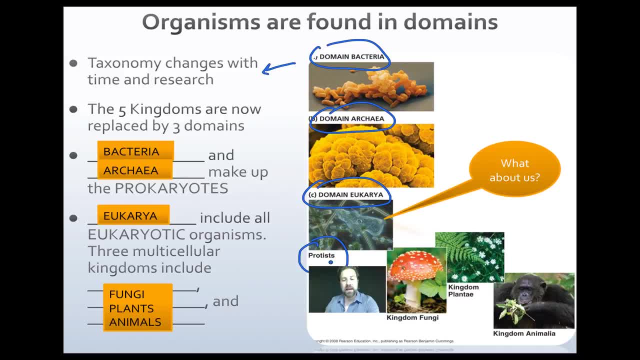 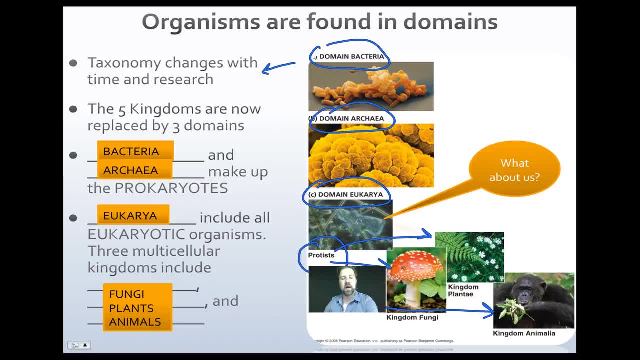 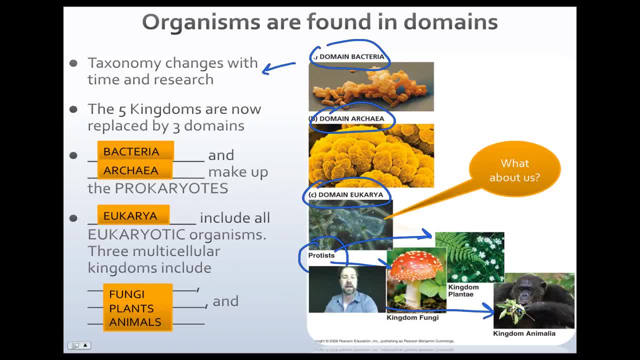 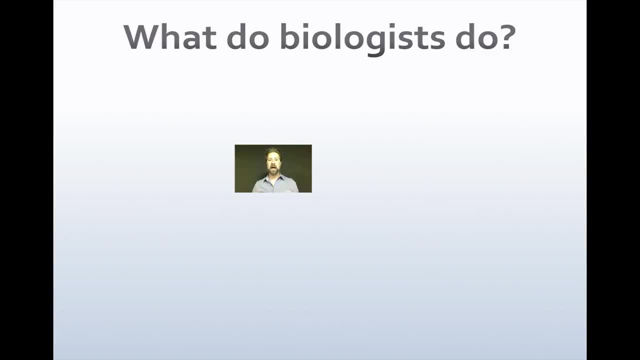 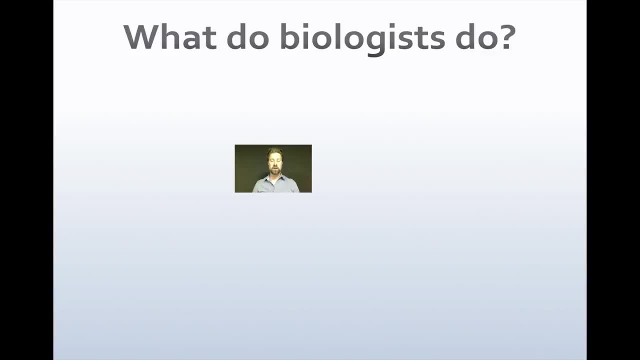 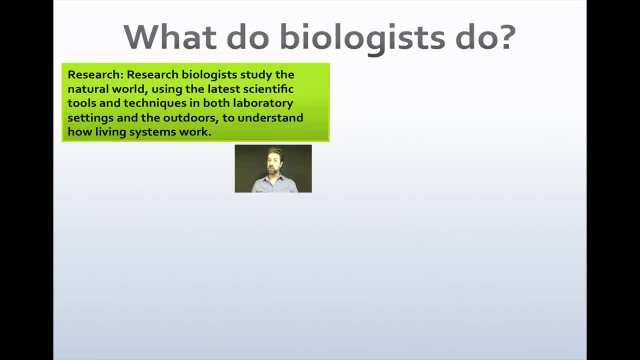 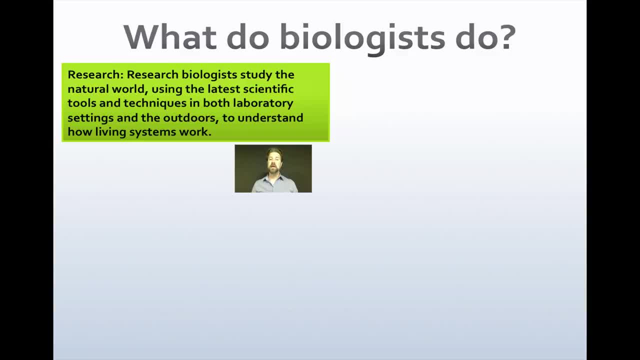 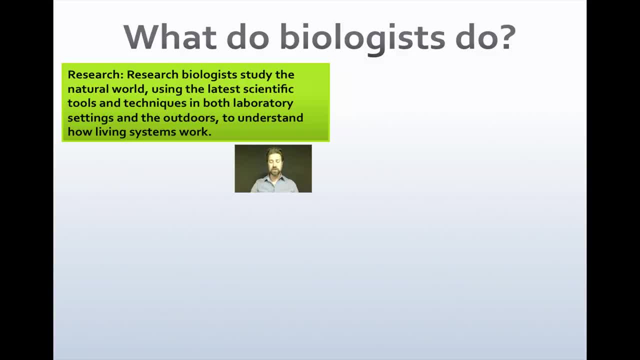 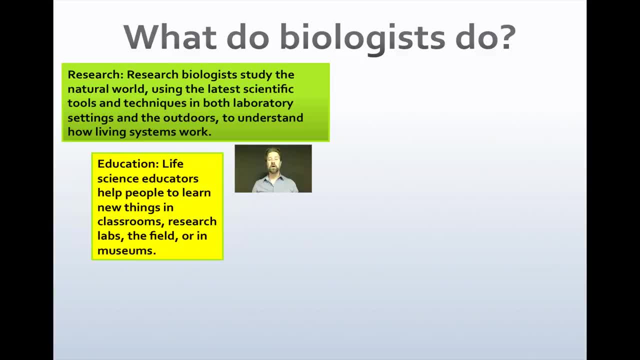 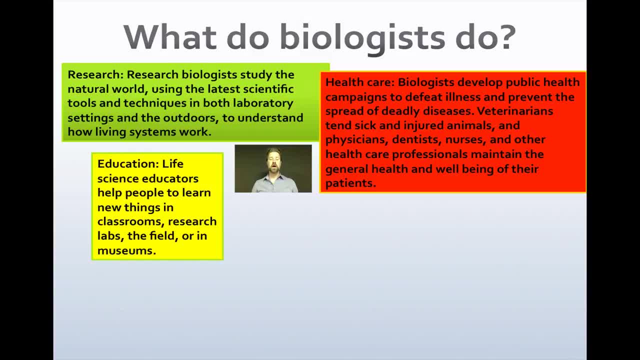 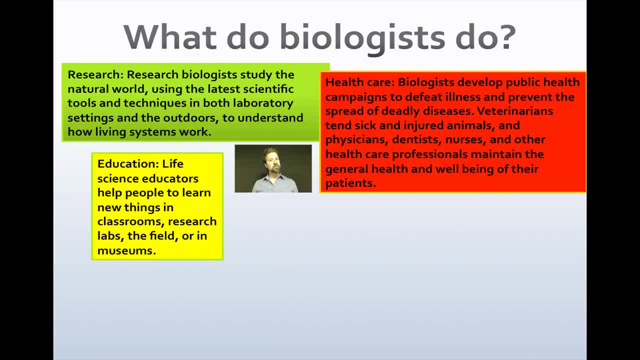 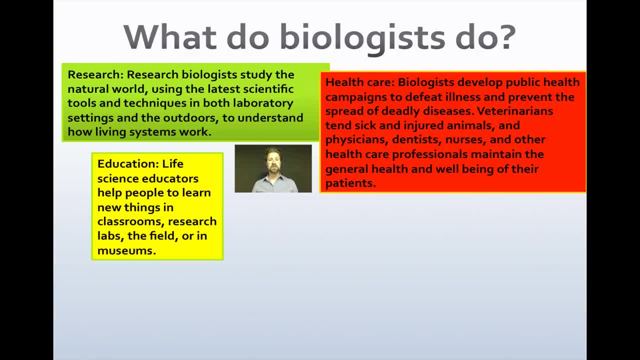 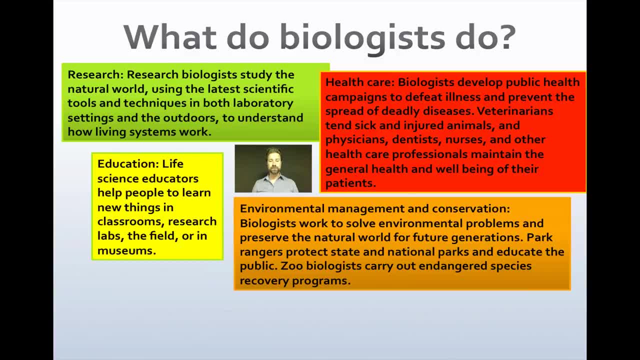 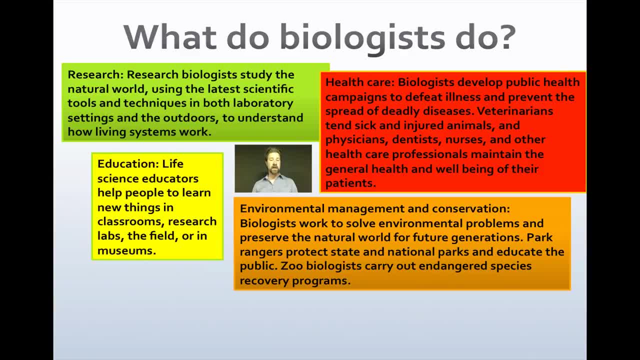 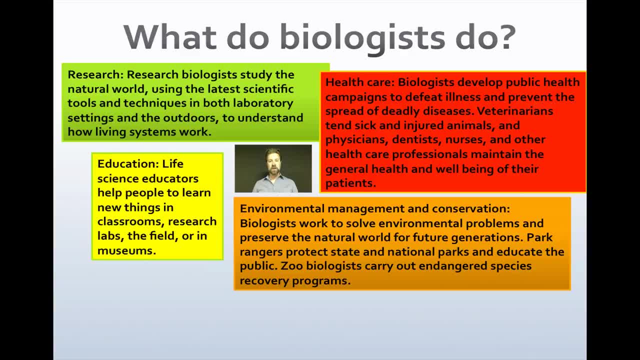 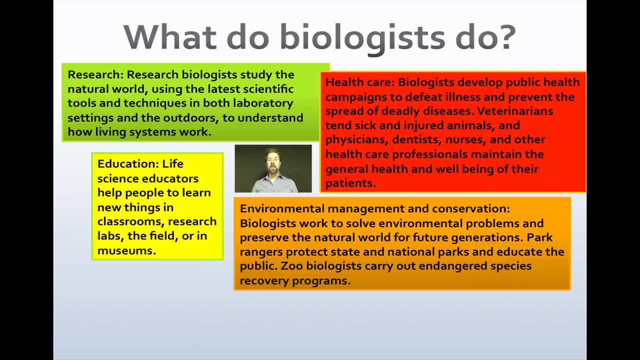 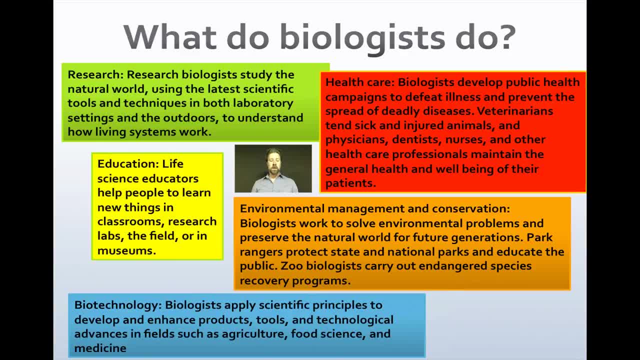 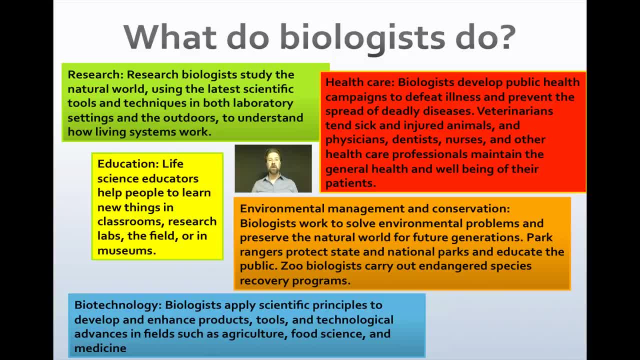 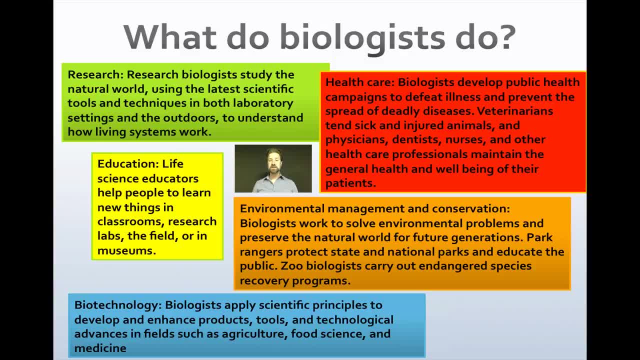 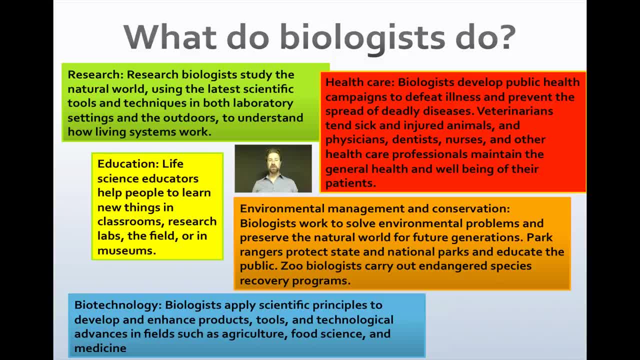 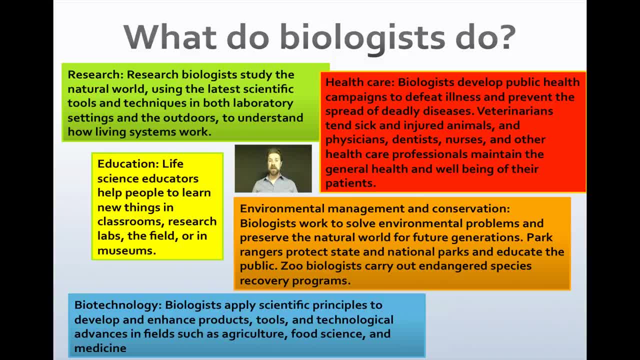 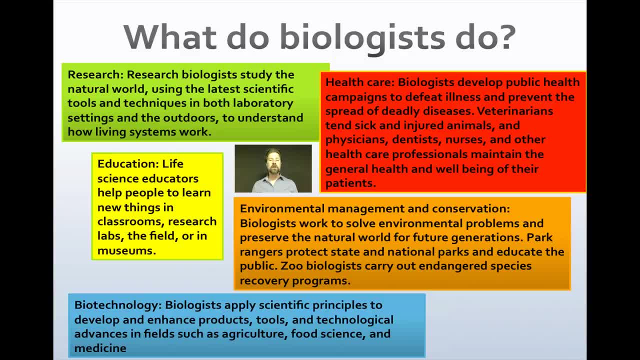 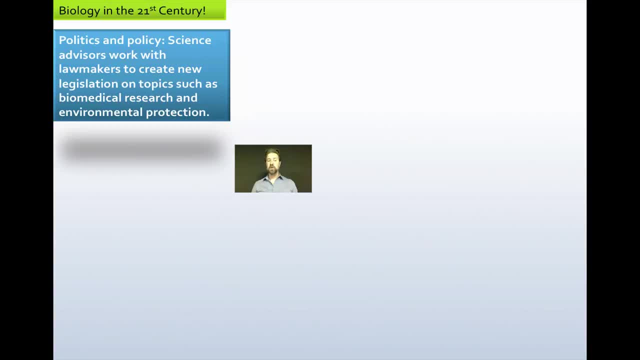 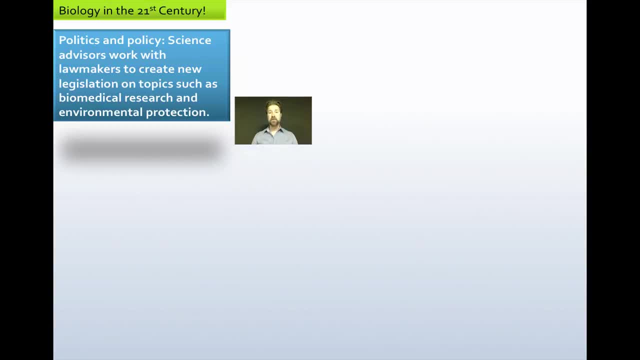 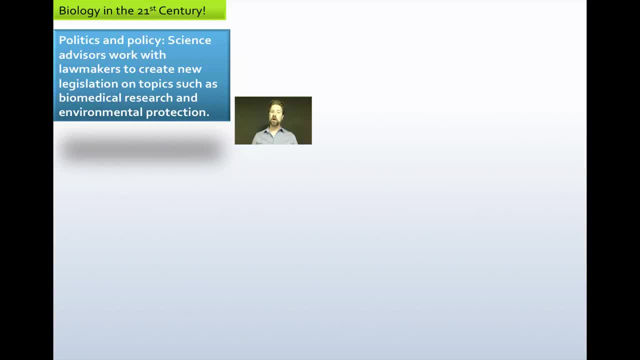 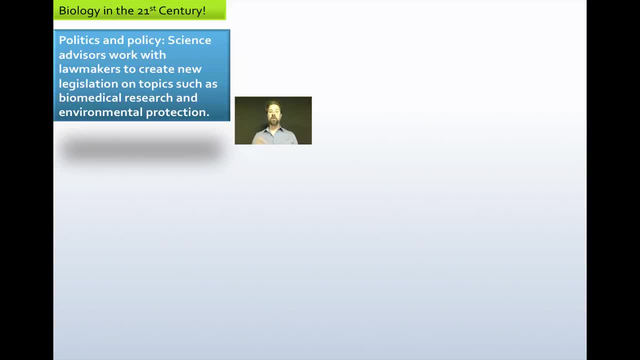 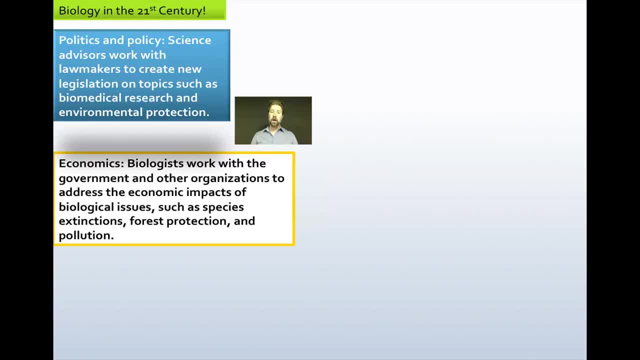 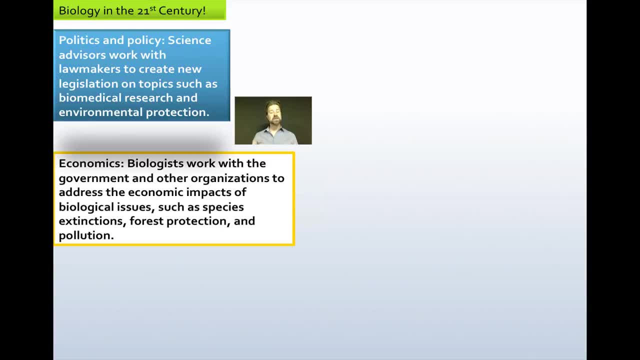 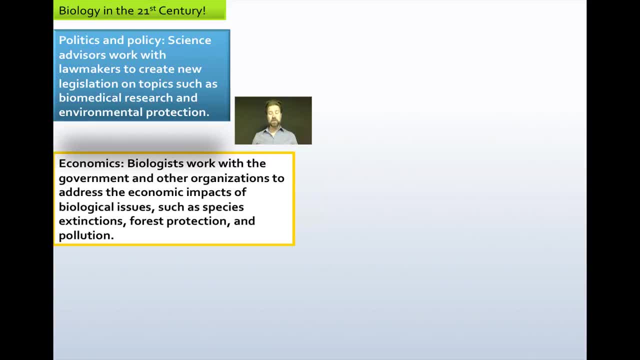 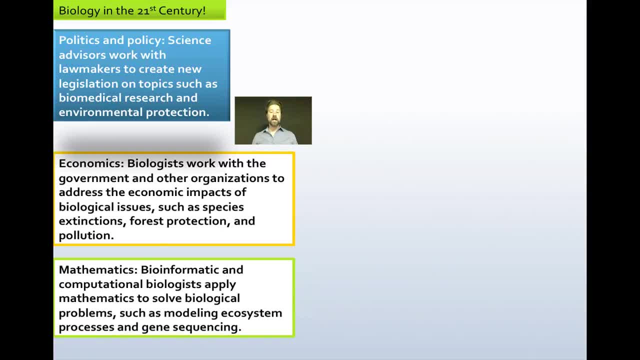 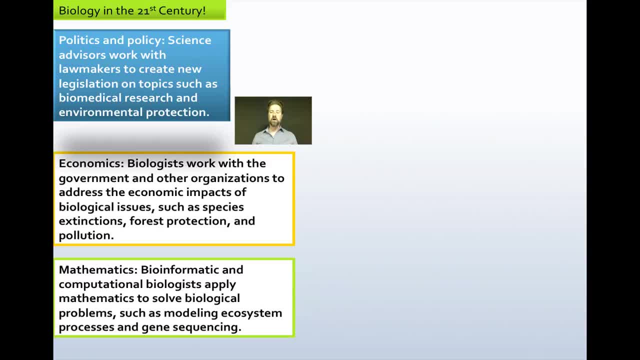 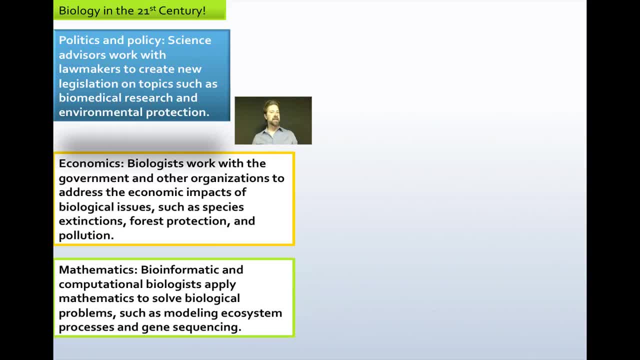 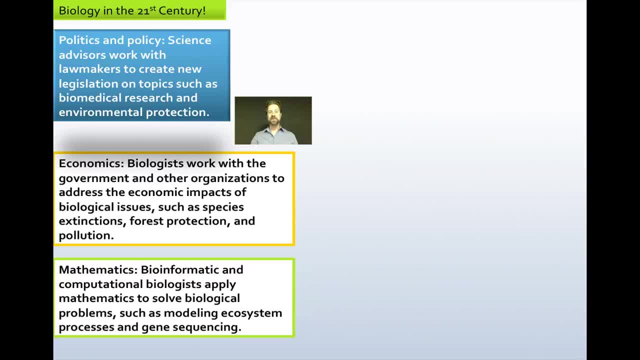 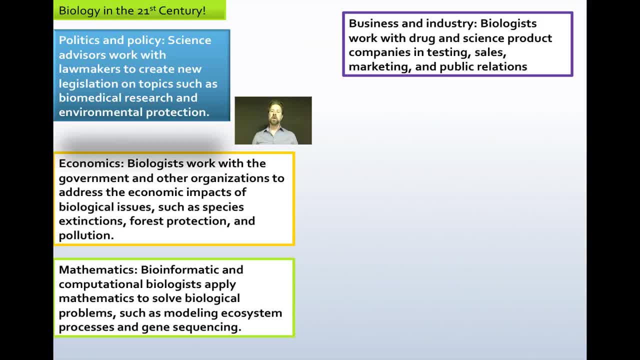 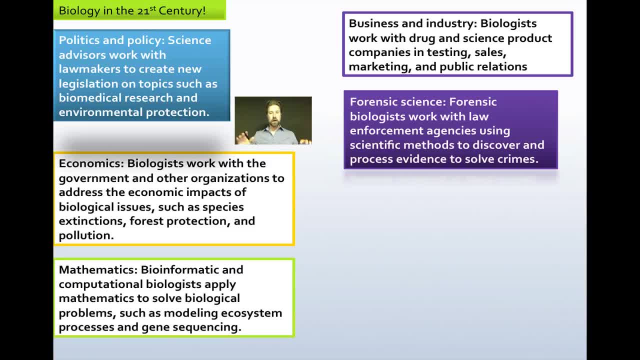 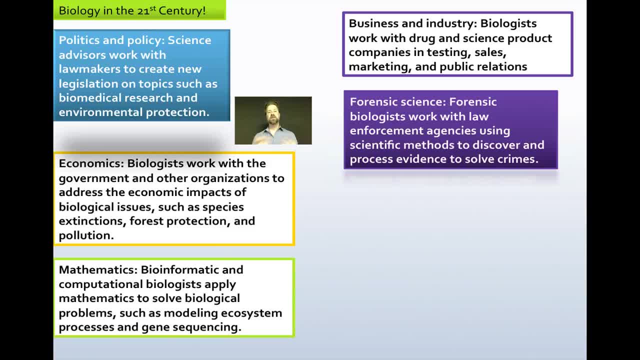 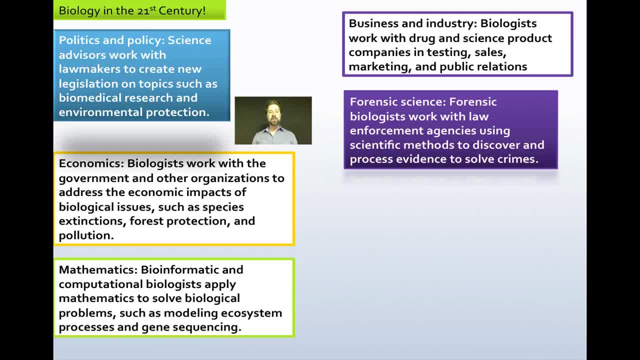 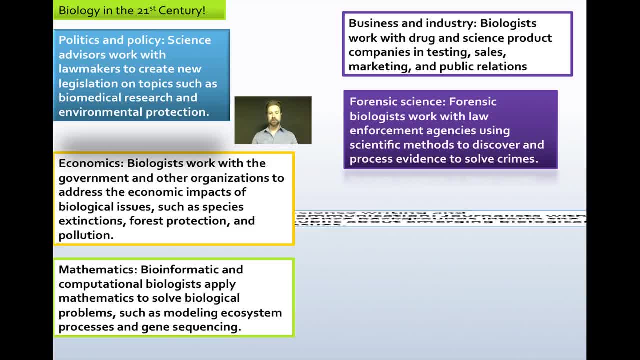 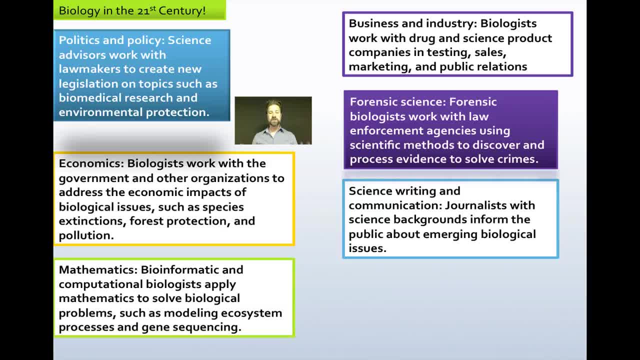 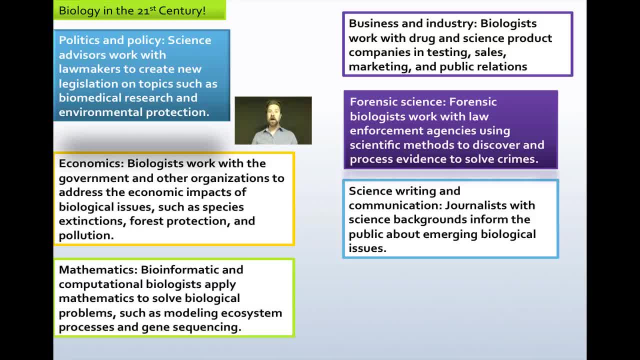 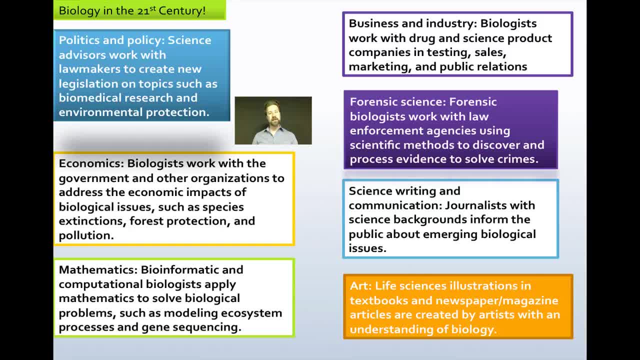 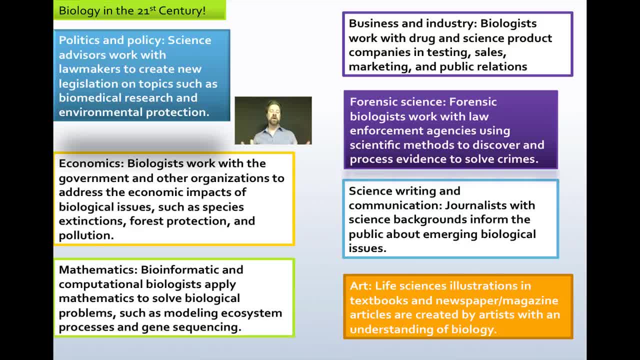 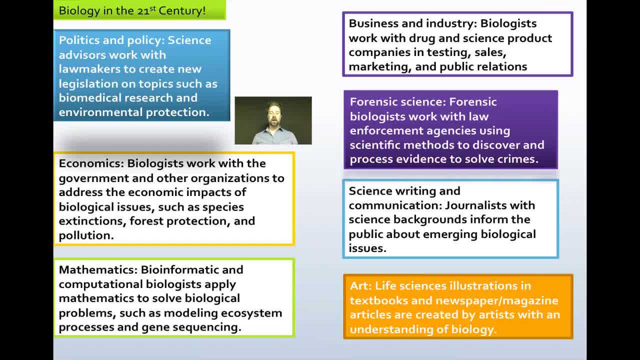 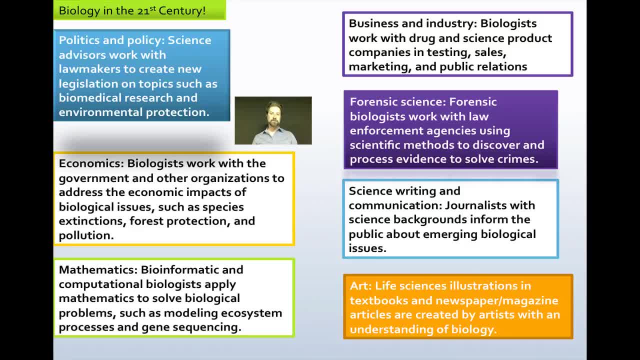 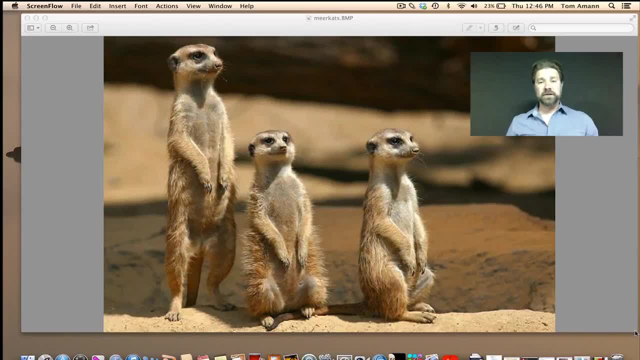 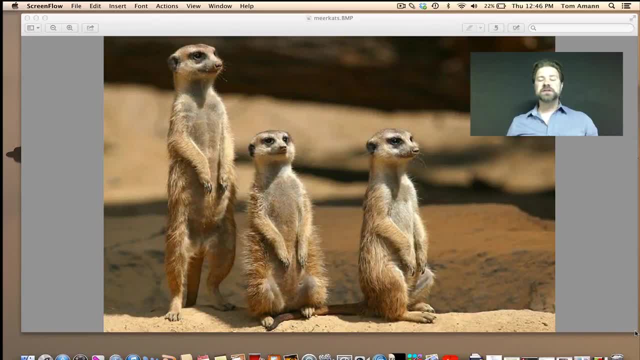 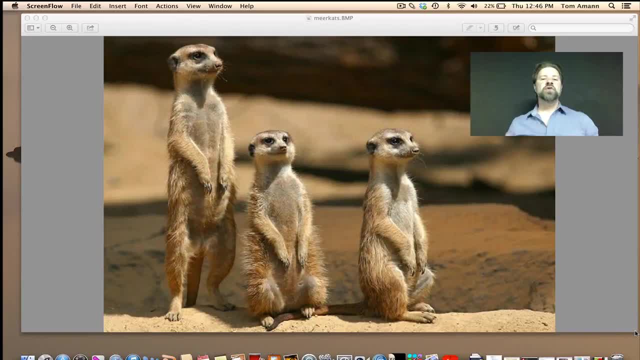 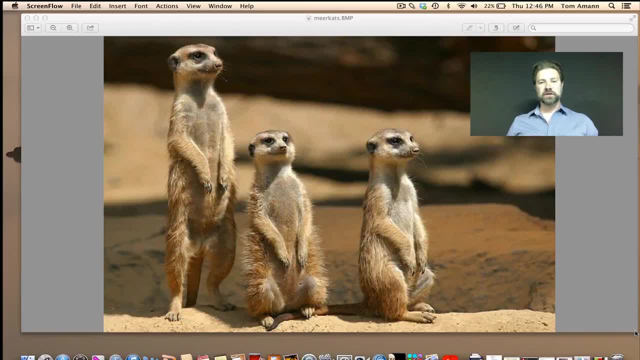 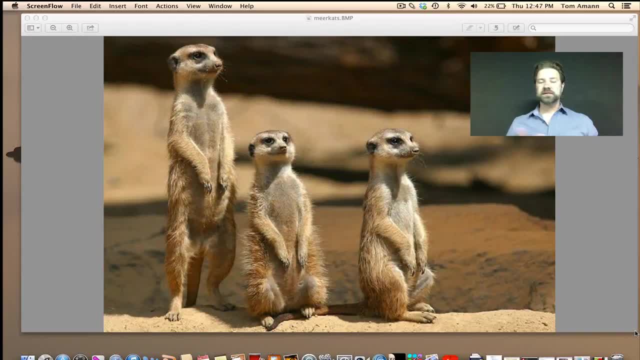 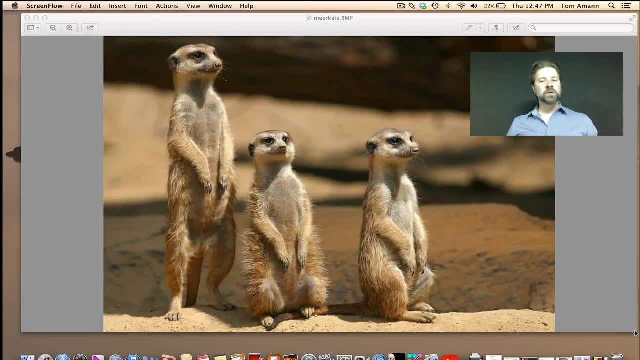 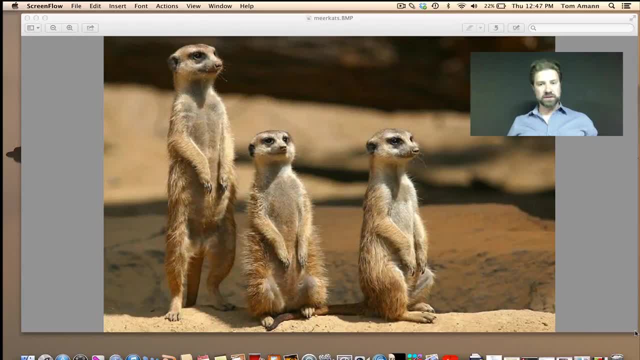 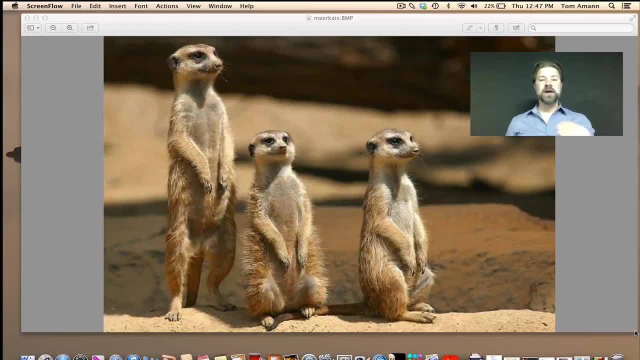 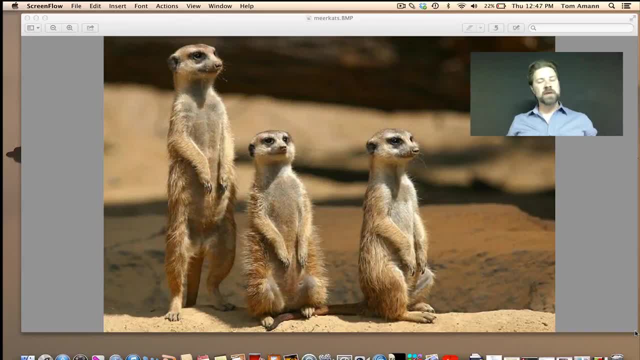 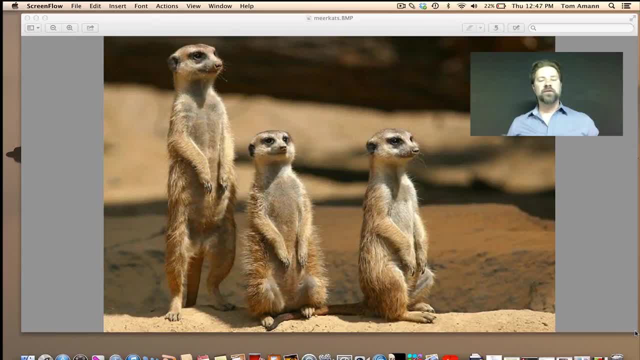 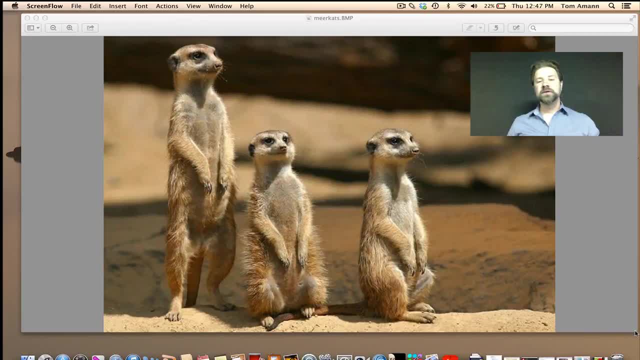 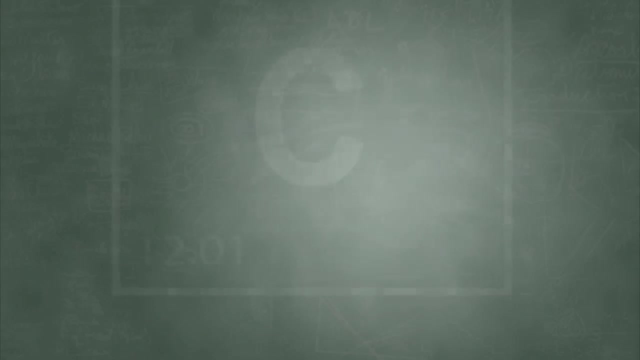